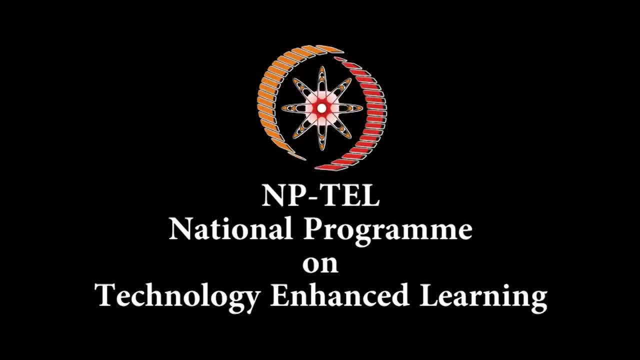 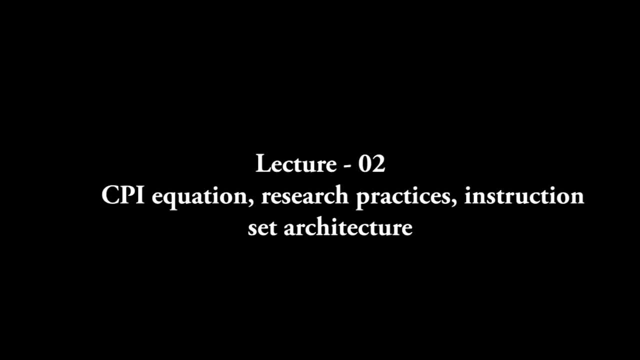 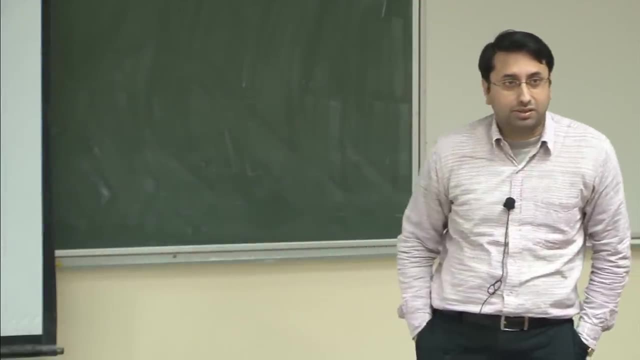 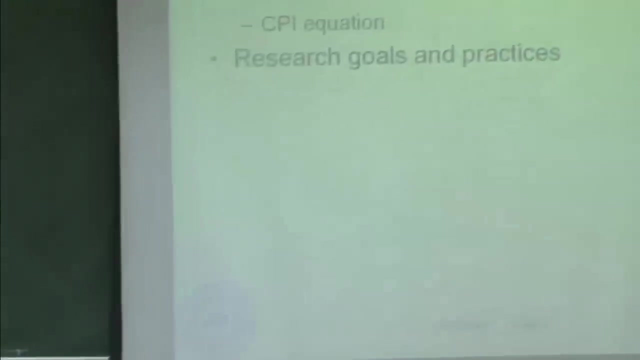 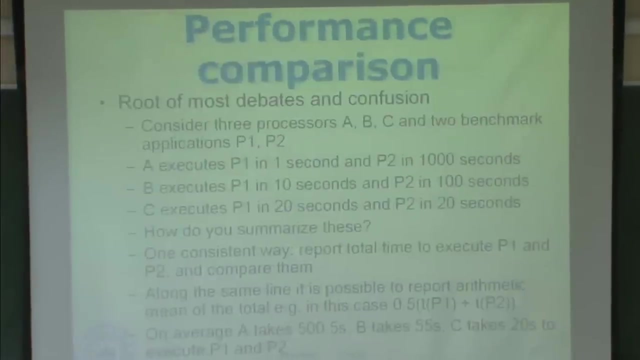 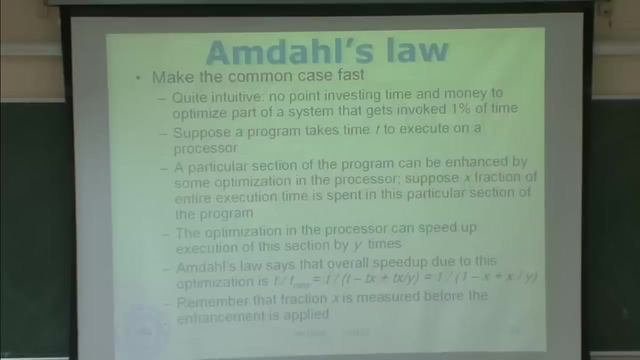 Yeah, we will talk about MIPS instructions. that actually has fused compare jump instruction. Okay, so quickly to recap what we are discussing. We talked about performance measurement metrics, benchmark applications and a little bit on performance comparison. We talked about arithmetic mean, geometric mean and harmonic mean. We talked about Amdahl's law and CPI equation. 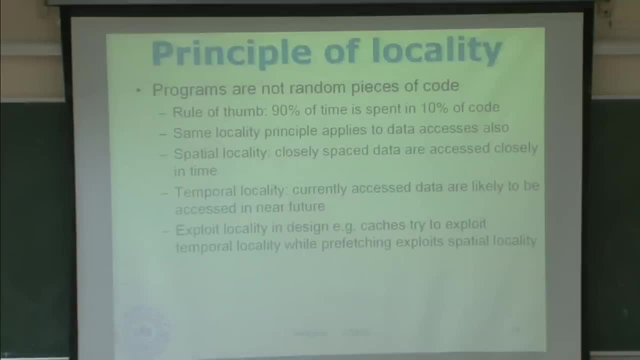 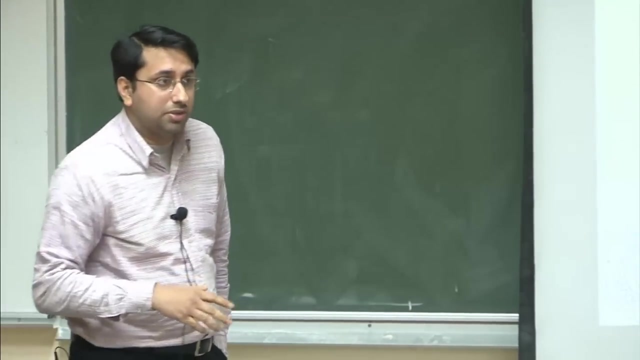 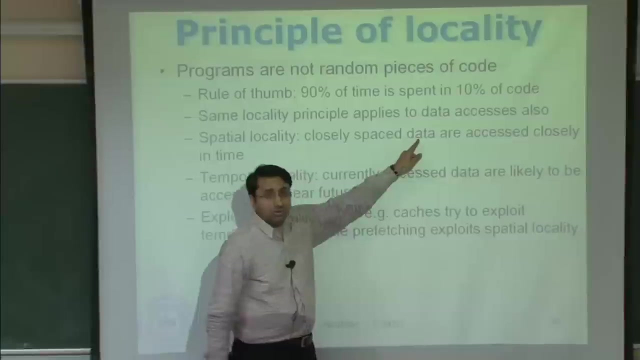 Looked at a few numerical examples as well, And we finished here talking about principle of locality last time. Okay, so this is one of the things that we will visit over and over in the context of, not just caches but in many others- The principle of locality. So here, do not think that this data always refers to your 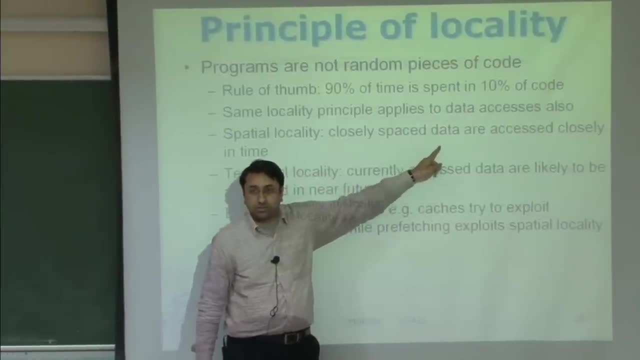 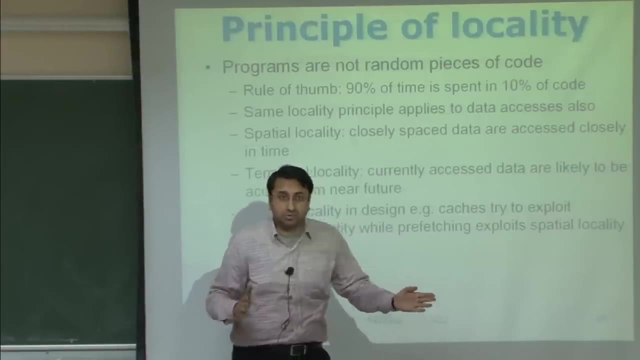 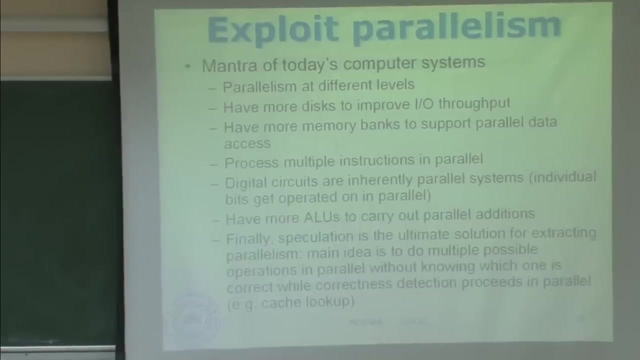 memory data. It can be any data, for that matter. So, for example, if you are looking at a sequence of data values, any data values locality principles may still apply there. So we will look at such things also. 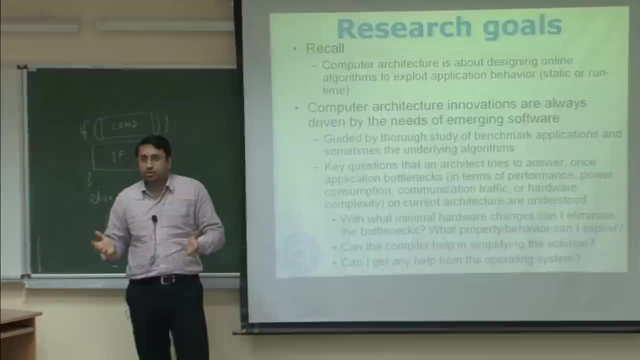 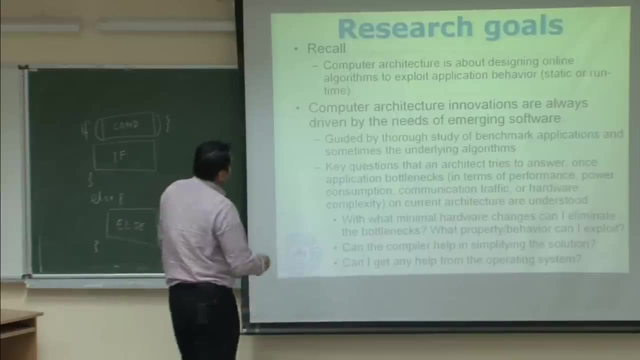 So this is a very simple example of a simple algorithm. So you can see that some new software comes up with some new problem, and that is what the architects study and they propose solutions so that the software can be spread out. Okay, So, guided by thorough study of 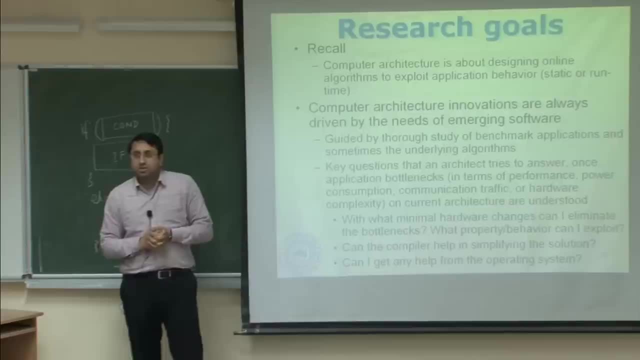 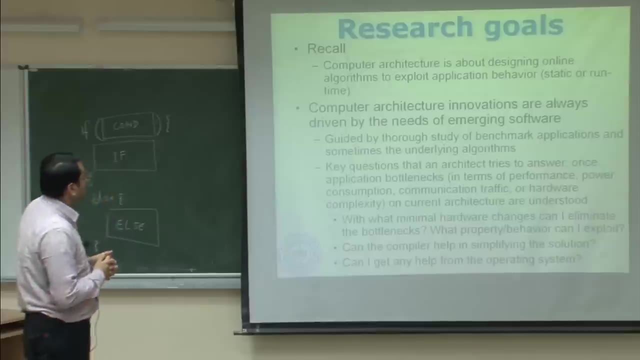 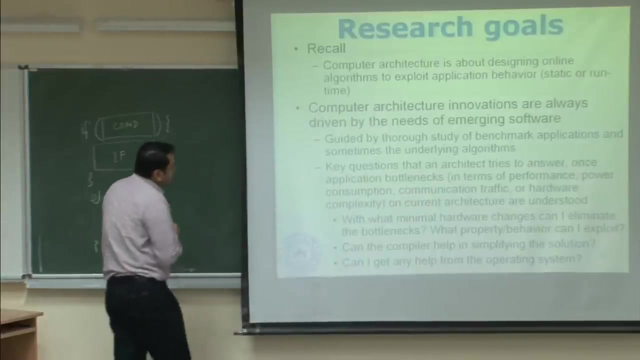 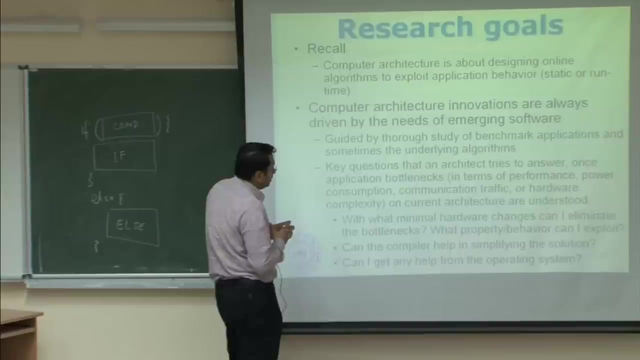 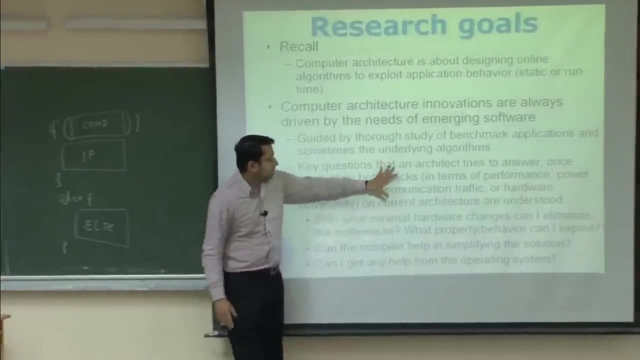 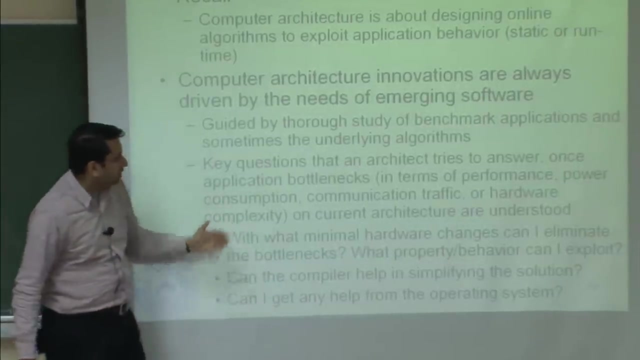 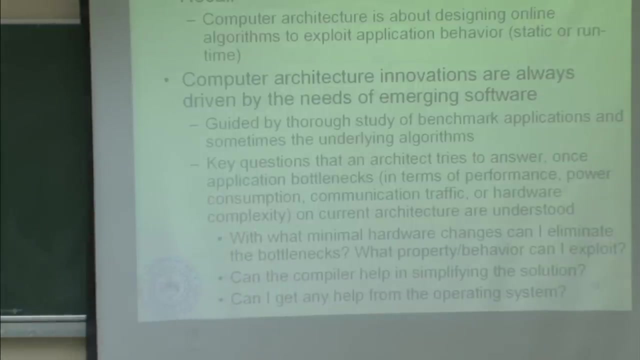 benchmark applications and sometimes the underlying algorithms. So computer architects spend a lot of time understanding applications, their behavior, profiling applications and understanding what they do by understanding the underlying algorithms of the applications. Okay, So the basic question is: can I eliminate the bottlenecks? So that is the basic question. All right, And this minimal part is very important. You have to be thrifty when you propose something. You cannot just propose something gigantic for solving something. Okay, That will not be acceptable. And, of course, what property and behavior can I exploit? Because we talked 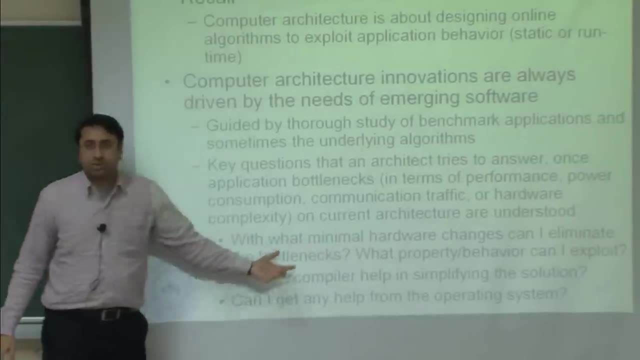 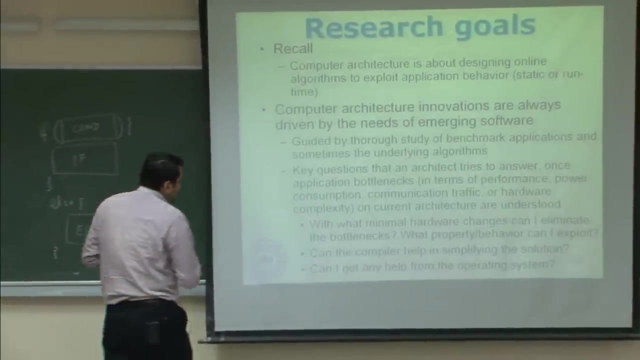 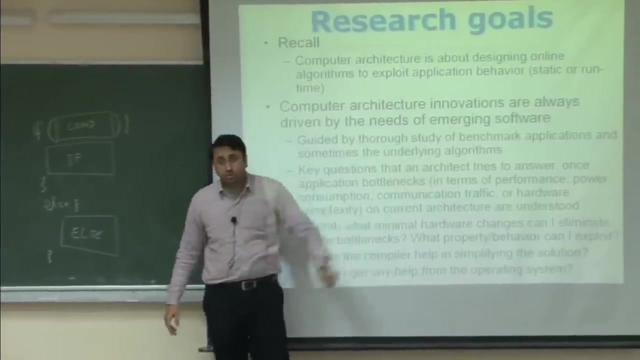 about this thing Right, That your solution usually exploits certain application behavior. So what is that property and behavior that I can exploit to solve this bottleneck? Okay, 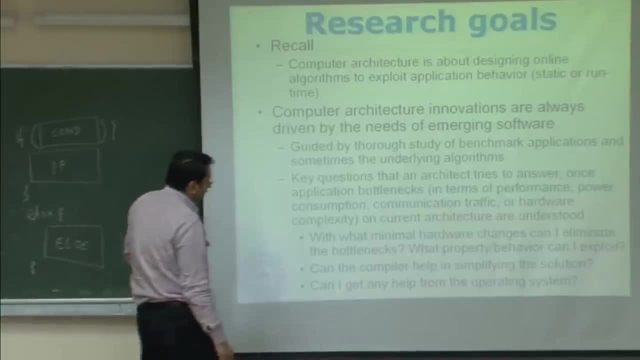 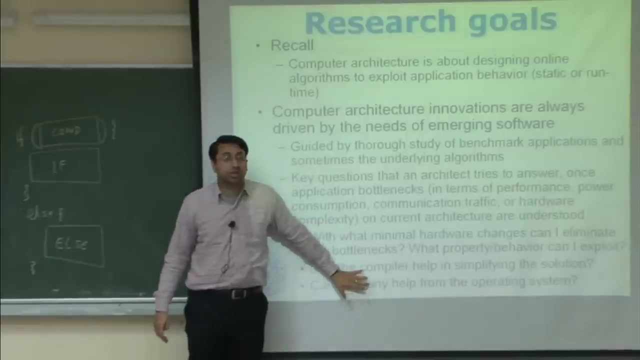 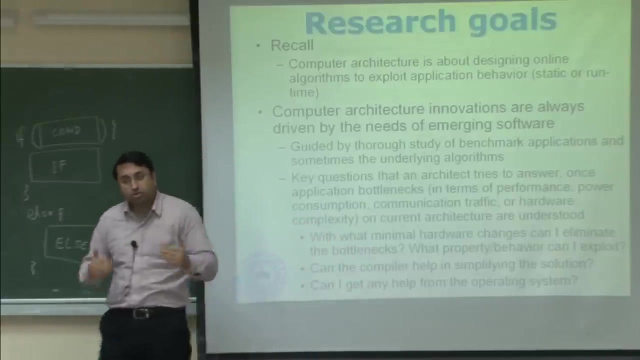 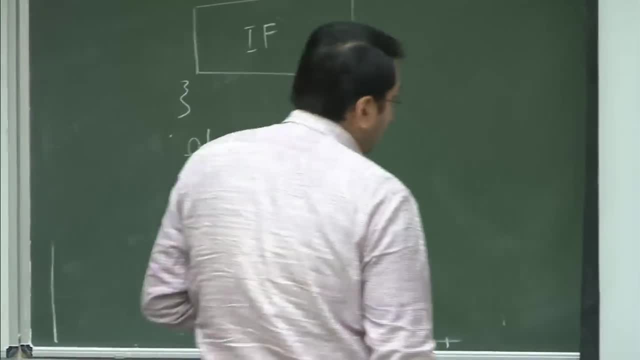 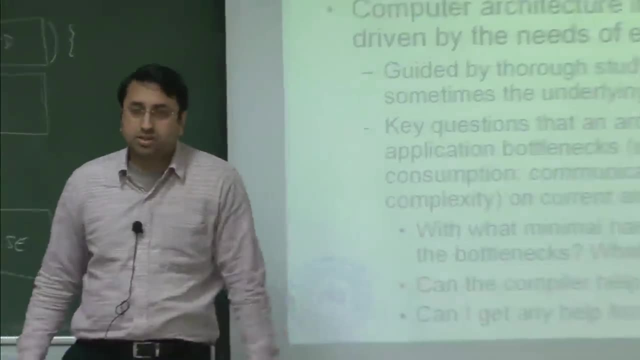 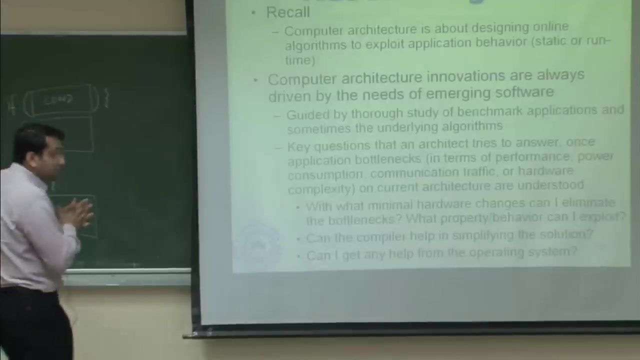 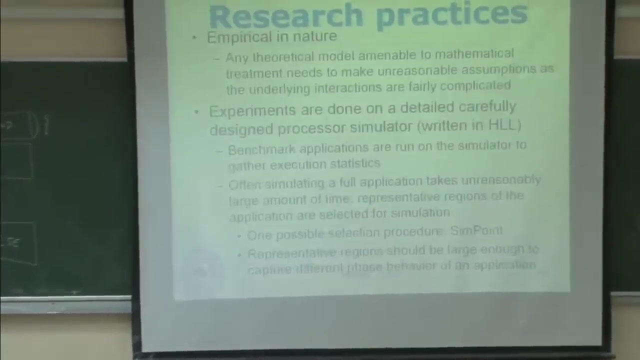 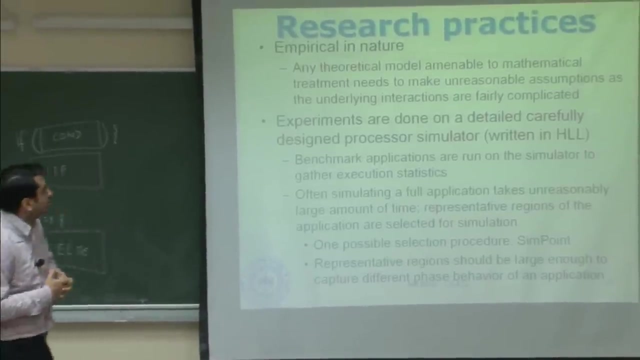 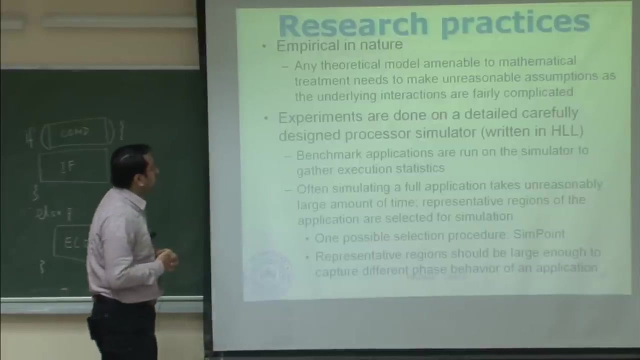 Any question. So how do you carry this out? So the research in this area is empirical in nature. The reason is that any theoretical model amenable to mathematical treatment needs to make unreasonable. 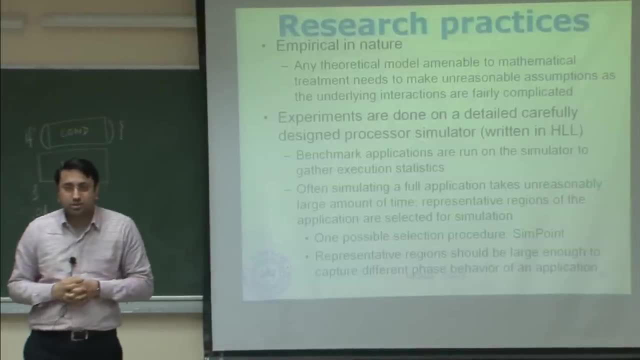 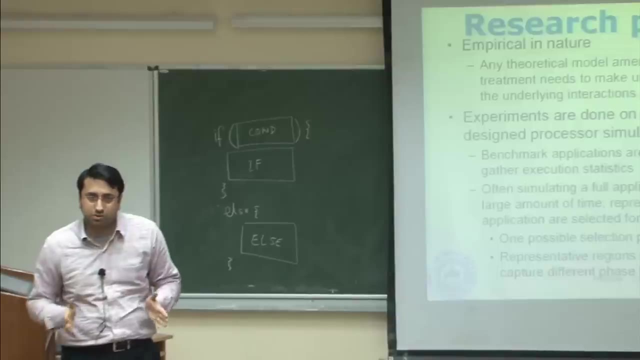 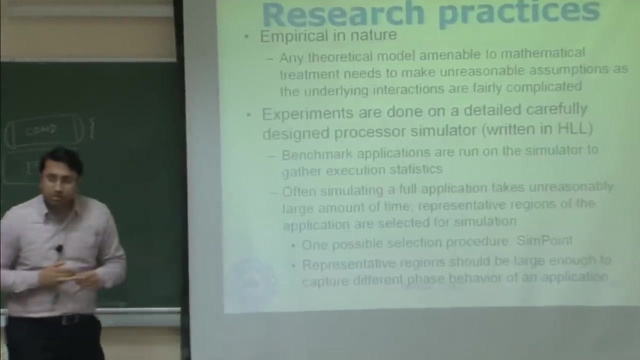 assumptions, as the underlying interactions are fairly complicated. So coming up with an analytical model for an architecture is extremely difficult without making certain unreasonable assumptions, Which is why what you do is experiments are done on a detailed, carefully designed processor simulator, usually written in high level language. 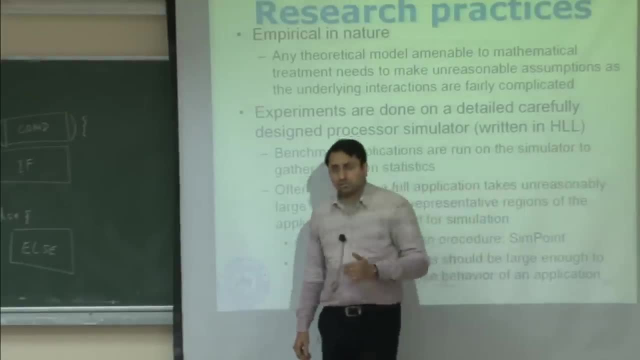 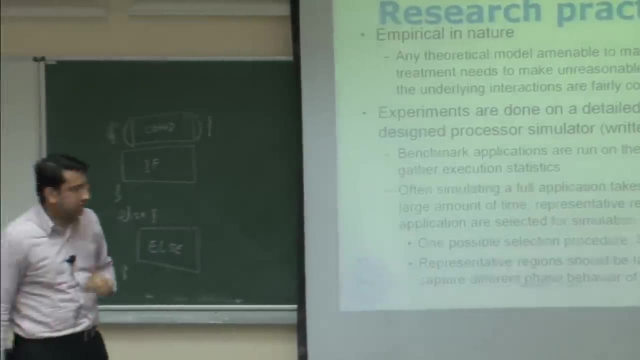 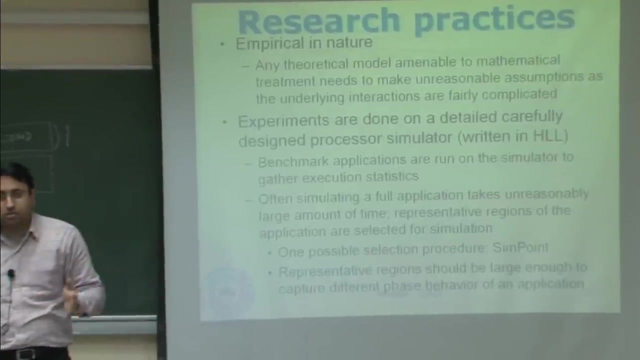 Although you can go to a little lower than high level language like Verilog. that is slightly lower than your C, C++. that is called an RTL language register transfer language. So what you do is you, the simulators, try to model the processor that you try to design. 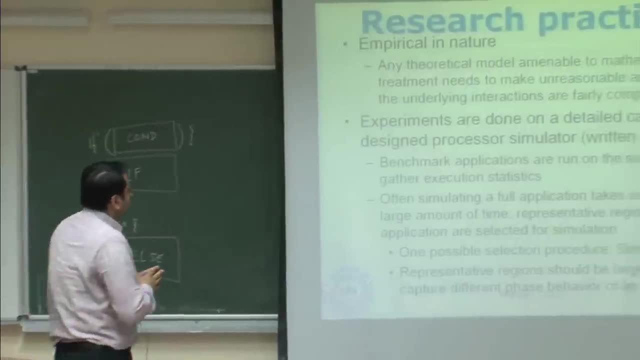 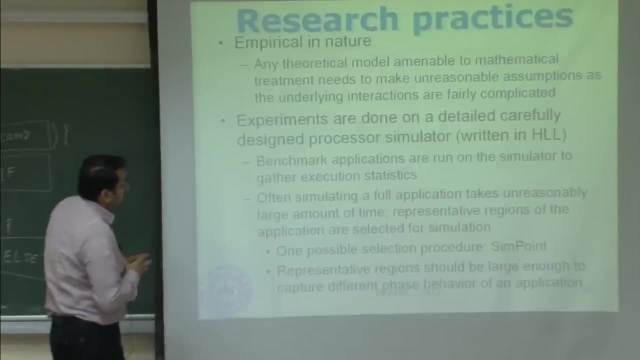 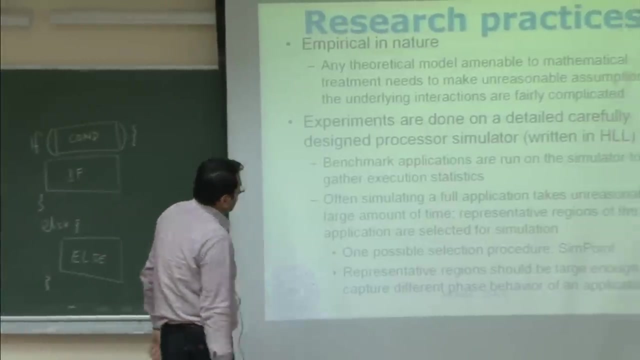 as accurately as possible. So it is a piece of software. this simulator is actually a piece of software that models your hardware processor and your benchmark applications are run on the simulator to gather execution statistics. So you run the benchmark application on the simulator and you pretty much can get to know. 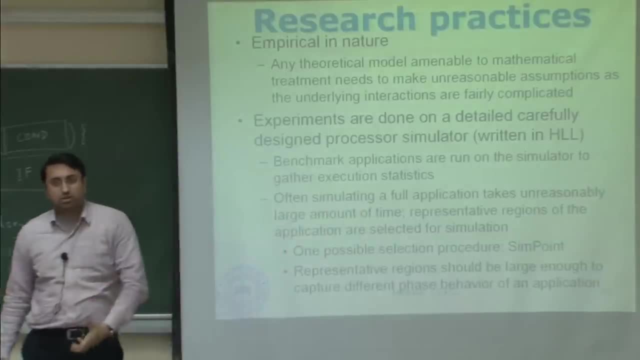 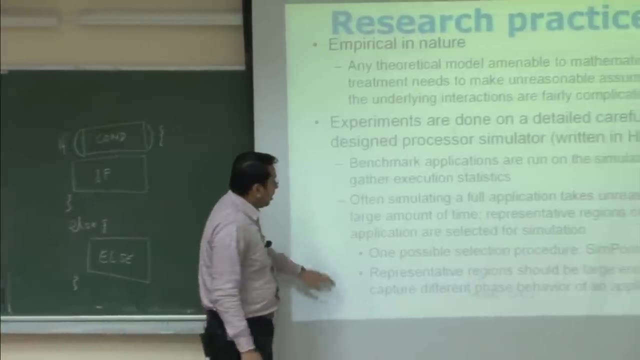 whatever you want to do, Because it is a piece of software, It is run by you, It is under your control. You tell it to tell you something you know. it will tell you that. all right, Often simulating a full application takes unreasonably large amount of time. okay. 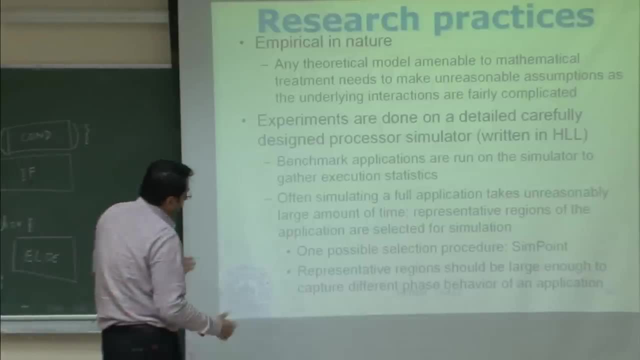 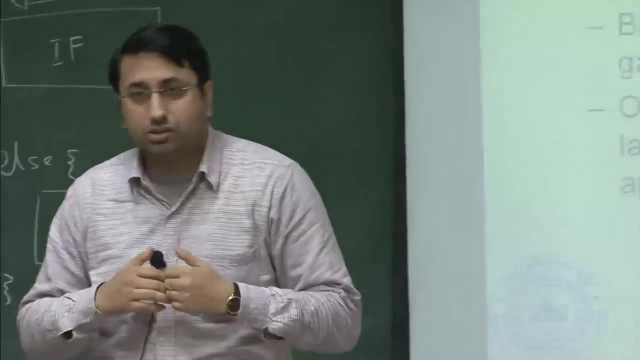 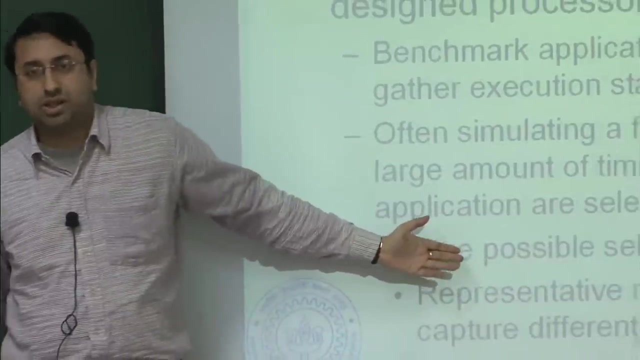 You will probably not believe, but there are. you know well, actually, pretty much almost all benchmark applications that are important will probably take months to run on any good simulator, okay. So if you, if you have to, you know, wait for so much of time, then of course, no innovation. 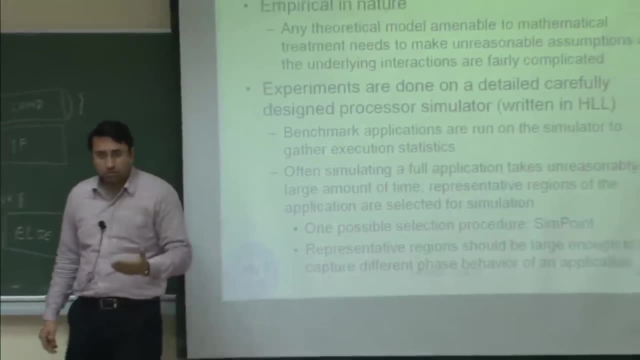 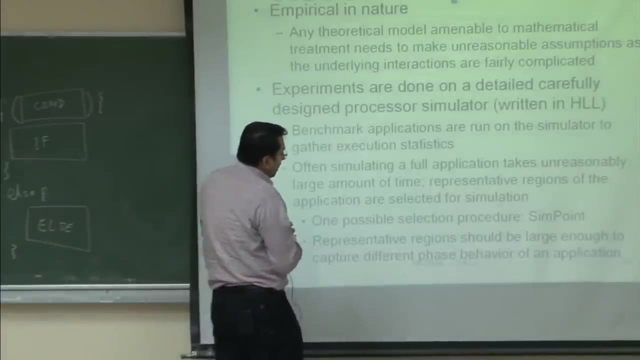 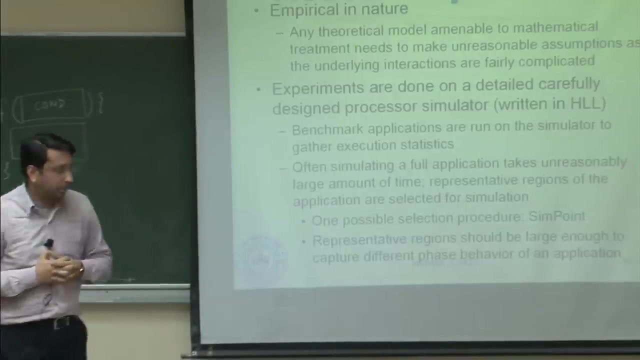 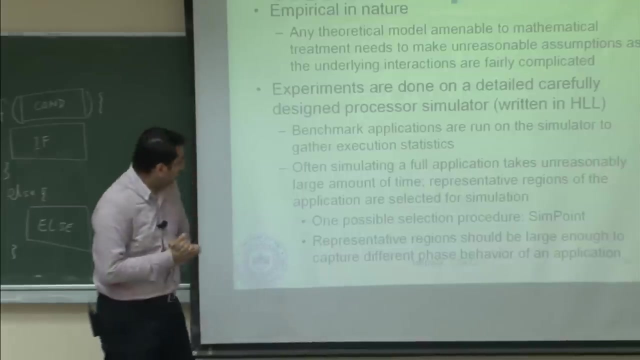 will get done in. So you need some other ways, of course, some scientific ways, of speeding up simulation. So what usually people do is that they find out representative regions of the applications and those are selected for simulation only okay. So any suggestion how to pick representative regions of an application? 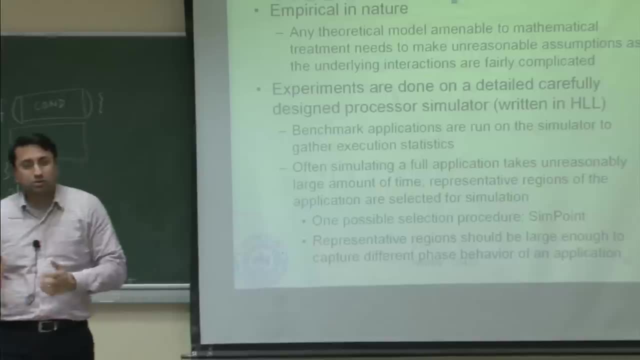 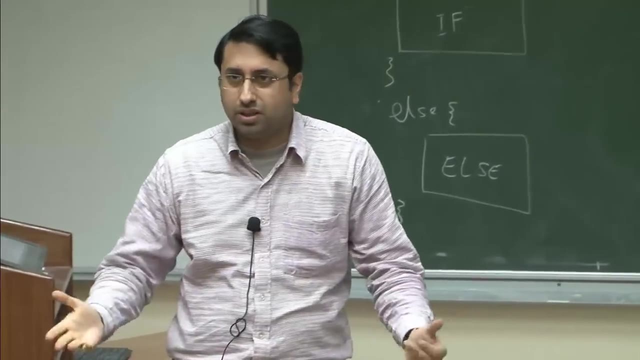 So it talks about something. it says sim point. you do not have to know about that. I will tell you Any suggestion. if you think of something. I give you an application, some program, right, and I ask you tell me the representative regions of this program. How do you do that? 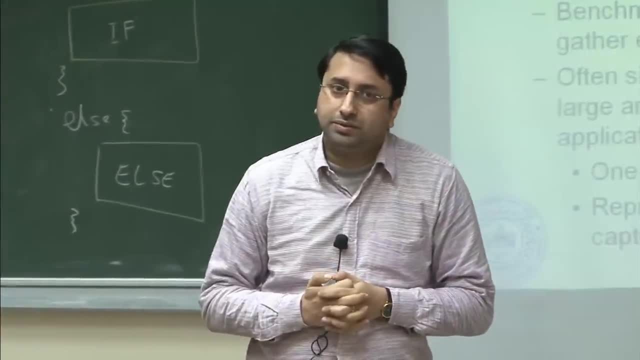 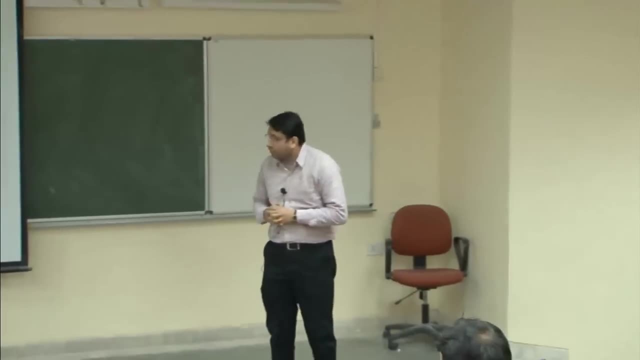 Try to look at the 10 percent of code, like: How do you, sorry, try to look at The 10 percent? you mentioned that 90 percent of the time 10 percent of the code runs. Okay, all right. So try to look at what 10 percent of the code is running for maximum work time. 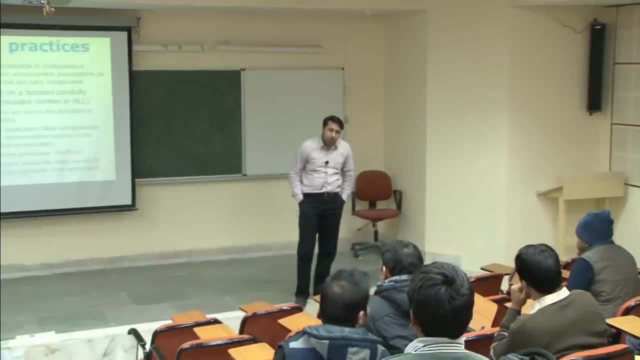 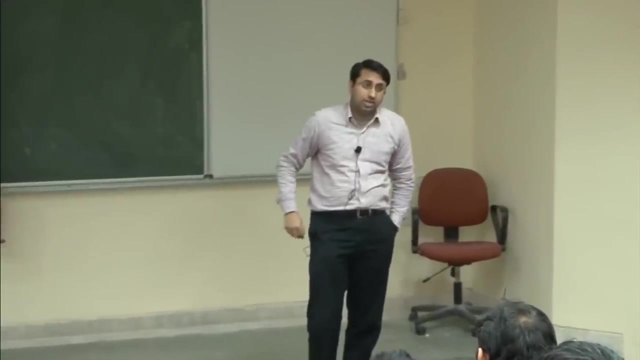 Okay. I mean you run a small application for small data and you try to figure out that region of Okay Application and then that region becomes But that region will take months to run on realistic data. 90 percent of a month is what. 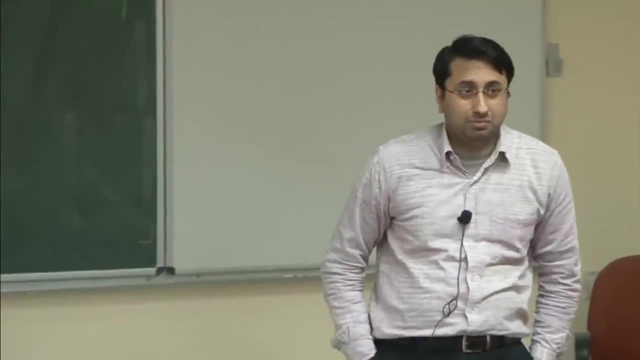 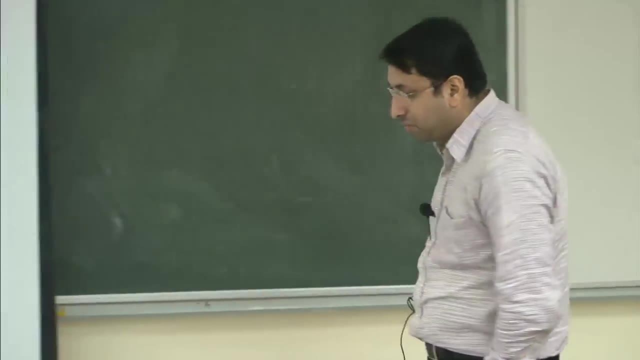 Yes, So you can run it on a small data, But that would not be realistic anymore. right? If you run it on a small data, everything will fit in my memory. I will not be able to model page faults. if you run it, even on smaller, even smaller data, everything will fit into. 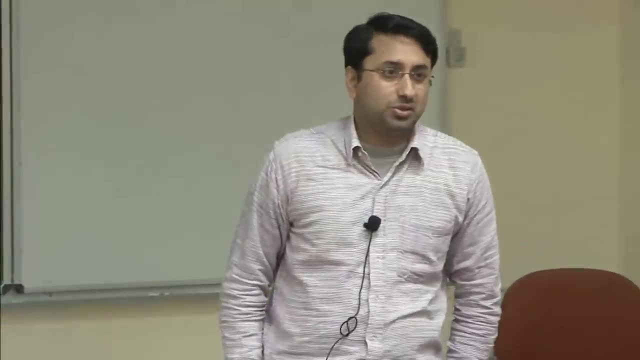 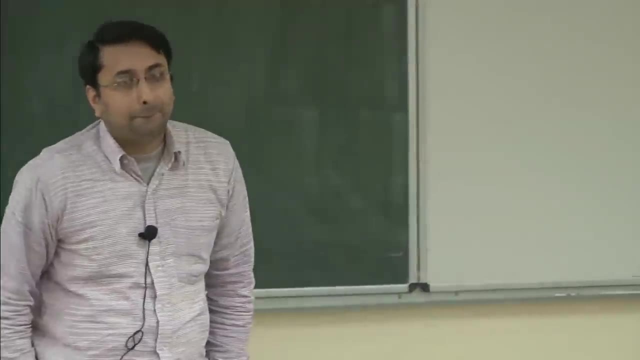 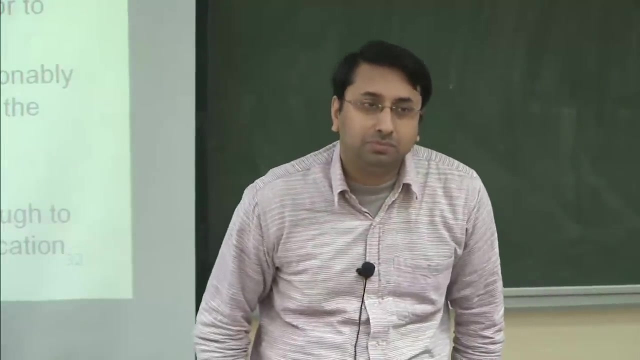 my cache, I will not be able to model cache misses. So yeah, you finished your simulation in 2 minutes, but it is useless. So try to figure out the regions in the code which have maximum complexity. How do you define complexity Means? if there are means, if it has more complexity, then we can. 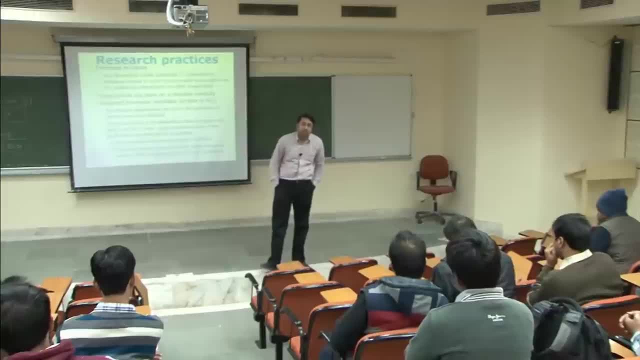 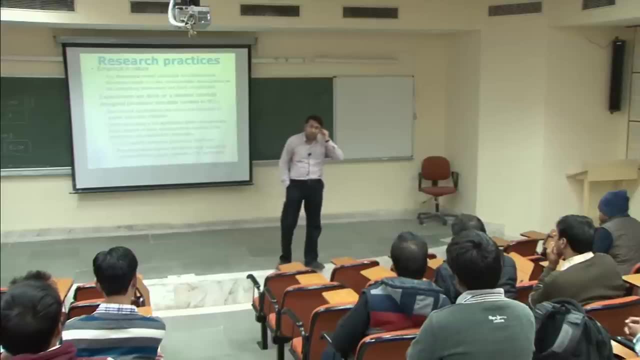 No, how to define complexity, Complexity? Complexity means that region which take maximum amount of time. So that is what he was mentioning, right, Yeah, but you do not. you do not have to run the code, you can just visually see a. Oh, you can do that. how do you do that? just by seeing, just by eyeing a code, you can tell. 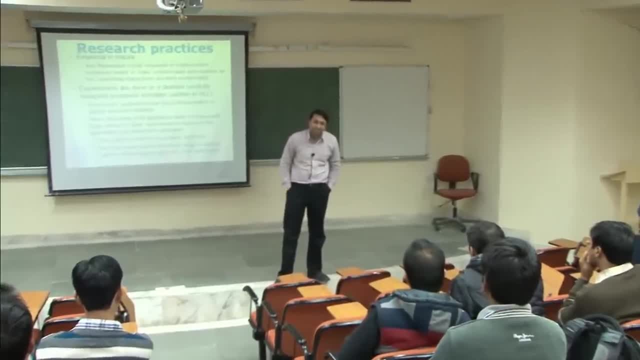 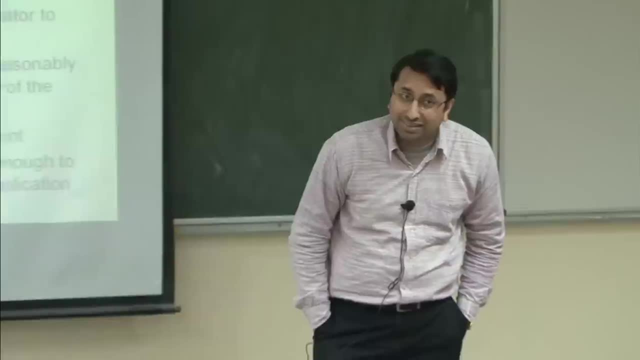 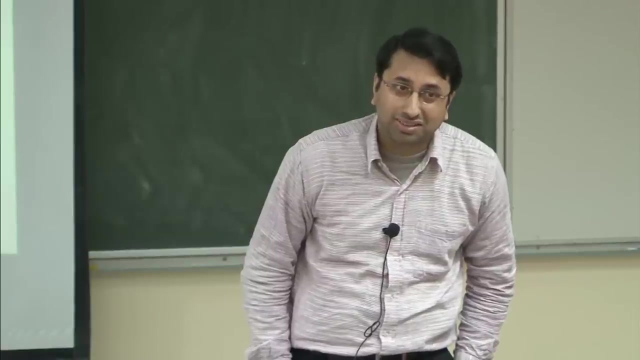 me which takes longer, which part takes longer? To some extent, you can say You can how By means. if there will be some loops and some recursion, Okay, There may be many of those. actually, how do you know which one is going to take longer? 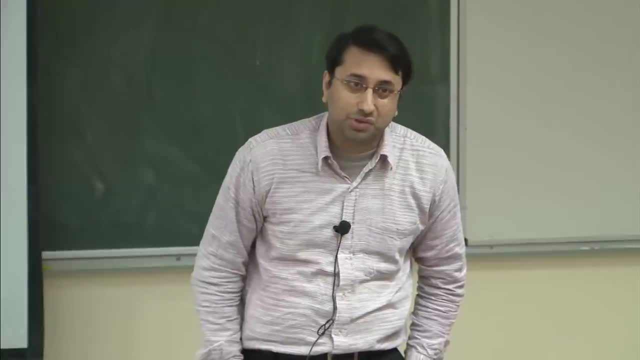 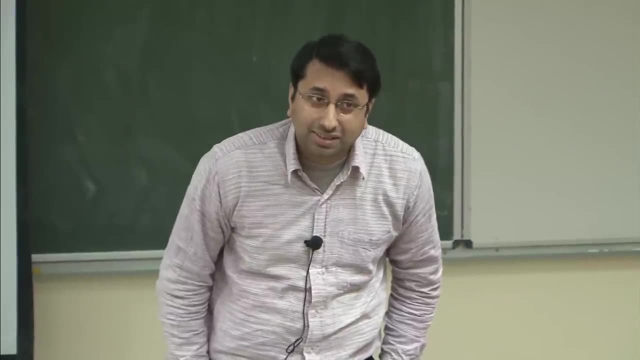 there may be you know 20 loops in your program. which one is the important loop. So we can figure out by seeing that region which region has maximum complexity. is it there Now? are you saying that the loop that is larger in size will be more complex? is that? 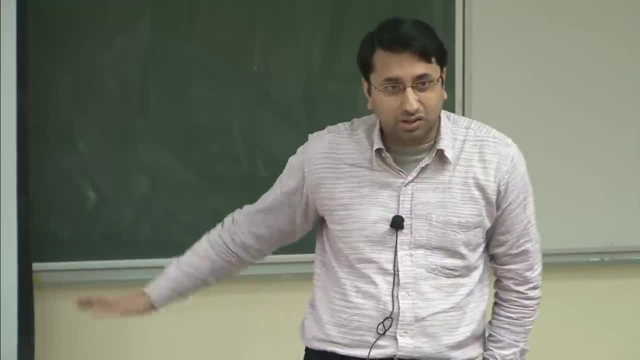 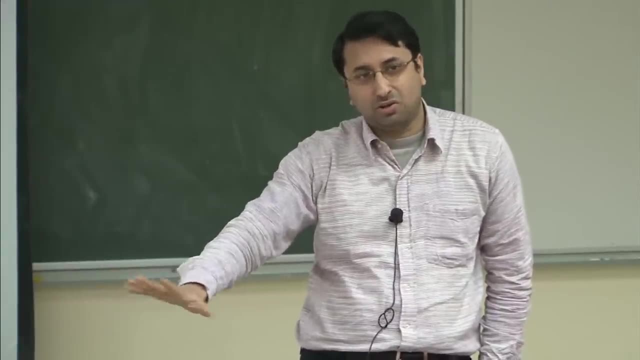 Maybe sometimes, but not always. But I need a solution which is accurate all the time, right? I cannot say that, hey, I am publishing this paper. you know, 10 percent of this papers results are correct. others may be wrong. nobody is going to read my paper, right? 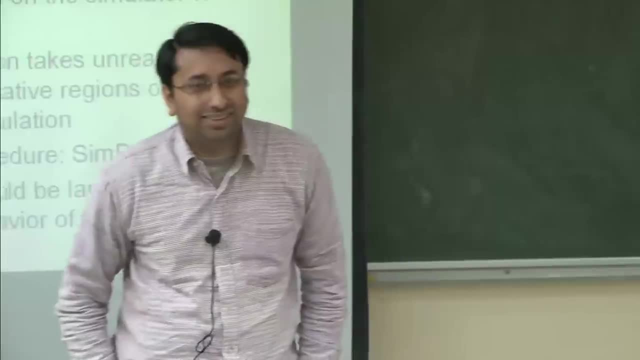 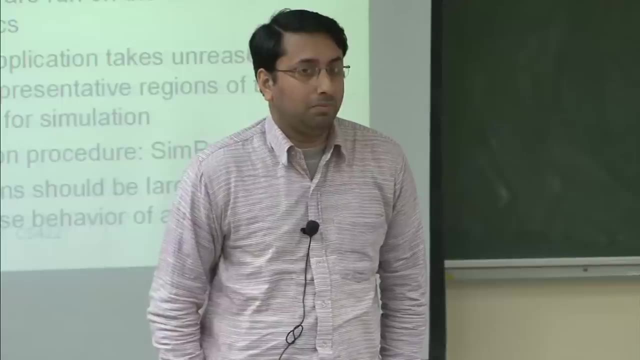 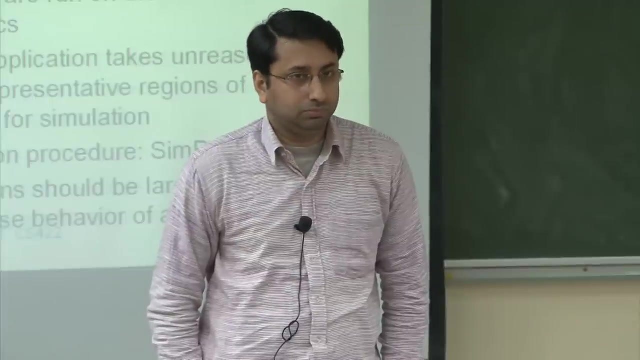 Tell me something that is a little more scientific, Sir. every program is having a path. we have a graph so we can try that each path is covered. we can have such data sets that each path is covered once at least, Okay, So that we will have less number of execution in the. 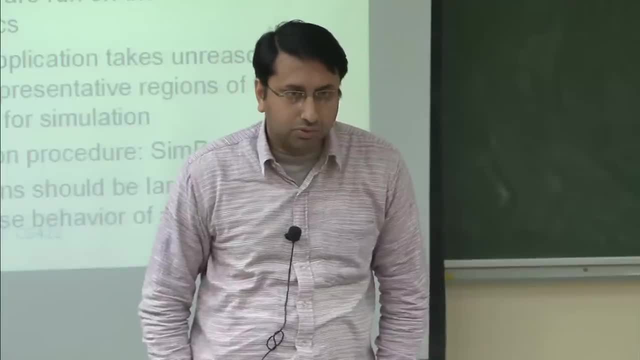 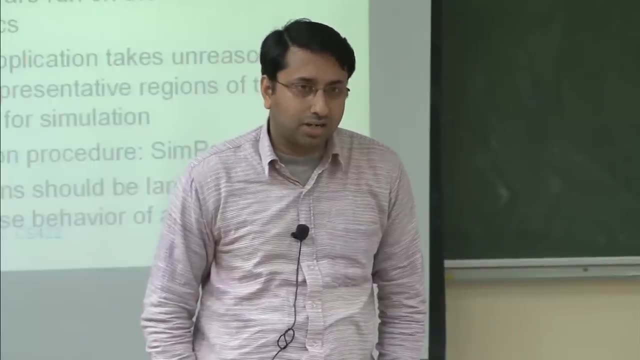 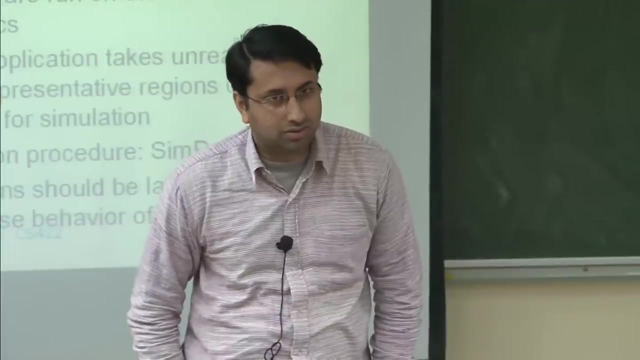 Right, So usually each benchmark application comes with multiple data inputs, and that is how the data inputs are actually designed, so that it gives you more or less 100 percent coverage of the program. Yeah, But so what? So what? Each of those data inputs will take probably months to run. 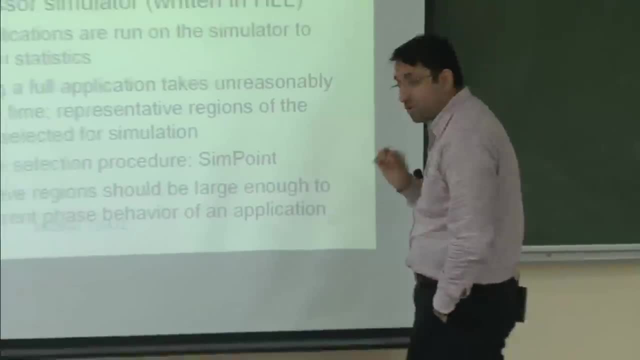 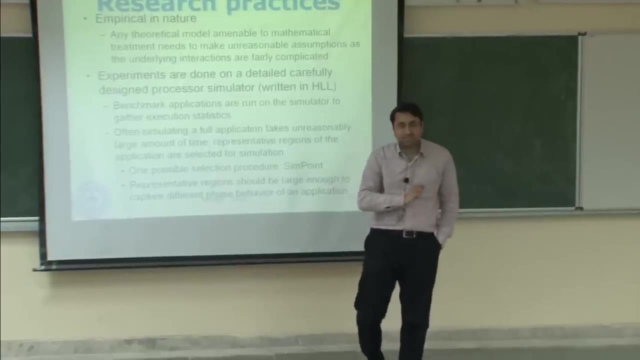 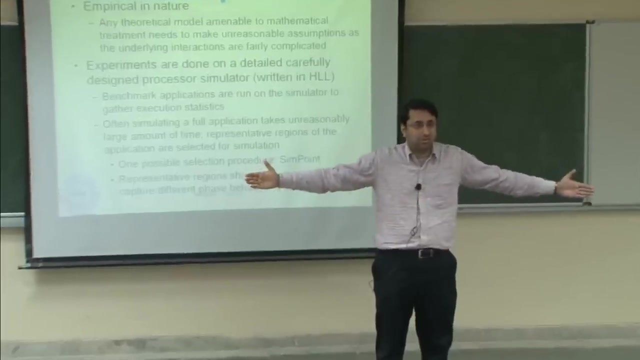 I do not know if you are understanding the question that I am asking. I give you a program. I am asking you to give me a representative region of that execution On a realistic data so you can think of an execution as what a dynamic sequence of instructions. 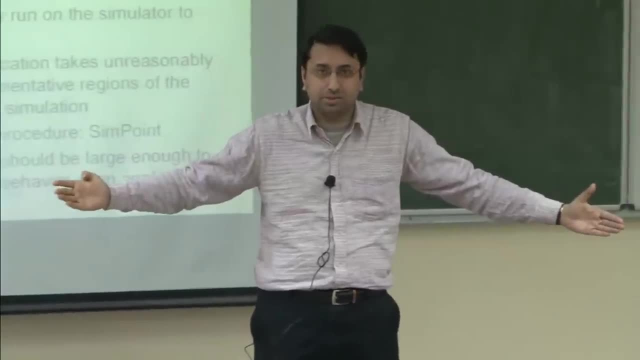 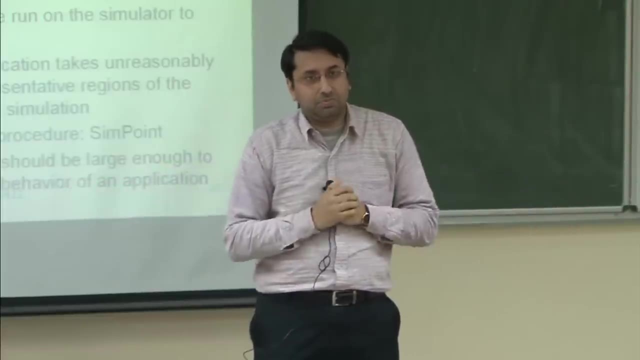 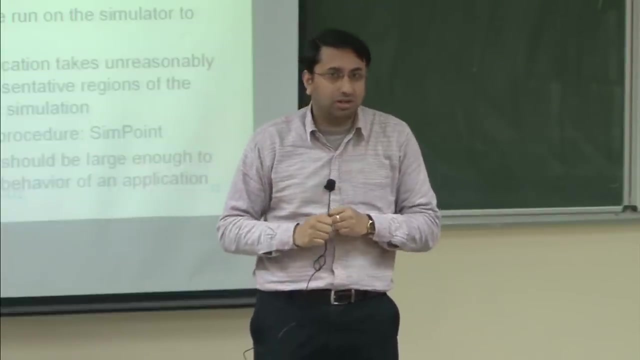 right, that is an execution. it may run for months, it may run for a minute, whatever it is. So it is a string of instructions that are given to you. I want representative portions of this. I can run. you know few such portions and I tell you that, well, you know what is. 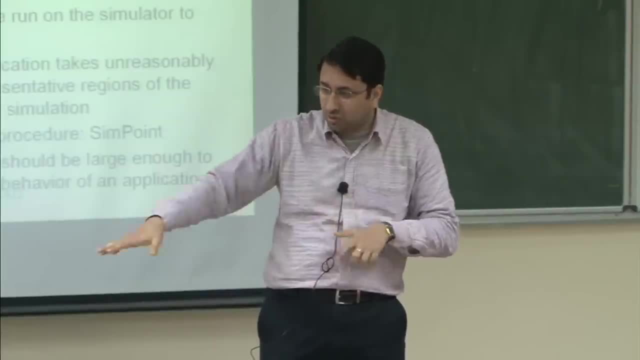 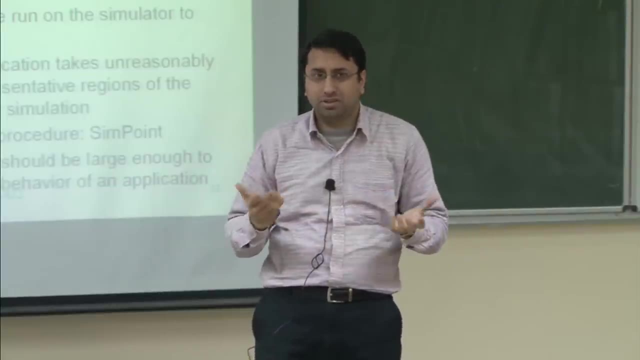 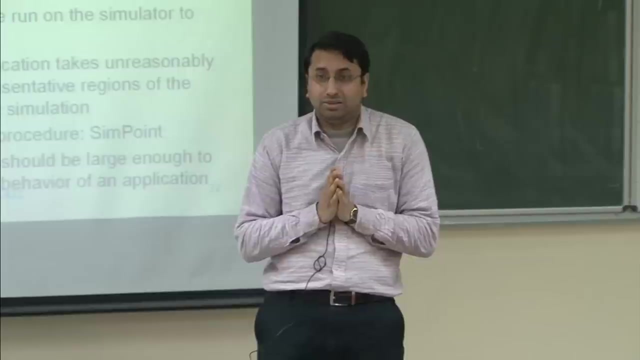 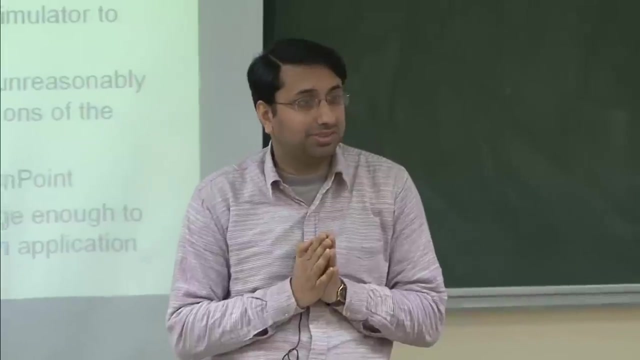 happening. So whatever behavior you are getting from this processor by running these portions is representative of running the full name. Does this problem sound familiar to anybody? No, Similar regions in a sequence: No, Nobody has seen such problems. Yeah. 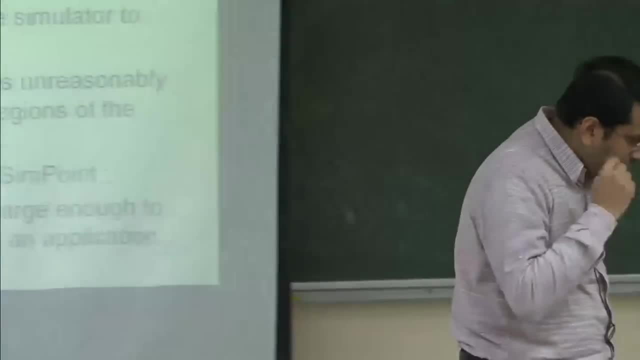 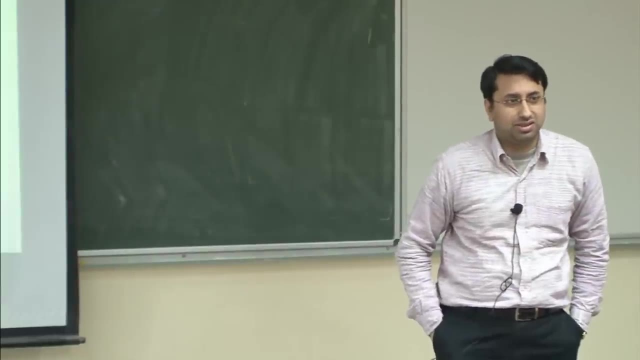 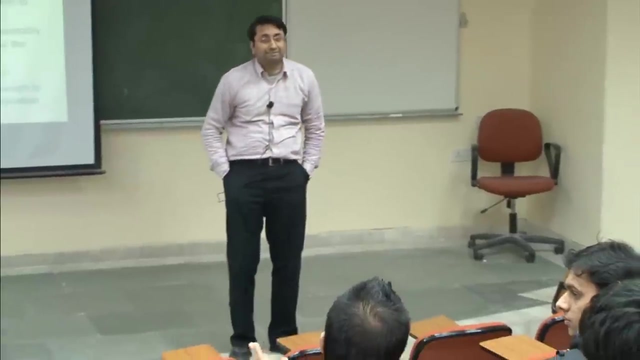 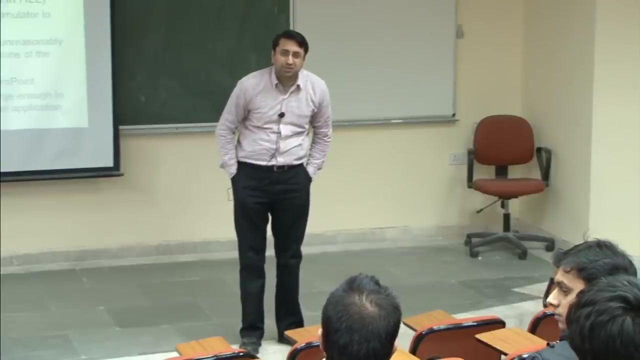 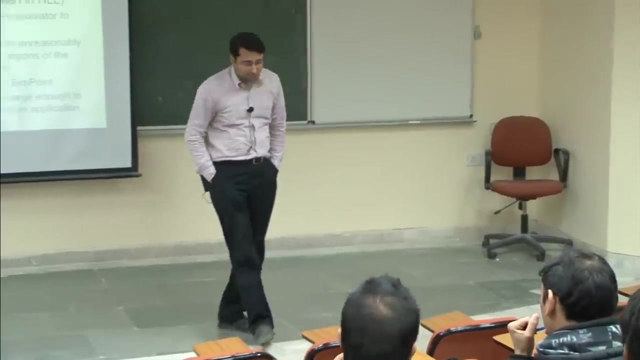 It is not common subset, exactly. I am looking for similar regions. What are they? Equivalence classes, Equivalence classes, But what are the equivalence classes here? how do I know? All are nicer sound, How you do it right, exactly. I want to find phases in. so he has used a new term. I do not know if you. 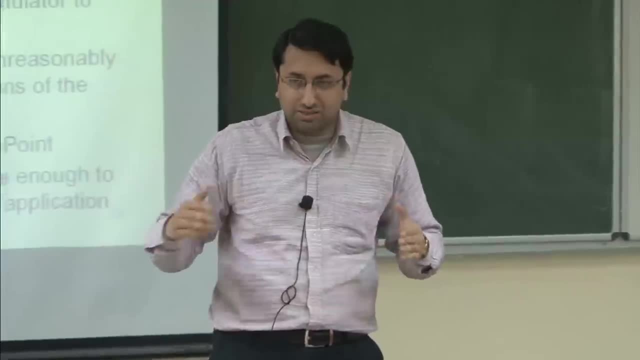 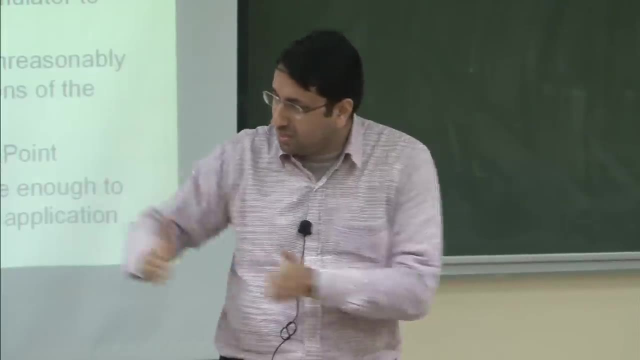 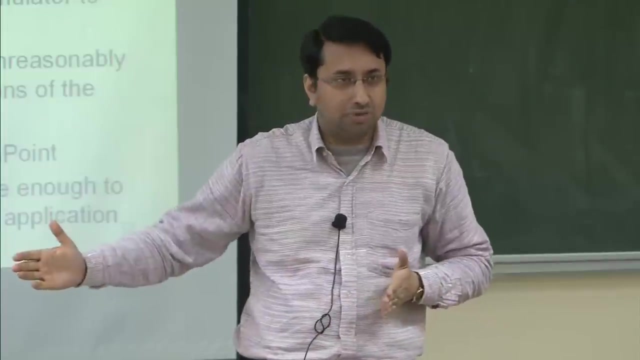 have heard of this term. phases are program regions, so that usually shows similar behavior. so one phase may come here, that this phase may repeat somewhere there again, right? so I want to pick up all the distinct phases of an execution. then I have pretty much covered everything, right? all possible behaviors, yes, so 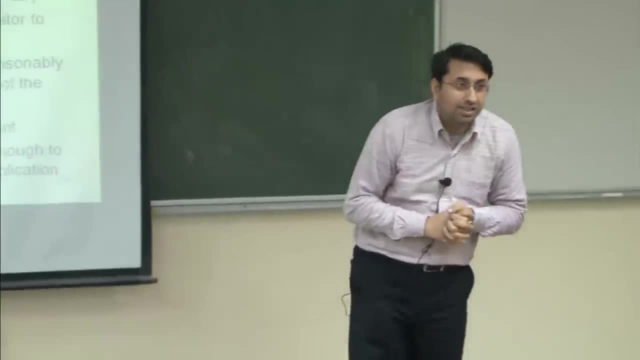 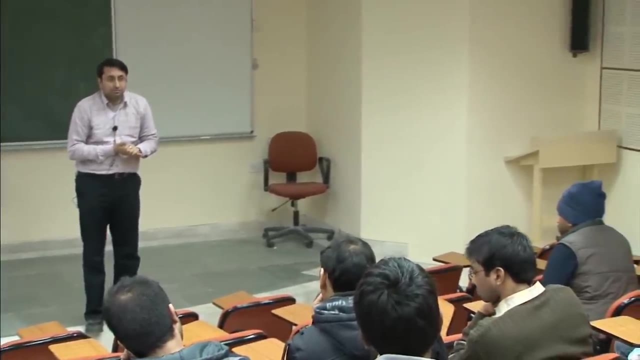 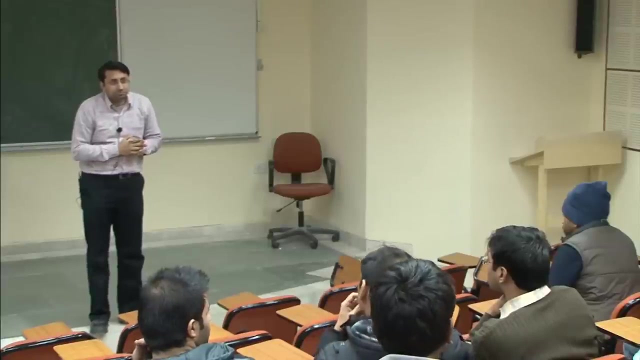 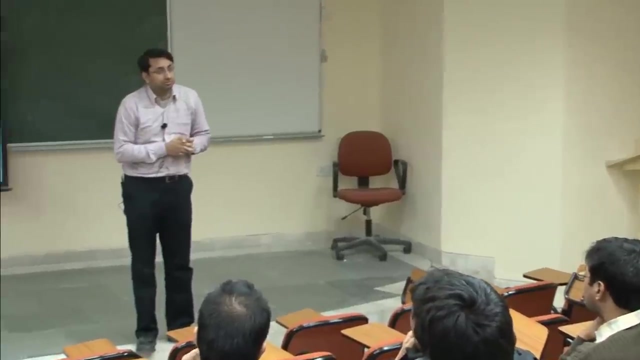 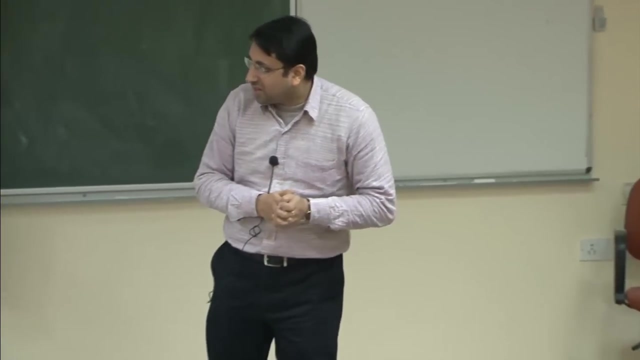 you search for the singular strings, so this phase becomes a string. yes, it is a string, it is a substring of this whole string. yeah, right, exactly. so maximum repeating substrings or repeating substrings will be, but I want all such substrings, right, right, all repeating substrings, okay, so, yeah, so this, that is pretty much what the problem. 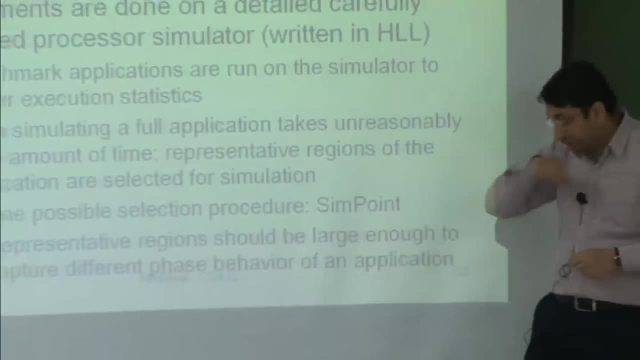 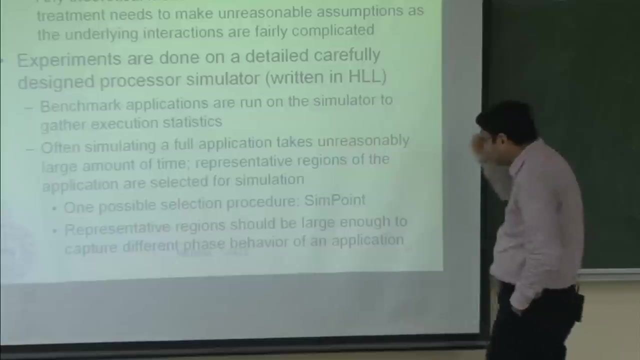 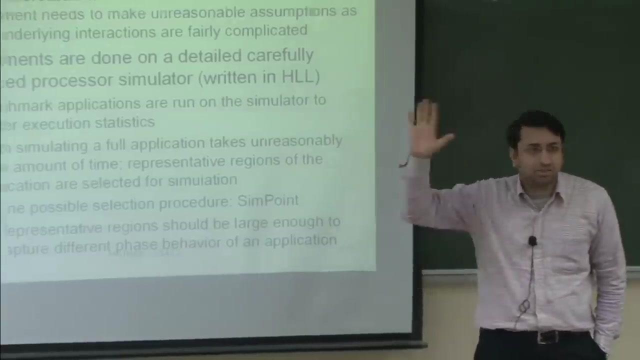 is so. there is one tool available which you can actually download, you can read about, you can go and search in google. that is called simpoint. so I will tell you what it does. it is a very simple thing. okay. who does not know about basic blocks, raise hands. okay, all right. 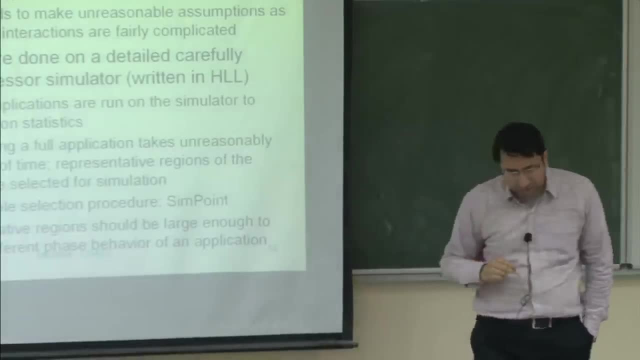 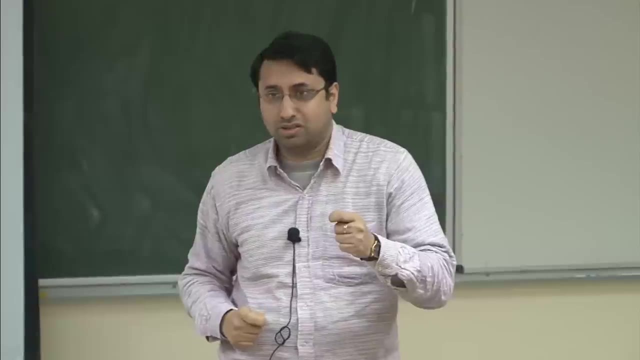 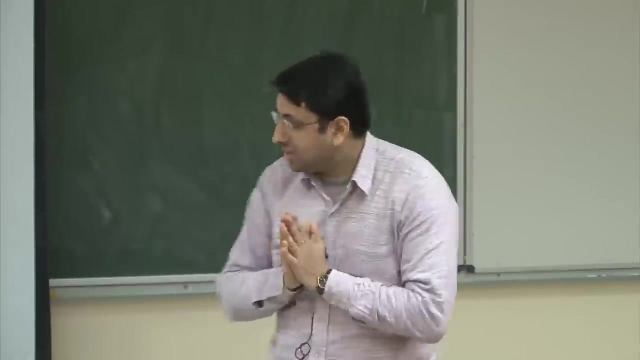 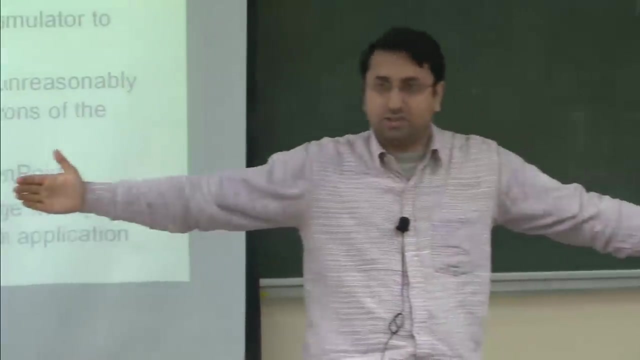 so. so basic blocks are regions of code that has one entry point and exactly one exit point, all right. so basic block is essentially a straight line piece of code. you enter here, you exit, all right. so what simpoint does is it takes this whole instruction sequence okay. 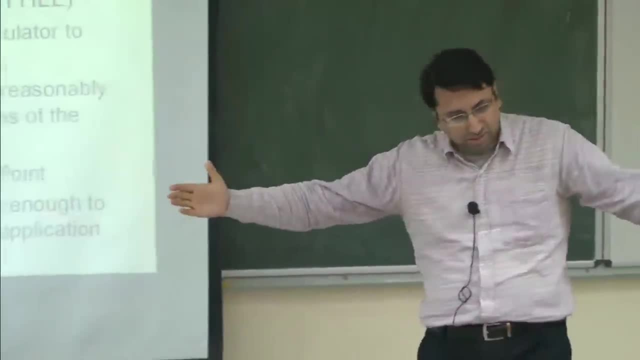 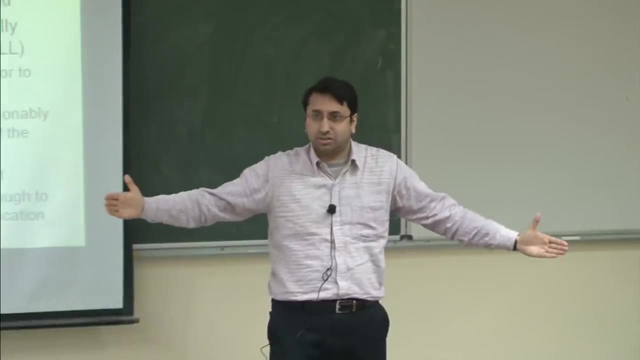 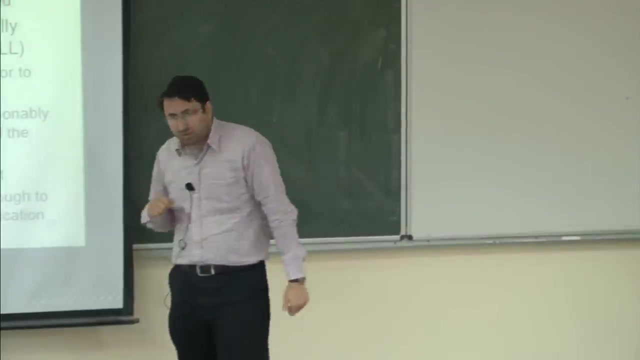 dynamic instruction sequence. okay, dynamic instruction sequence. let us suppose this just For the sake of example. suppose this length is 100 billion. let us suppose 100 billion instructions there. okay, this in this whole execution of the program. So what it does is that it asks you that you know. tell me what is the size of the phase. 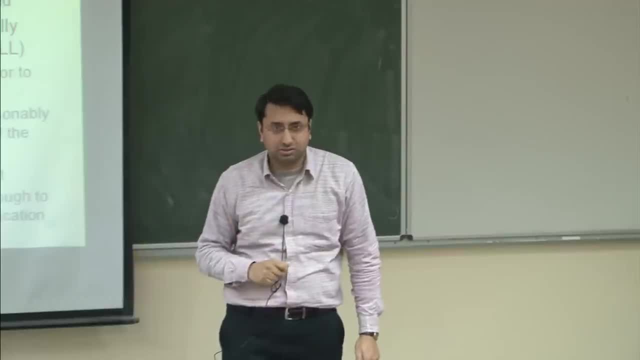 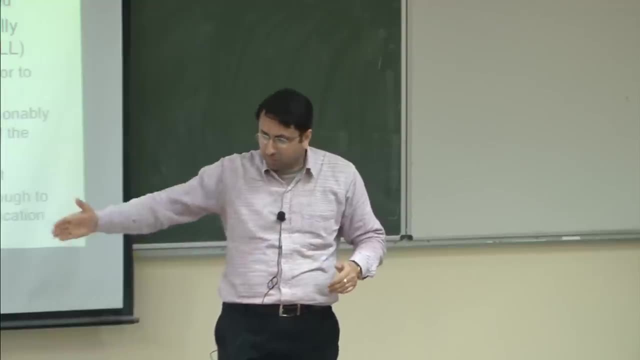 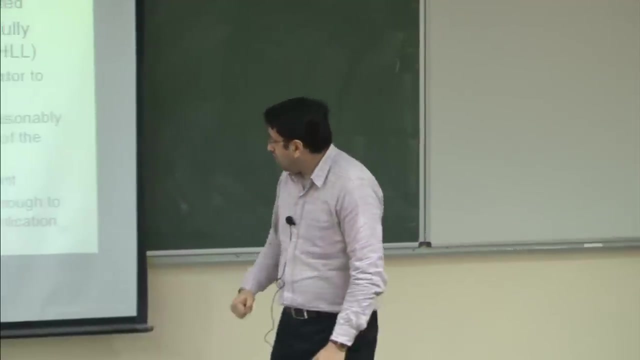 that you want. Suppose you tell it that I want 1 billion phases, 1 billion length. so why each phase should be of length 1 billion instructions? so what it does is that it chops it up into 100 different parts. all right, so 100 billion will give you 101 billion substrings, right? 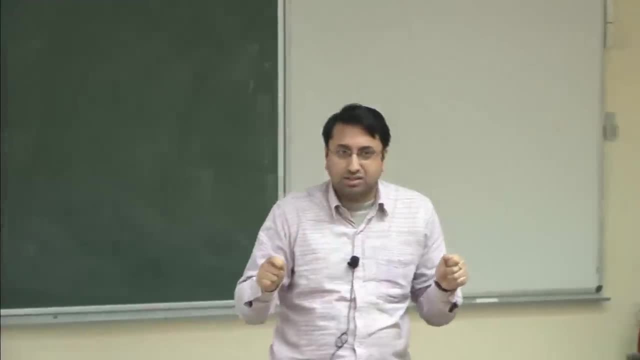 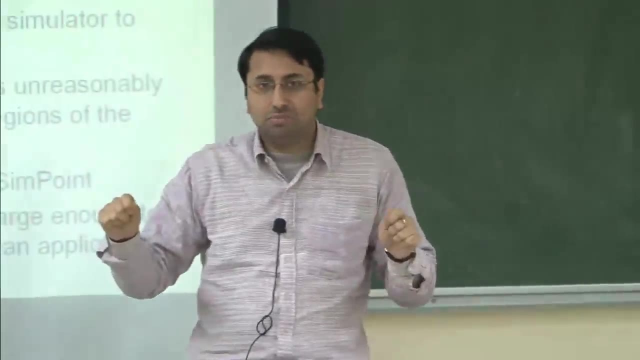 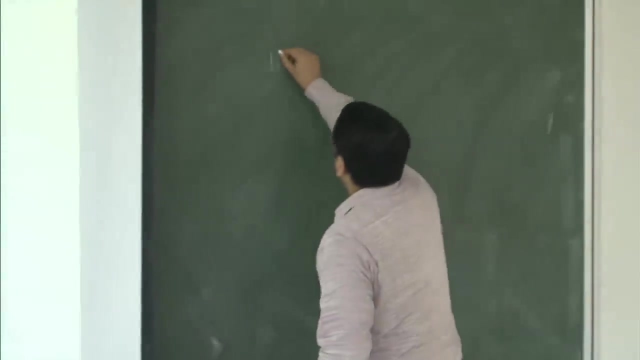 Now what it does is that it looks at each of these 1 billion substrings and encodes this one, each substring, as a series of basic block vectors. okay, So, if you so, let us suppose this is my 1 billion instructions. okay. 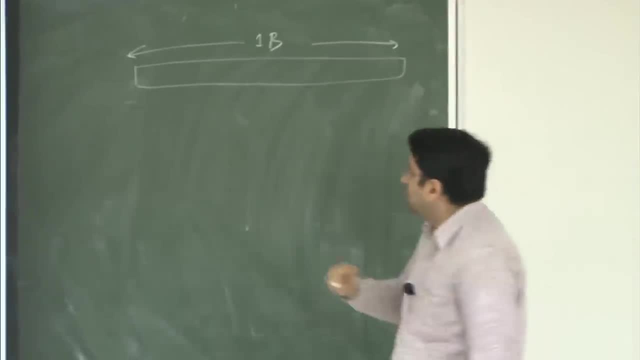 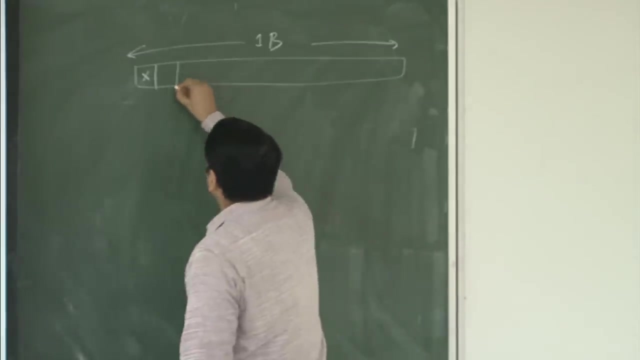 This is my instruction substring. all right, okay, If I take this instruction- the first one, it belongs to some basic block right in the program. okay, So let us suppose it belongs to basic block X, right? The next instruction probably belongs to basic block Y. 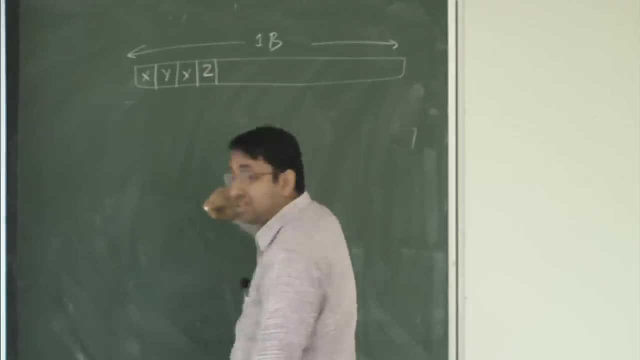 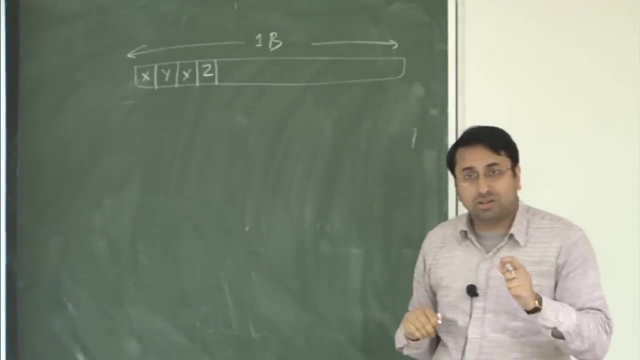 This one belongs to X. again, this may belong to some other, Z, and so on and so on. okay, all right. So if you scan through this, what you will get For each block, For each basic block, you are going to get a count. 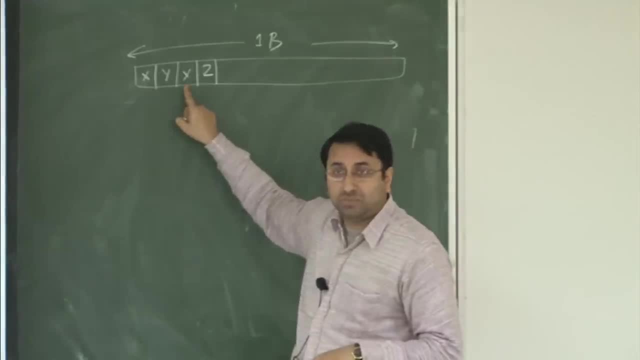 For example, here I have shown a count of 2 for basic block X. So at the end, what you can do is you can answer the following question: that in this 1 billion instruction string, how many times did I visit basic block X? 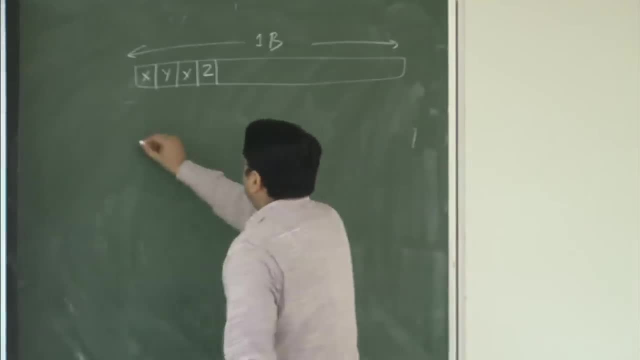 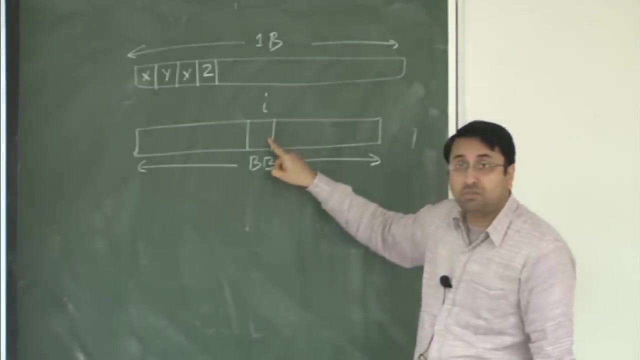 That should be a number, right? okay, So it builds a vector from this. The length of the vector is equal to the number of basic blocks that you have in your program And the entry I tells you number of times you visited basic block I in this instruction. 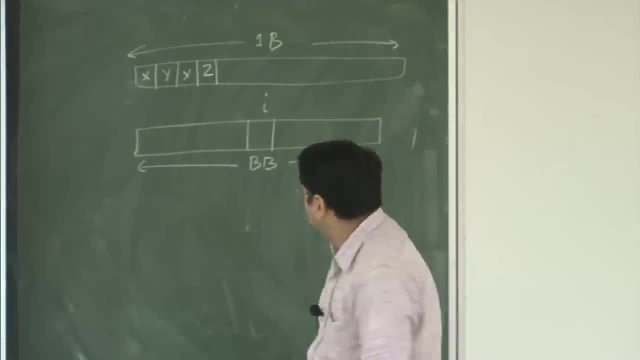 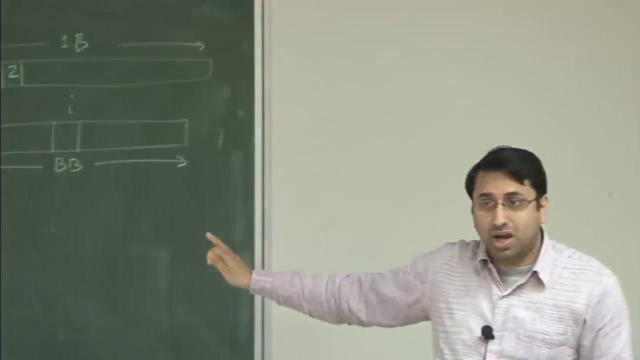 sequence. all right, clear, okay. So let us suppose I have n basic blocks in my program, so this is an n-dimensional vector, integer vector. okay, clear till now. So I am going to get 100 such n-dimensional vectors right from my 100 billion instruction. 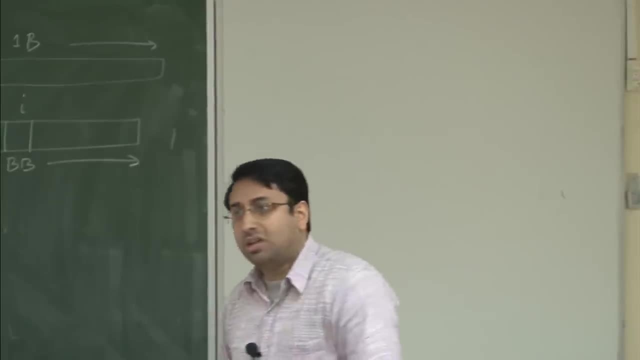 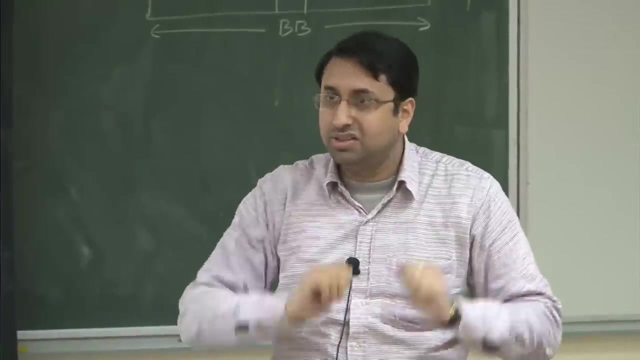 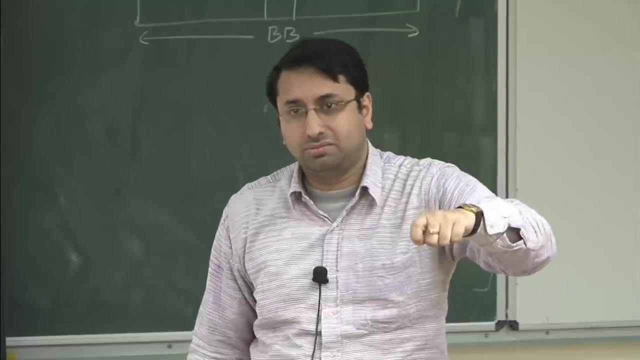 sequence. So now it becomes n-dimensional. Okay, So it boils down to clustering these 100 vectors in a dimensional space. okay, And what I will do is that, once I have clustered, my clusters will have similar vectors and I will pick the vector closest to the center of each cluster. 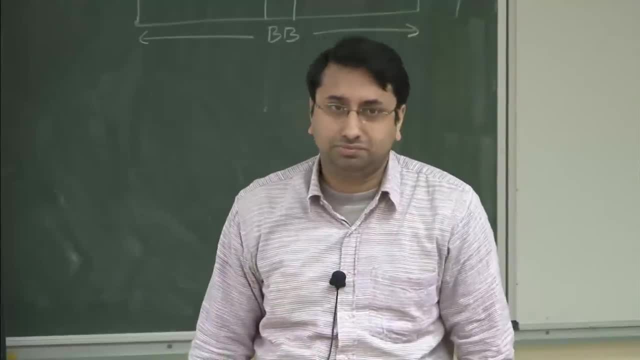 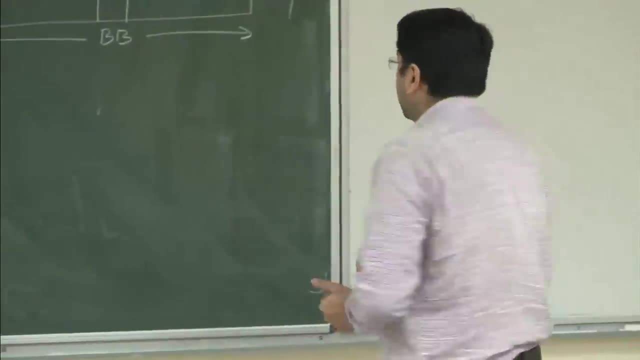 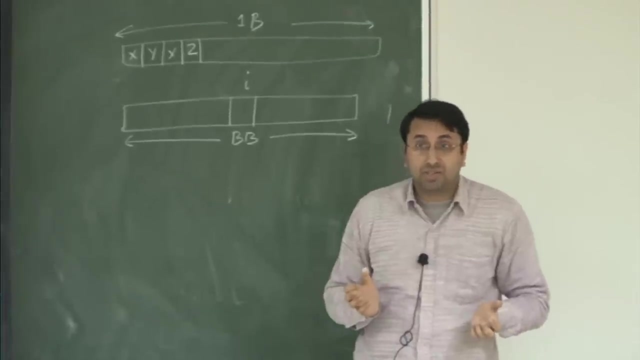 That will be my representative: 1 billion instruction periods. is it clear? You may not know what, how you do clustering, but clustering essentially clubs together the similar vectors. okay, all right. Is it clear? If you just want to run one representative region of 1 billion instructions, what can? 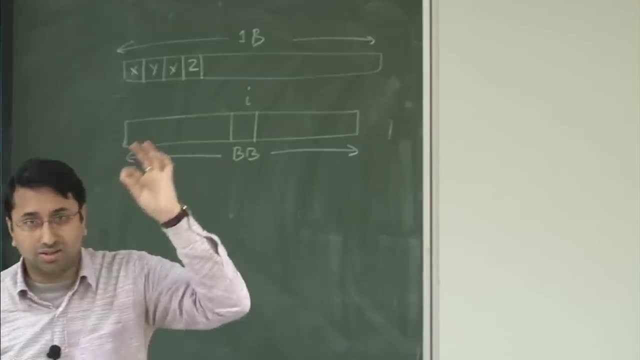 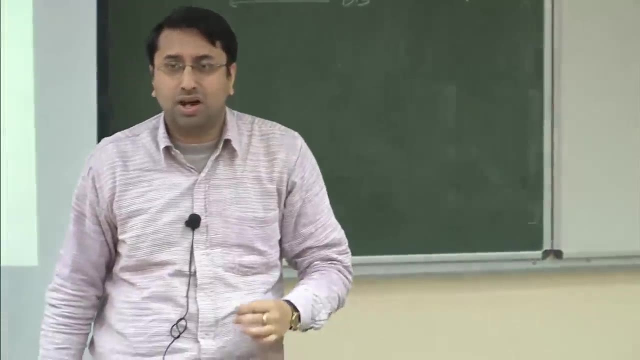 you do. Can anybody suggest One cluster? Just one I want to run, because I can suppose somebody tells you that my simulator is so slow that I can only run 1 billion instructions, not more than that. what can I do? 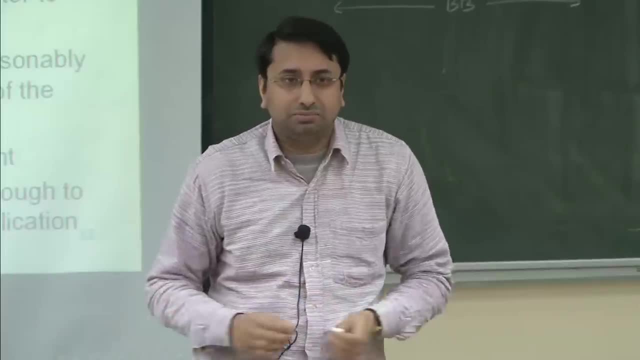 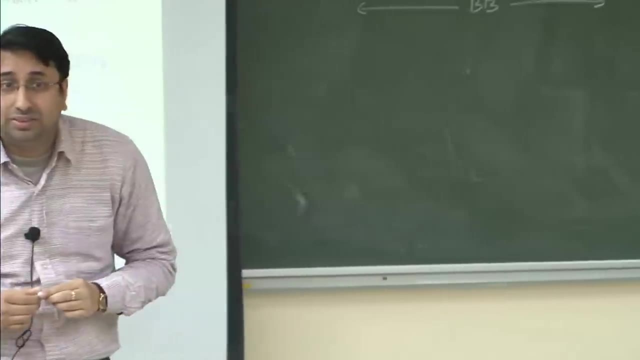 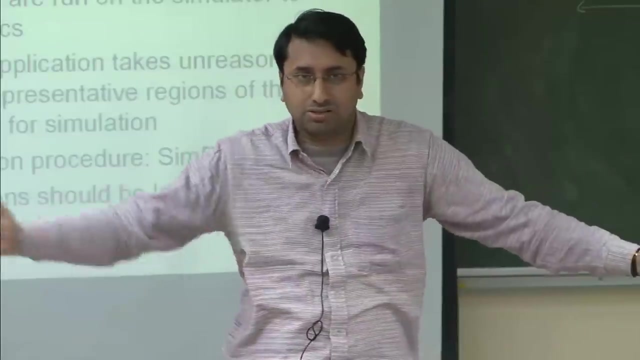 I have to pick one of these 100.. Okay, So you will bring. let us take a look at this. which one should I pick, Right? which one should I pick Most frequent? most frequent ones, Most frequent one. 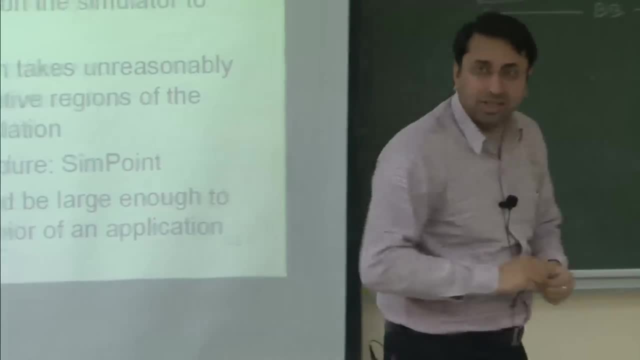 What do you mean by most frequent? These are all distinct, right? I have a 100 billion instruction sequence. I have chopped it up into 100 parts In the center of this vector, The one that is closest to the center of this of this vectors. okay, right. 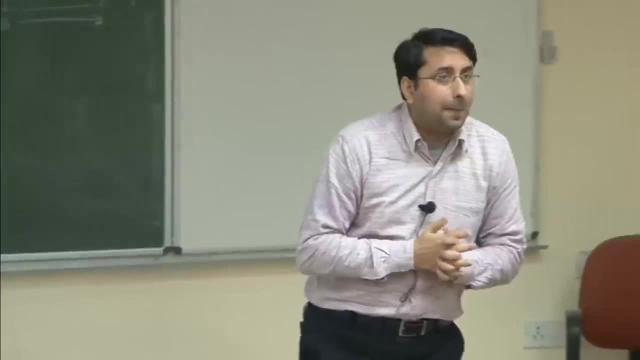 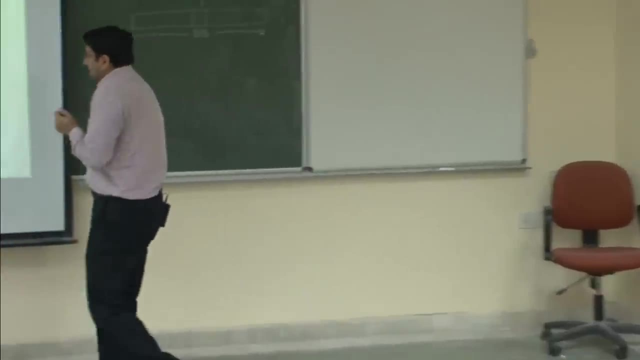 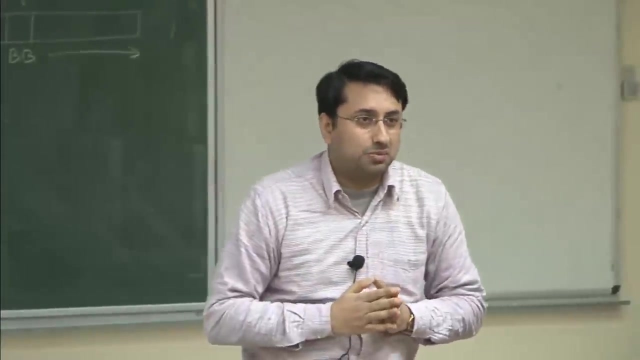 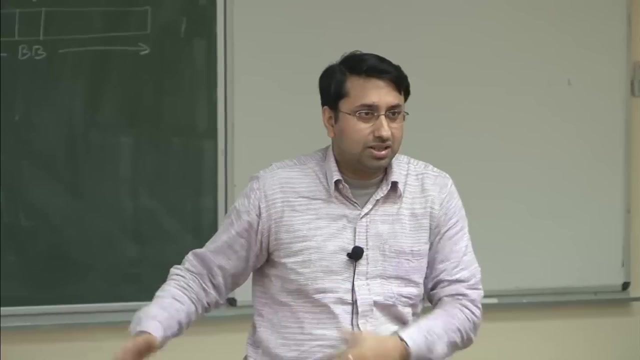 Okay. So these are sorry. I have a question, Sorry, yes, Okay. so yes, here the assumption is that you are what you execute, so the piece of code that you are executing should manifest your behavior. that is what the assumption is here. 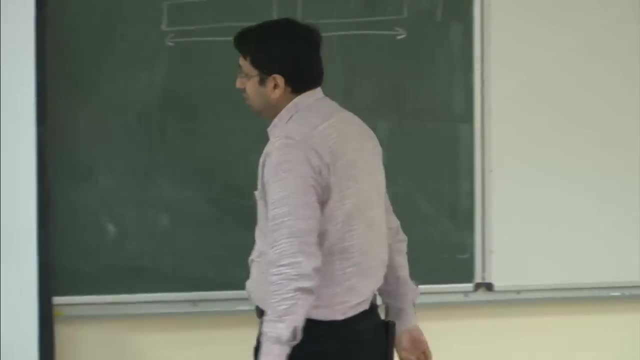 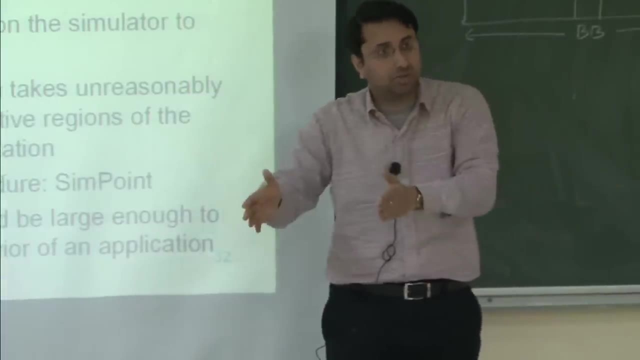 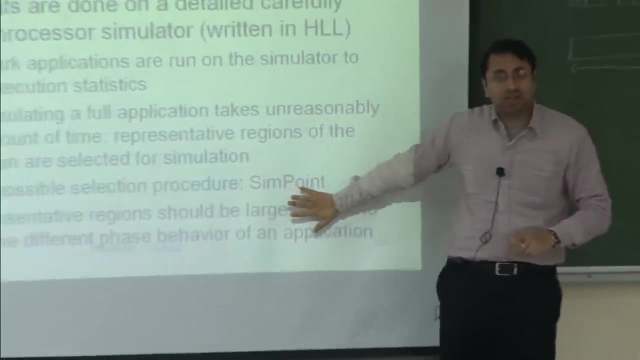 and it actually follows- pretty accurate in most cases- that your the set of instructions that you are executing roughly tells you your branch prediction behavior, your memory behavior and many other things. It is a very simple algorithm. you can, of course, improve it significantly in that. but to start, 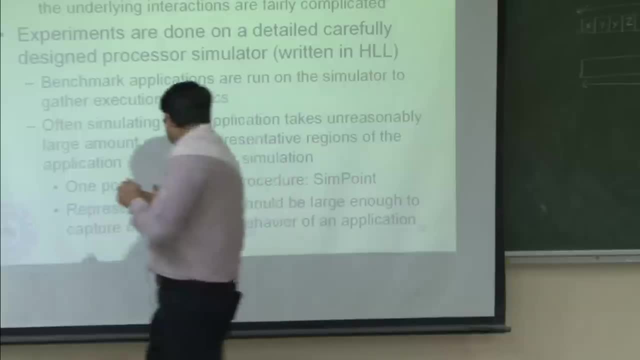 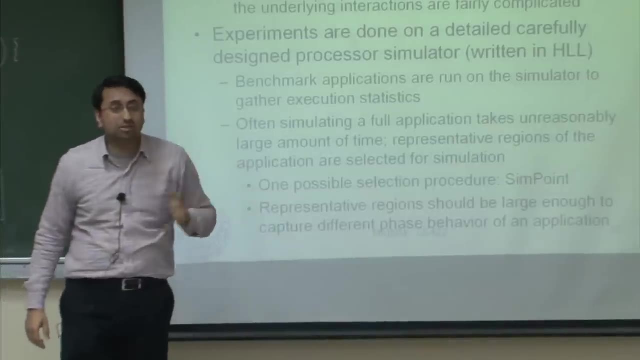 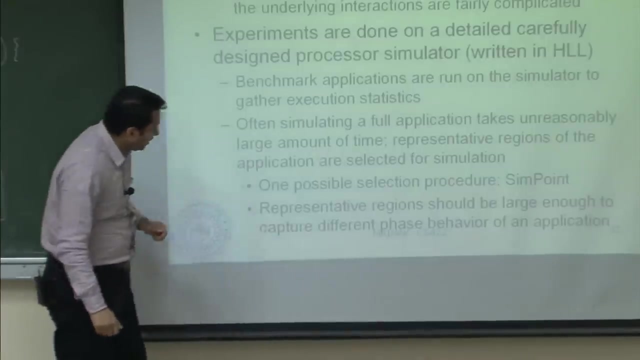 with is a good one. So, representative regions, so the. so one thing that we assumed here is that parameter right, 1 billion, which is the point we will ask you that tell me how big a phase you want. So here you should be careful. these regions should be large enough to capture different phase behavior. 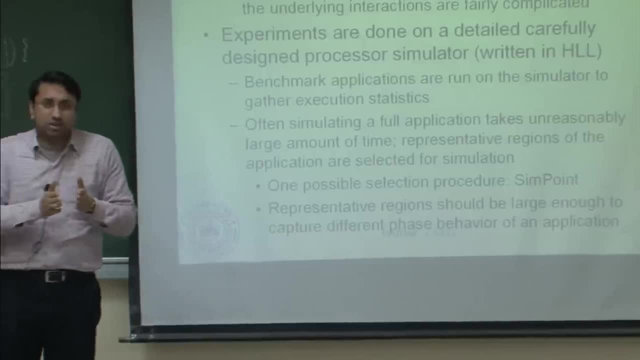 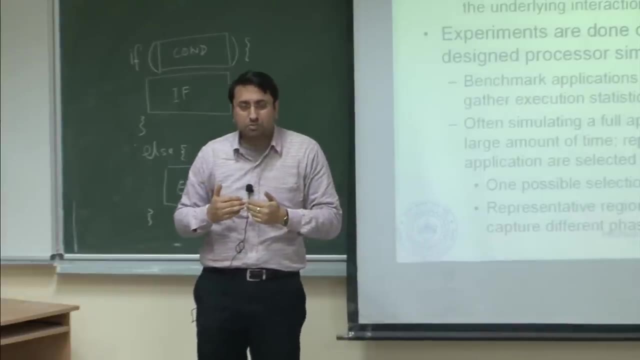 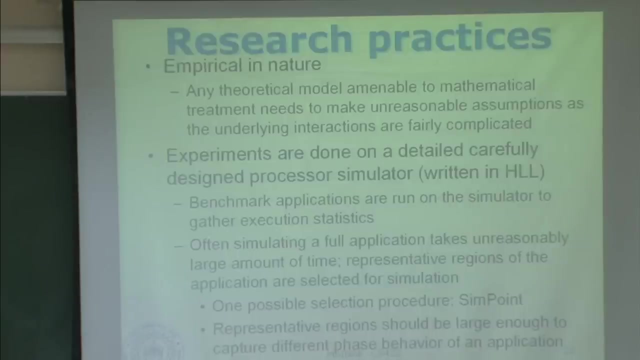 of an application, so it should not be too small. and if it is too large- and of course you lose the whole benefit of doing this- you will. you are actually now approaching pretty much simulating the whole application, Any question. so if you want to read up on this, you can just go and search in google. 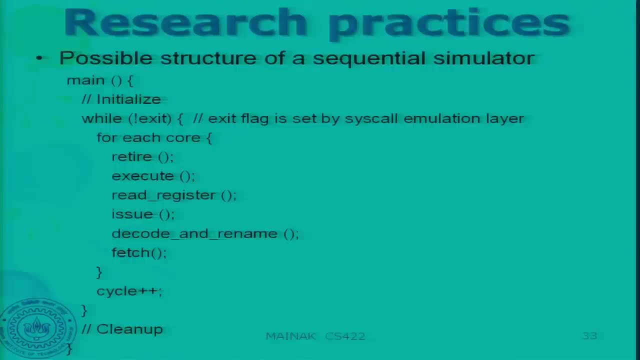 so how does a simulator look like? So here is a possible structure of a sequential simulator. so this is the main function of the simulator. it would first initialize bunch of states in your simulator. by the way, this is over simplified, so usually a simulator is several hundreds of thousands of lines. 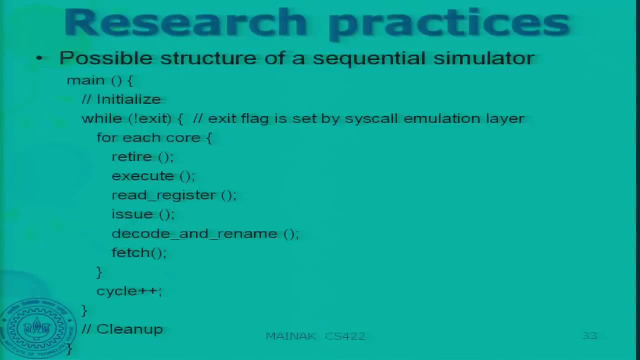 of code. it cannot fit in a slide out of question, but this is just a skeleton. so what you do is then you run a while loop which says: while not exit, where exit flag is usually set by the system call emulation layer. when your program exits, 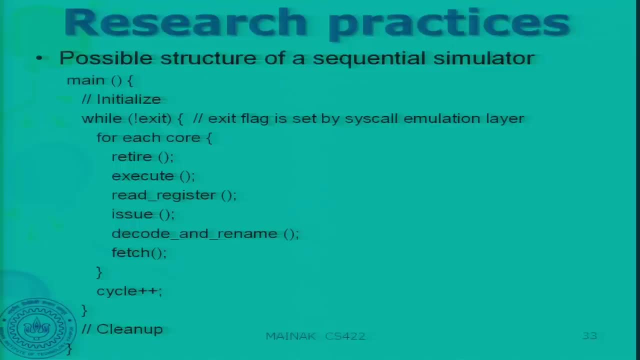 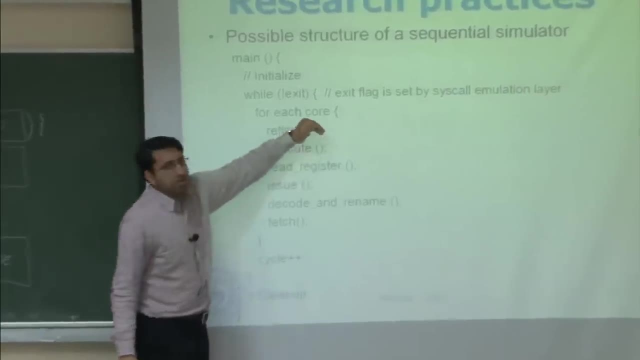 When a program makes the exit call, this exit flag will be set at that time. okay, until then you keep on running. so what do you do for each code? so I am assuming that you have a multiprocessor, so for each processor code you would go and do something in each cycle. 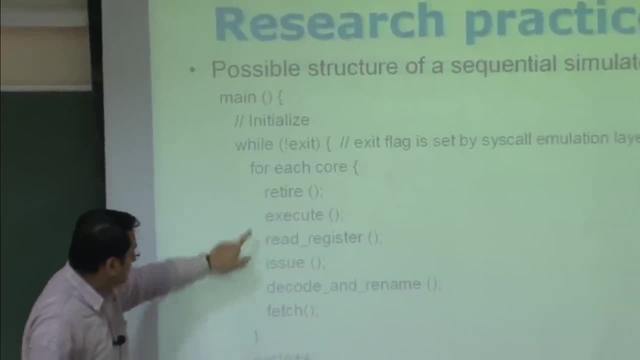 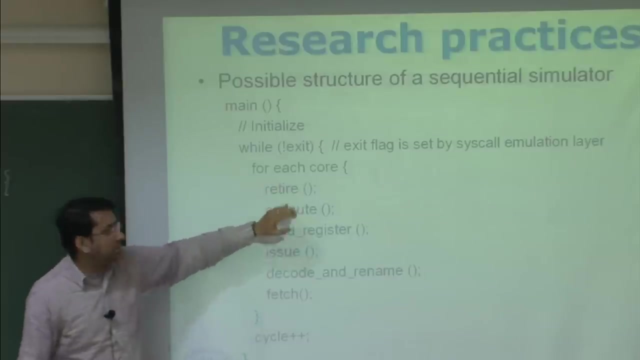 what do you do? So you first. so this is: this is a pipeline of a processor, Okay, which we haven't talked about. we'll soon get there. You'd first retire that any. so retirement means completion of an instruction. You'd complete any instruction that is pending in this cycle. 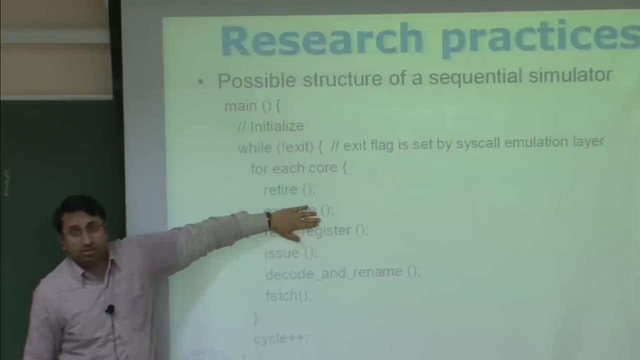 Then you'd go and execute an instruction that should be executed in this cycle. You'll find out the instructions that are waiting to read registers. you'd read those registers. You'd issue the instructions that are waiting to be issued in this cycle. You'd decode and rename instructions. we'll talk. 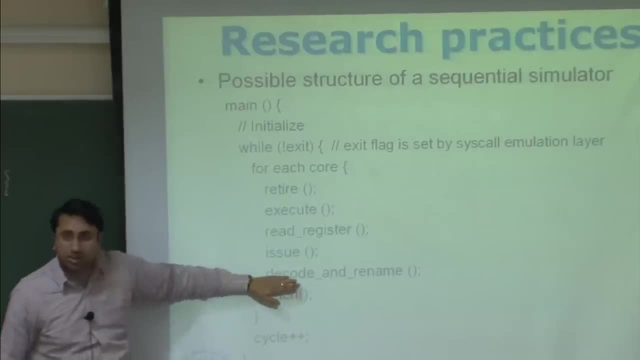 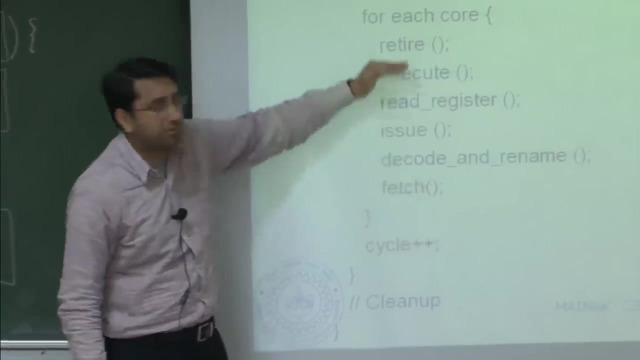 about this particular phase of the pipeline soon. Decode should be easy to understand. What is rename? we'll talk about And you'll fetch any instruction that should be fetched in this cycle. These are distinct pipeline phases. okay, all right, And then you do this for each code. 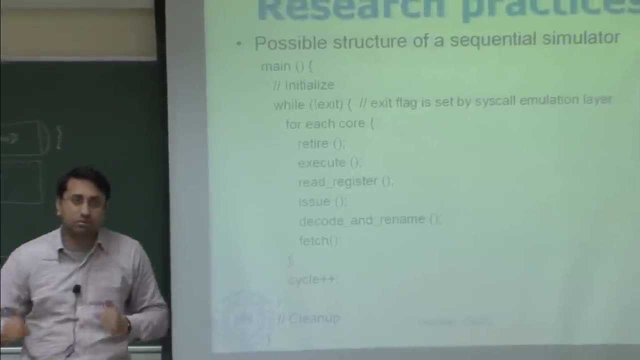 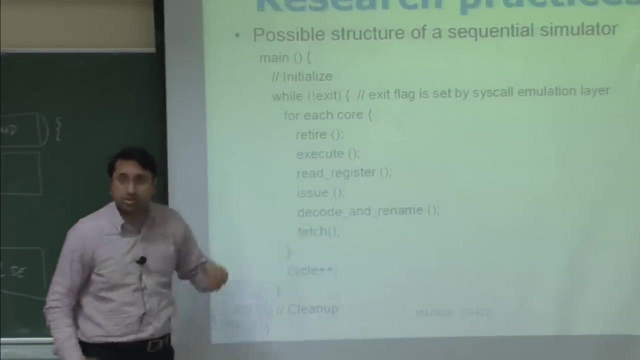 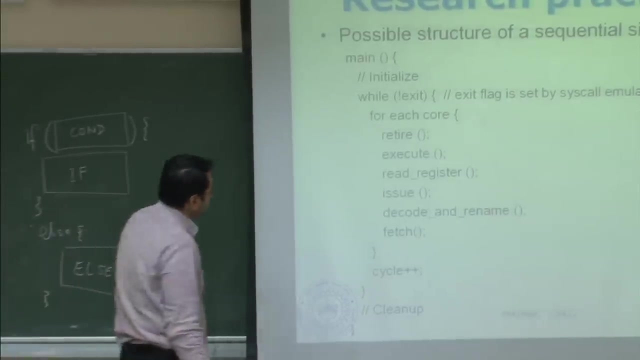 and then you increment the cycle count. That's one cycle of your simulator. okay, all right. And when the exit is set, you have essentially simulated your processor pipeline for this program and you exit, all right. So we'll talk about these pipeline stages very soon, okay. 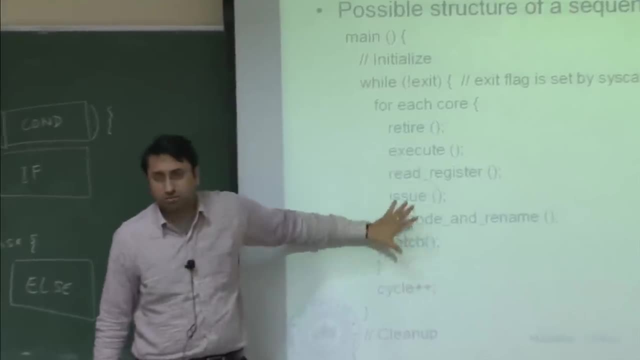 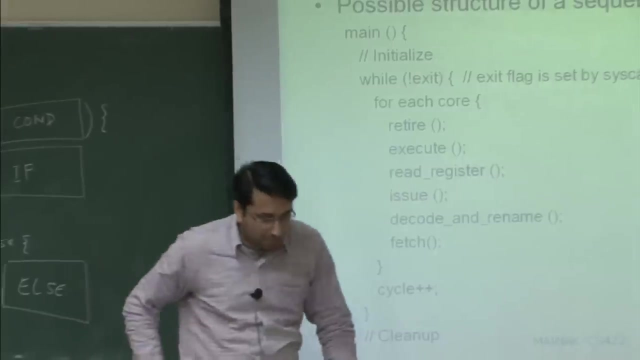 Just currently. just think about these as some phases of execution. okay, An instruction starts at fetch and leaves the pipeline here Upside down. I mean, should we? Yeah, So can somebody? I was actually trying to avoid this question right now. 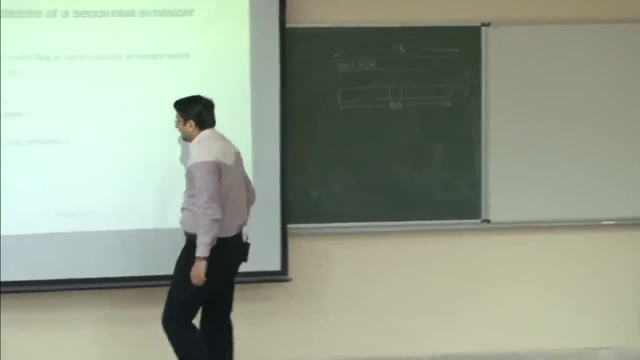 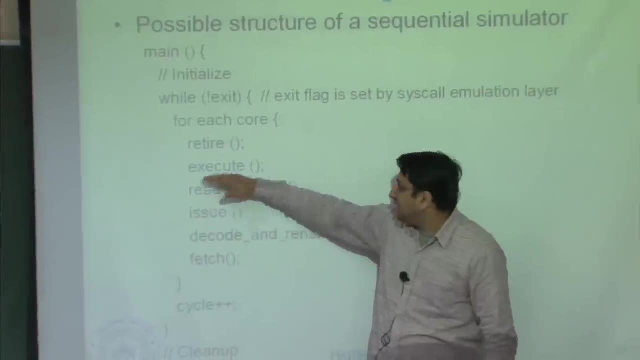 But since he has asked, so what? he's pointing out that an instruction really starts here, right, It is fetched and then decoded, then issued. then it reads: register operands, Executes and then completes. Why am I putting it in the opposite order? 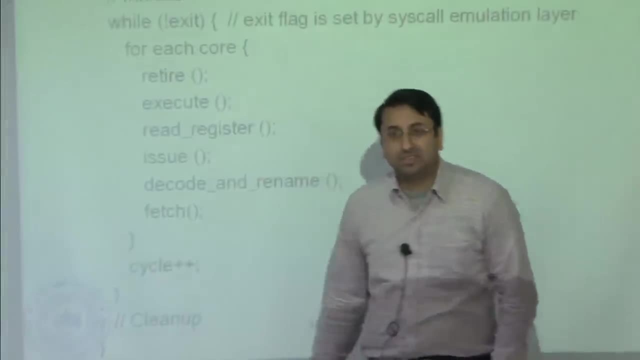 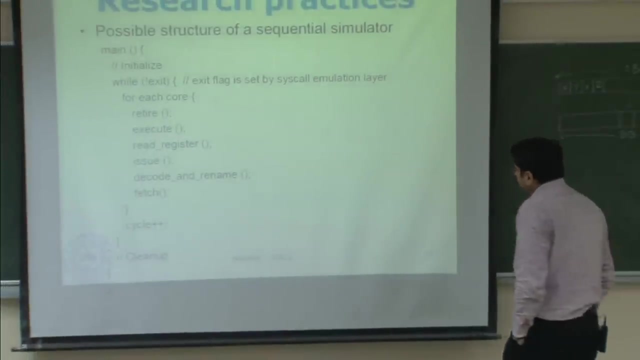 What would have happened if I put it in this order, in the other order, Sir? Yes, So while retiring, you're creating space for the instruction that will get executed and will fill up the gap. So, basically, I'm taking this in the pipeline. 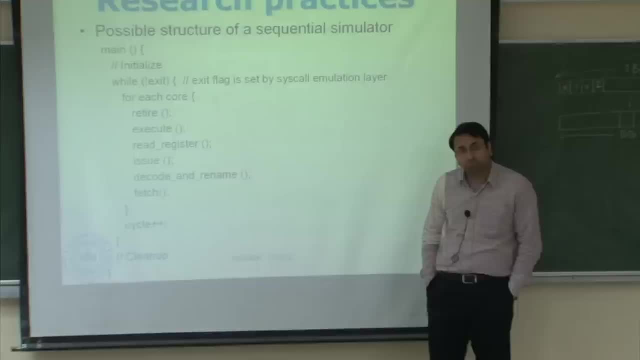 and then shifting them all by one. Okay, So if you do it in the other order, then well, if you do the first, Then there's already one. some instruction that is blocking that which is still waiting to be fetched. You can't overlap the two, right? 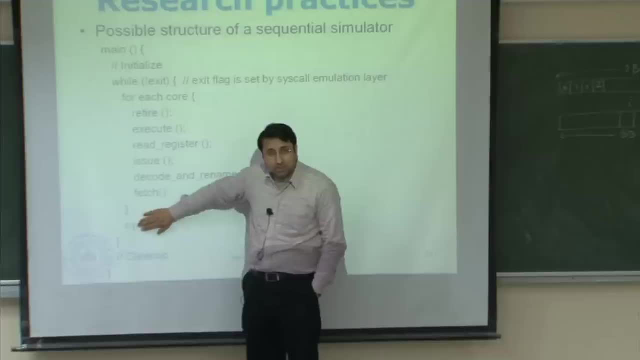 There's no space. So you're talking about freeing up the space. So you're assuming that there is some space allocated for the instruction to be fetched, Like some, maybe some resource, Some resource, Yeah. So you have to first empty it and then fill it. 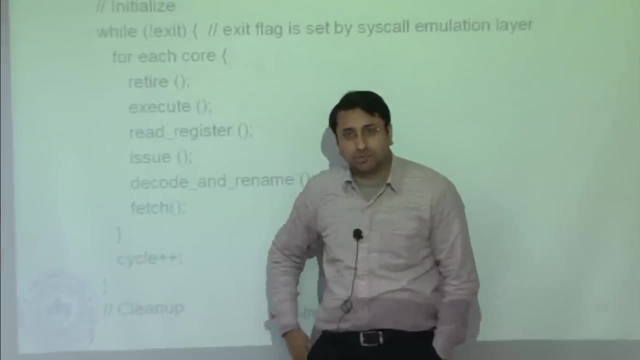 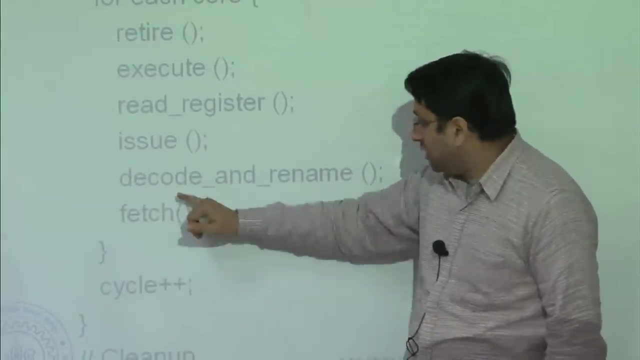 Okay, I could oversize that. But there is a more important reason why I don't do it. If I put the fetch, The upside down this whole thing, what will happen? I fetch an instruction and when I invoke decode, I'll decode that instruction only right in the same cycle. 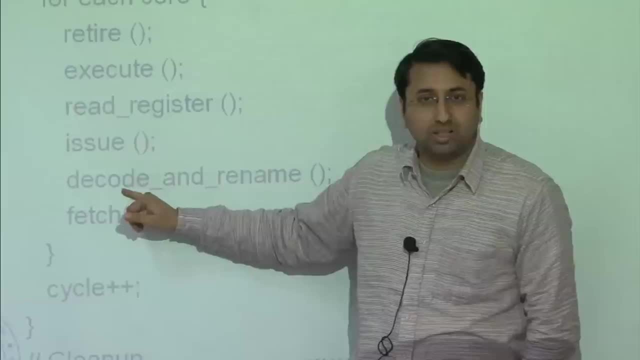 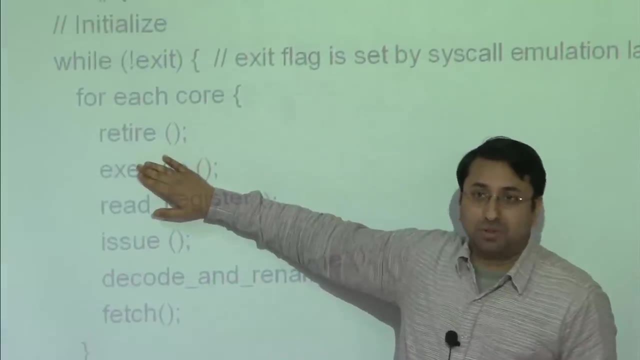 But that's wrong. I shouldn't be decoding that in this cycle. It should be decoded in the next cycle, right. By invoking the pipeline from the end, I actually avoid that problem. I complete the instructions that have to be completed in this cycle. 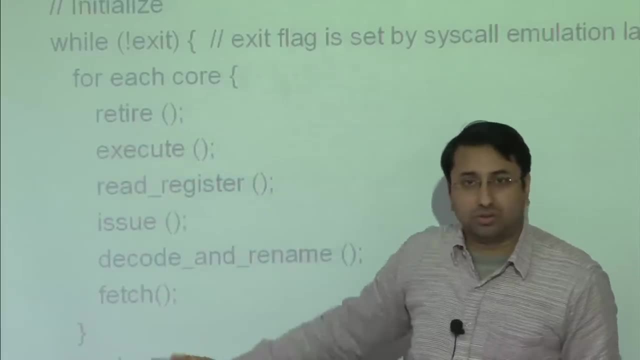 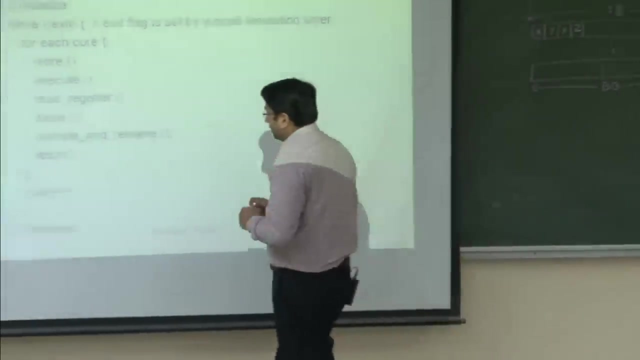 Then I find out what is to be executed in this cycle, I execute them and so on and so forth, And at the end I fetch. This makes sure that And instruction will not be fetched in the cycle and will also get completed in the same cycle. 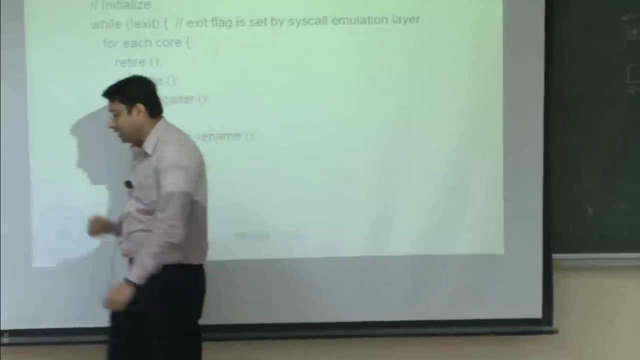 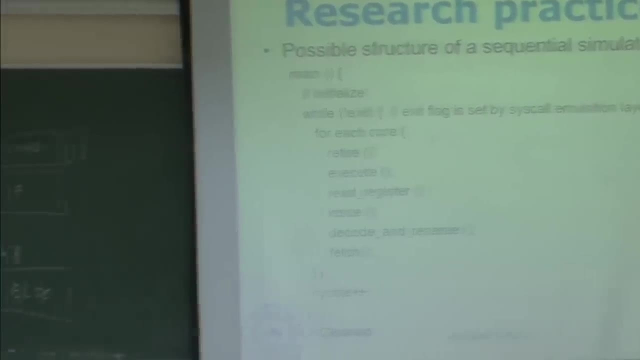 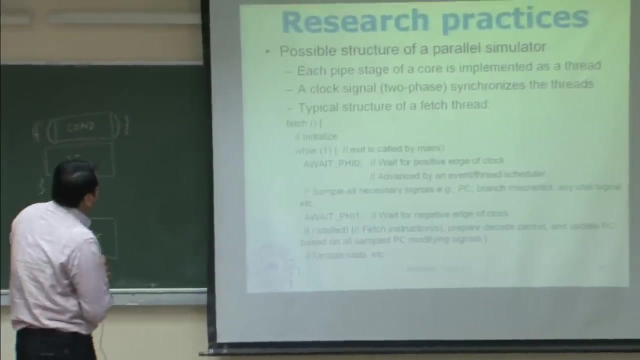 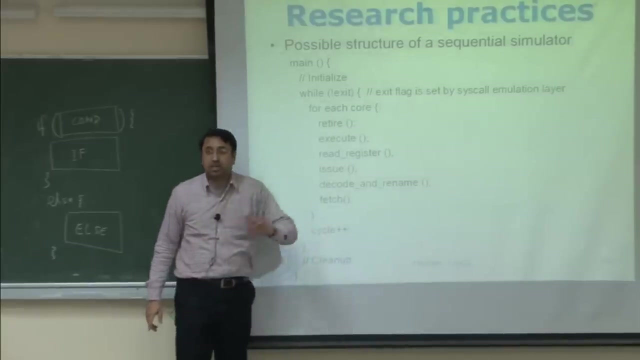 That's not how the pipeline works, So we'll come back to this structure again later. And there are parallel simulators also, So here what happens is that each pipeline stage, these ones, actually run on a different thread of execution. okay, 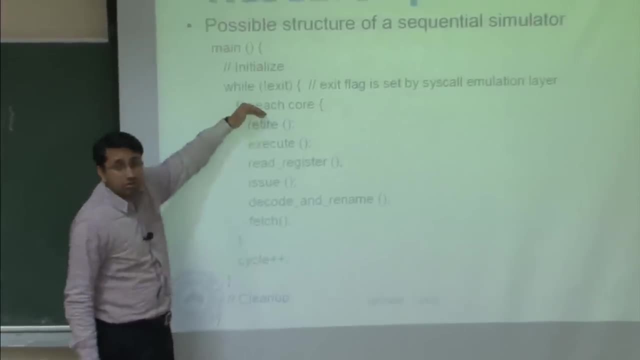 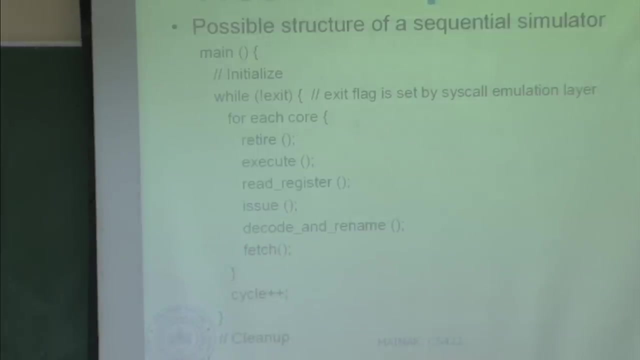 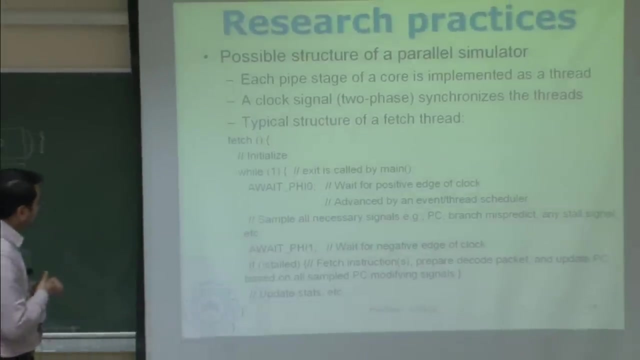 So that's how you get the parallelism. So for each core, each pipeline stage will be assigned to a different processor. okay, and they will simulate that. okay, So a clock signal will synchronize the threads, et cetera, et cetera. 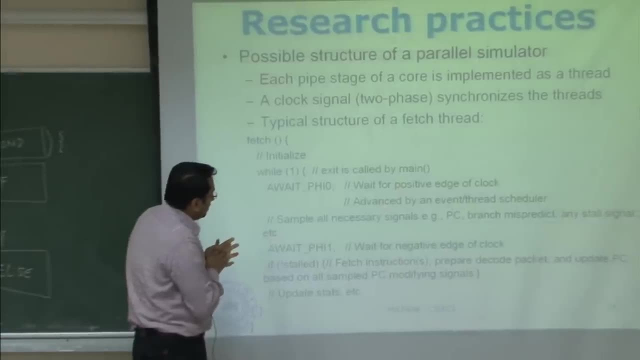 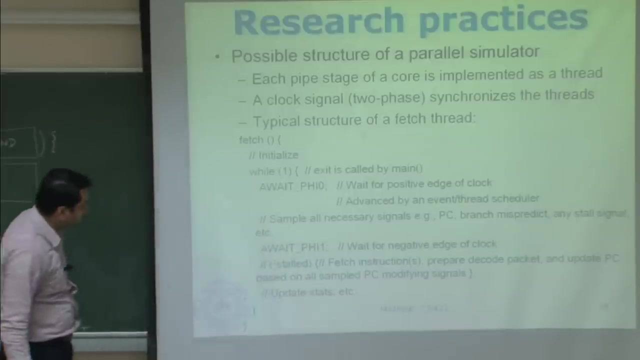 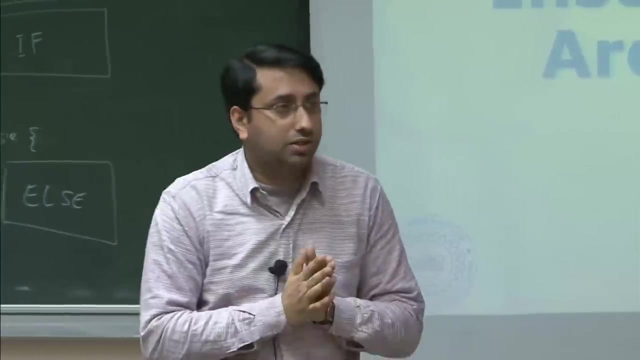 I'm going to skip over these things because there are details which will probably not even follow right now. okay, We'll come back to this later, all right? Okay, so we'll start something new. Any questions before that? on the material: the first lecture. 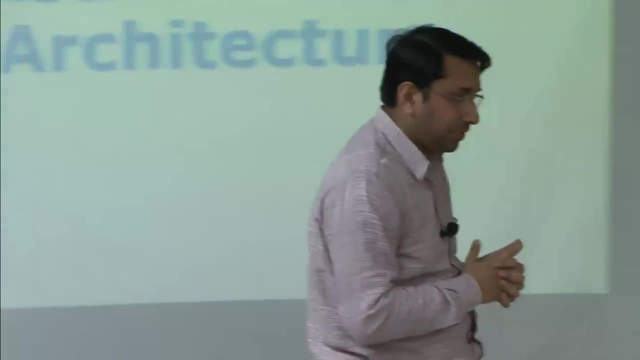 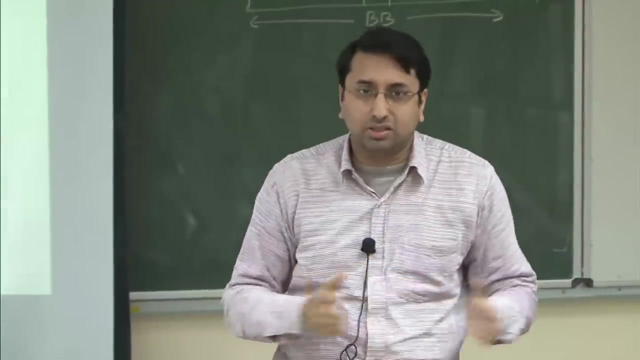 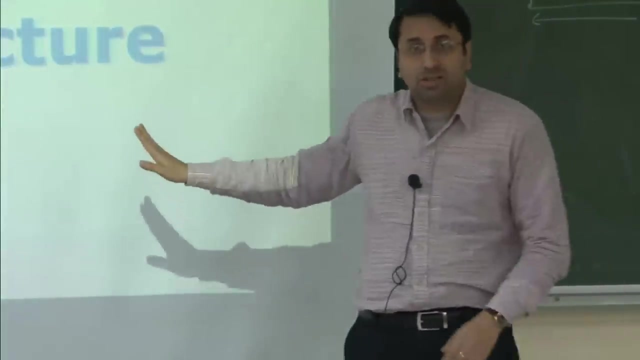 So you should be reading the text, the first chapter that has more than what we have discussed in the class. It talks about the industry trends and all these things which we have skipped over in the interest of time. So this one is again from your book is the first appendix. 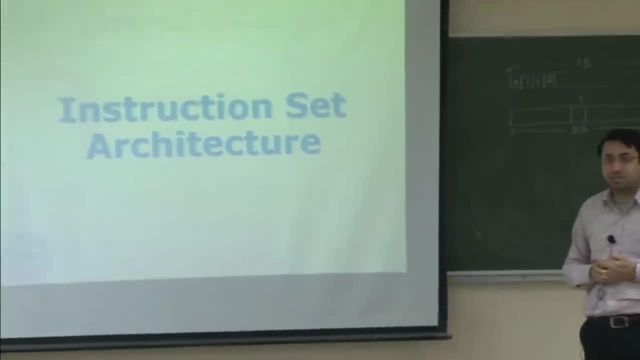 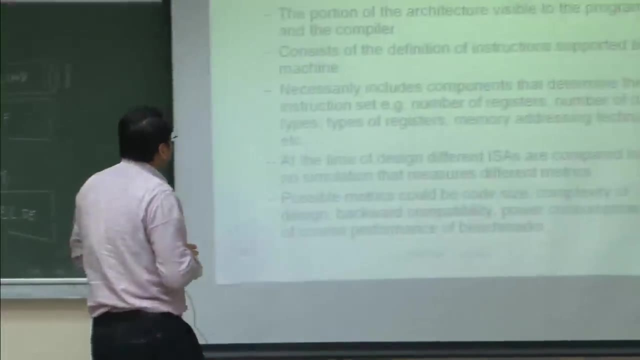 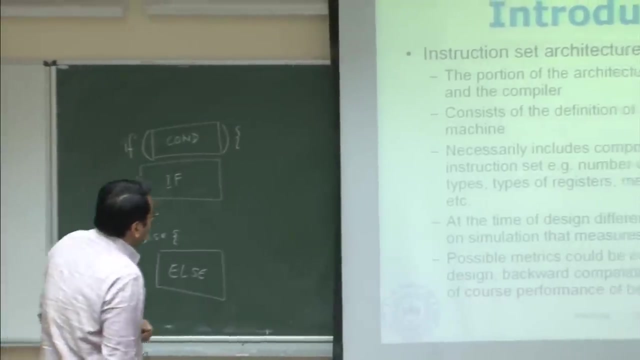 Okay, and it's in the appendix, because the assumption is that you know these things already. So instruction set architecture is the portion of the architecture visible to the programmer and the compiler. okay, And it consists of the definition of instructions supported by the machine. all right, 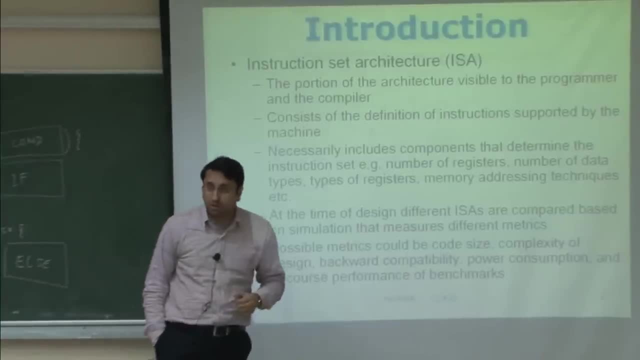 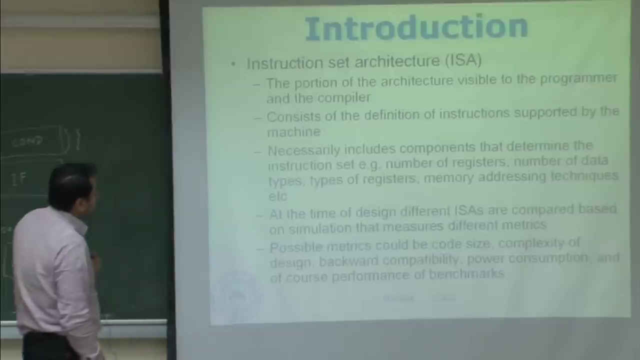 So whenever you talk about a processor reference manual, this is what usually that manual contains. okay, the instruction set, architecture, All right, and it necessarily includes components that determine the instruction set, that is, number of registers, number of data types, types of registers. 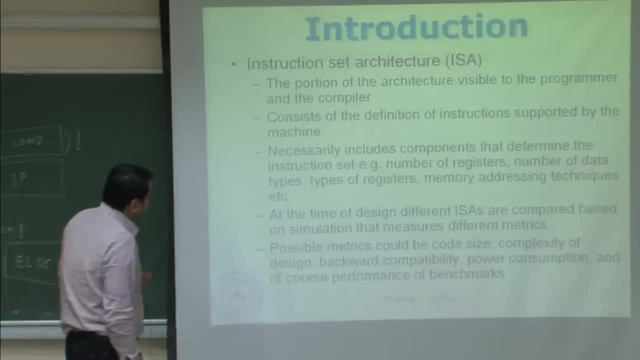 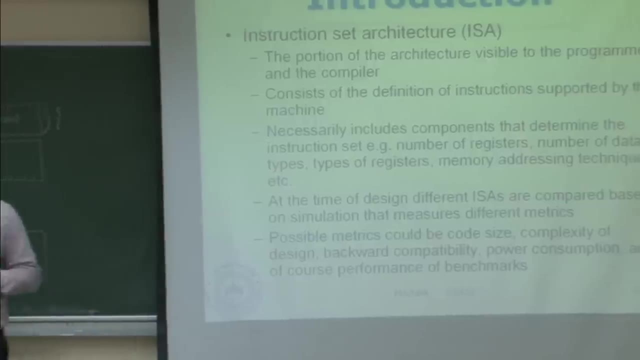 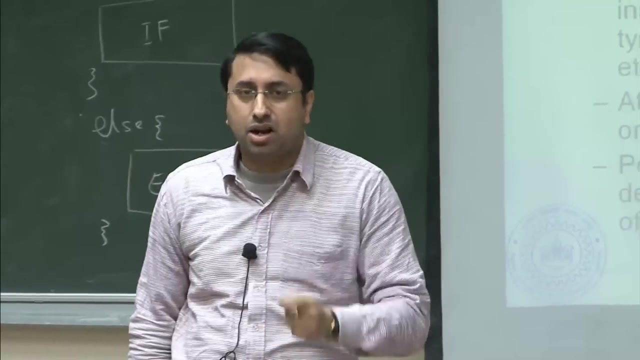 memory, addressing techniques and so forth. okay, At the time of design, different ISAs are compared, based on simulation that measures different metrics. okay, So at every stage of the design you'll find that a simulator is used. So that's integral part of a design cycle. 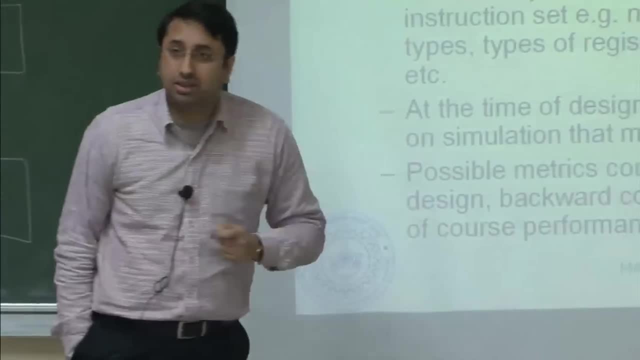 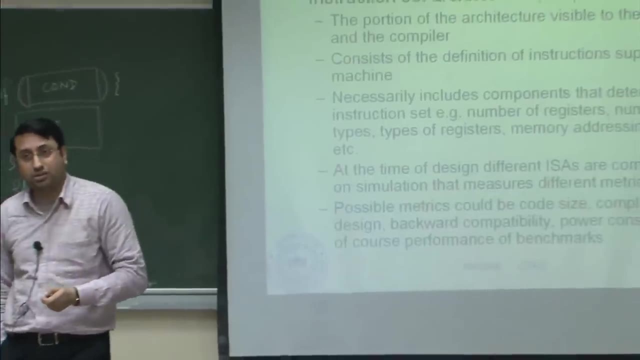 And almost 50 to 60% of your cycle is spent on simulating before you send a design to the factory- Before, because you have to make sure that your design makes sense before you send it to factory, Because manufacturing is a very, very expensive matter. okay, 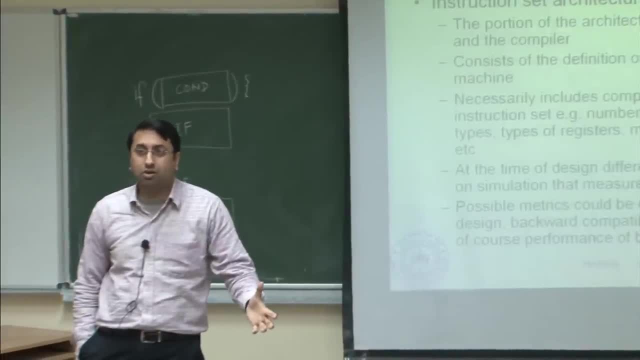 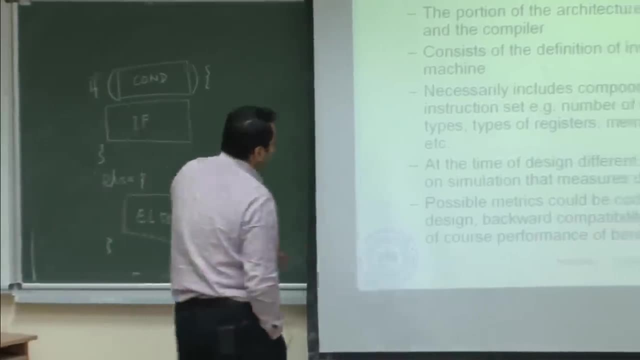 You cannot just send something designed to a factory for fun and say, oh I made a mistake, That you know that costs your company a billion dollars, So it cannot be done. You spend a lot of time simulating to make sure that what you're proposing makes sense. 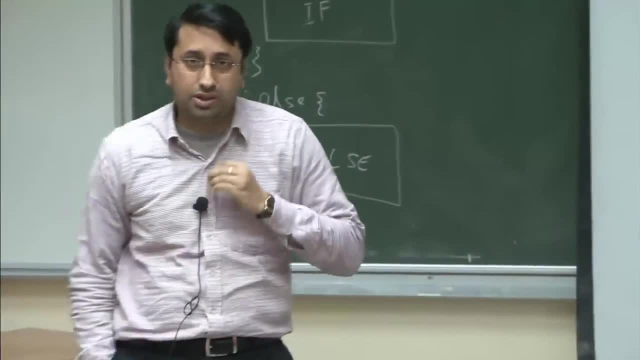 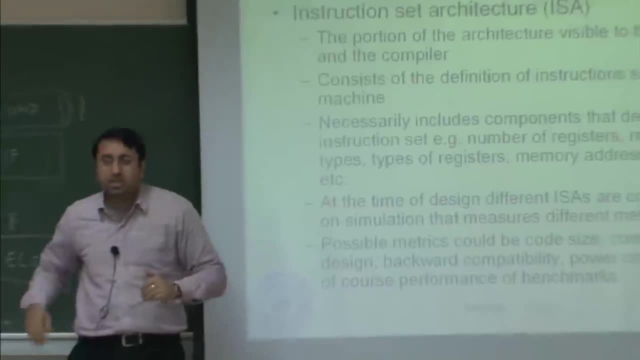 what you're proposing is correct. what you're proposing is not correct. What you're proposing probably brings performance, okay. So at this stage we are talking about instruction, set architectures And, of course, we'll see that there are many options. 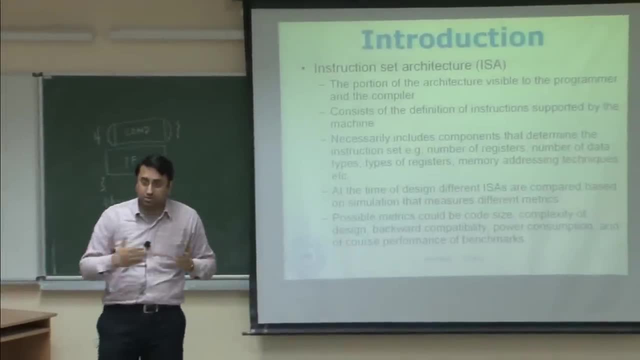 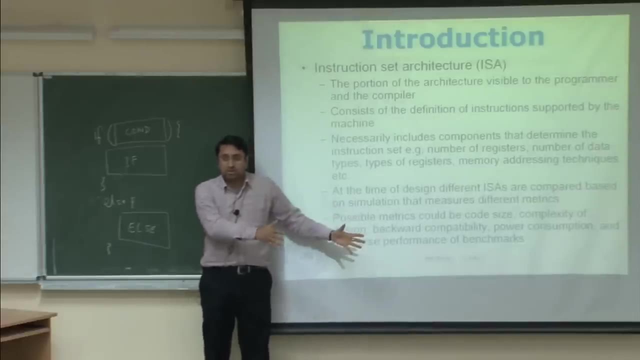 We have already discussed a couple of options in the last lecture regarding branches. okay, right, So you have to figure out which way to go, And the only way to figure that out is to use simulation. You take your benchmark applications, compile them for multiple different ISAs. 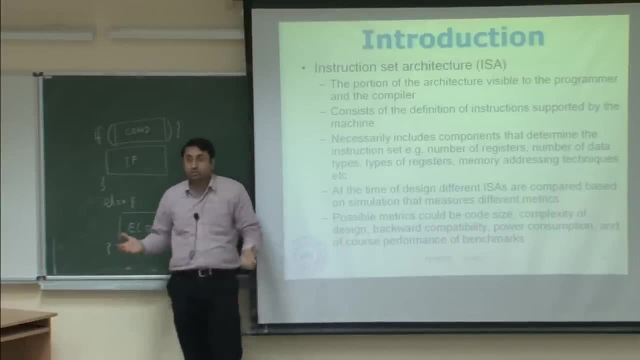 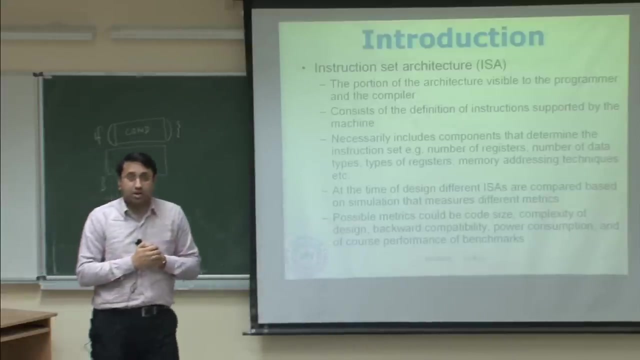 run each of the executable on the simulator and find out which one runs faster. okay, It's not just running faster, it also depends on how complicated your design is. all right, So possible metrics could be code size, that is, when you compile a program for a particular. 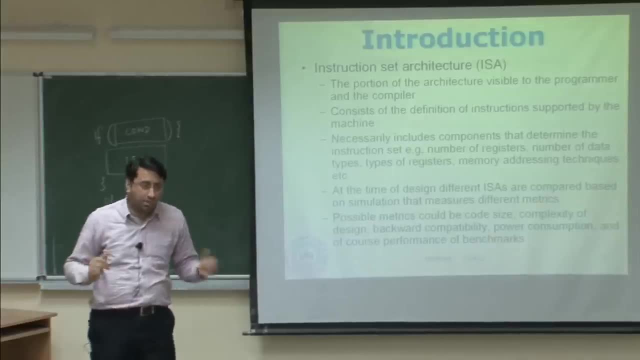 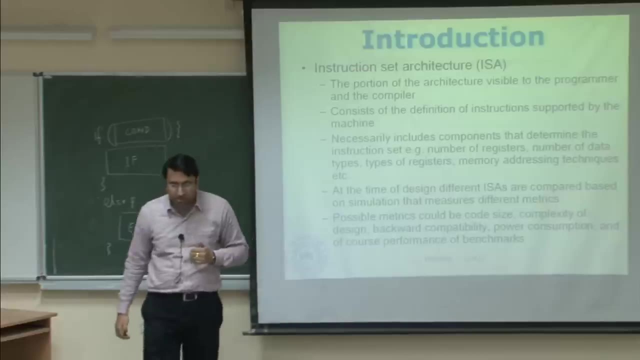 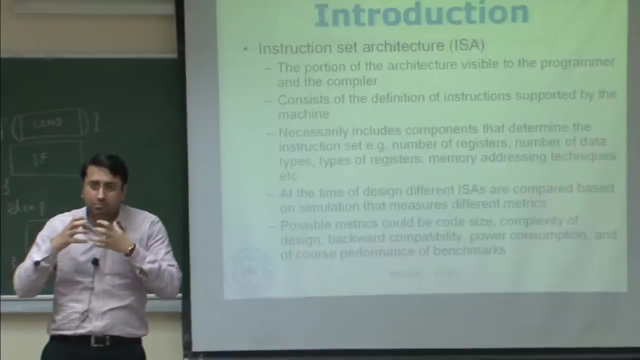 ISA. how big is my binary? That's a very important thing. Complexity of the design. that is, if I have an instruction set, architecture that is very compact, but each instruction is overly complicated, So it gives you extreme complexity, Okay. If I have an extremely compact binary, very small, okay. but my design is lousy, gigantic. 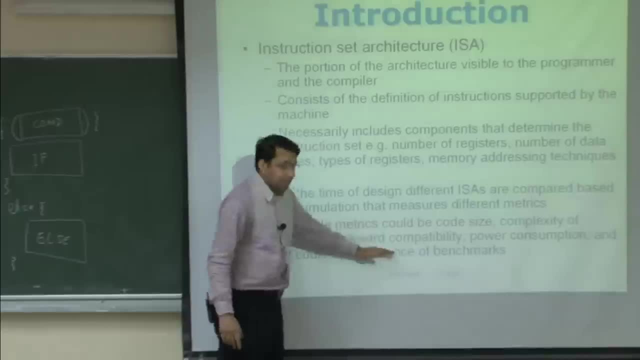 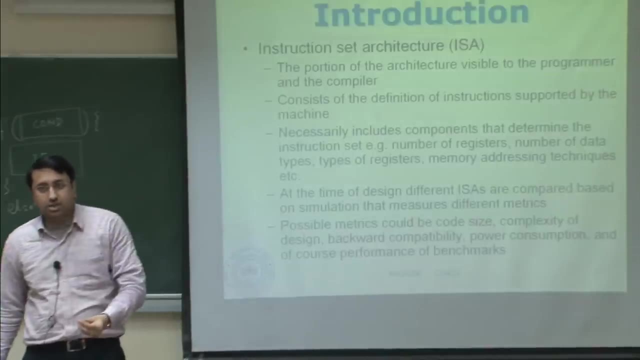 and complicated. okay, not done. Backward compatibility: that's very important for business. If you are in the industry, you are designing a new instruction set architecture. it is important that users that are using your machine's previous versions should be able to continue to run. 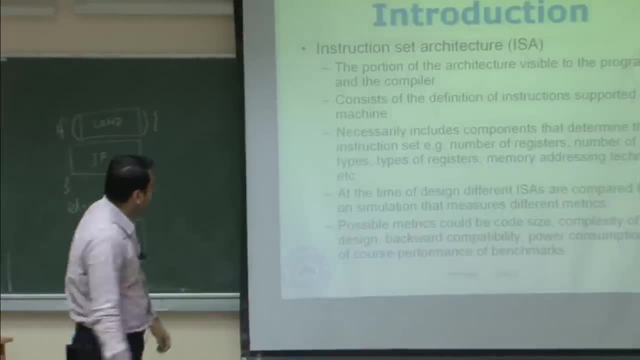 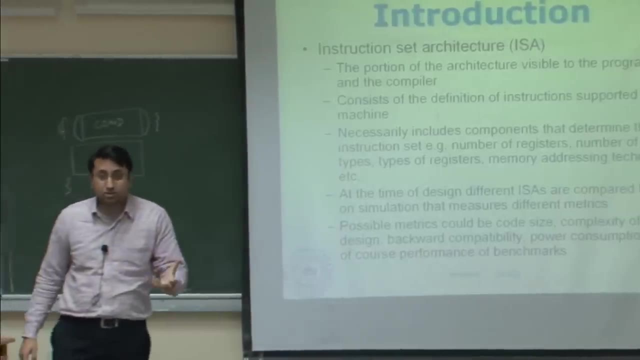 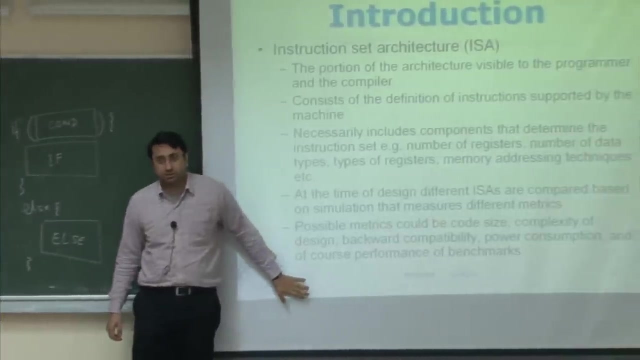 those binaries on the new machine. okay. so that's backward compatibility, Okay. Power consumption: how much electric bill my new ISA would actually make my user pay? that's also another important point. And of course, performance of the benchmarks: okay. 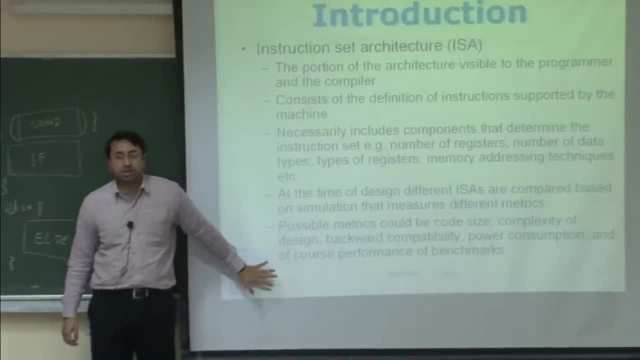 So there are various things that you have to balance when choosing an instruction set, architecture, And this is a very important decision because remember that this is the only thing that will ultimately get exposed to the compiler, designer and programmer. okay, So if you make a gross mistake here, 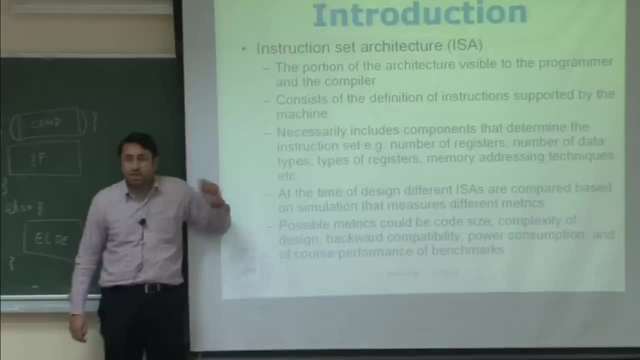 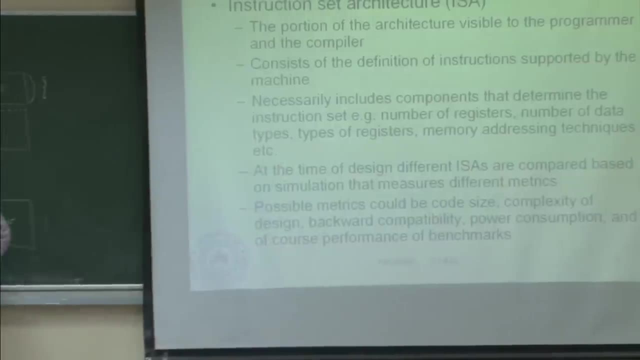 Okay, Okay, And if you make a huge mistake here, for however smart a design you have inside, nothing matters. Okay, This very important in set architecture, Like recall that you know string copy instruction that we discussed last time. Okay, 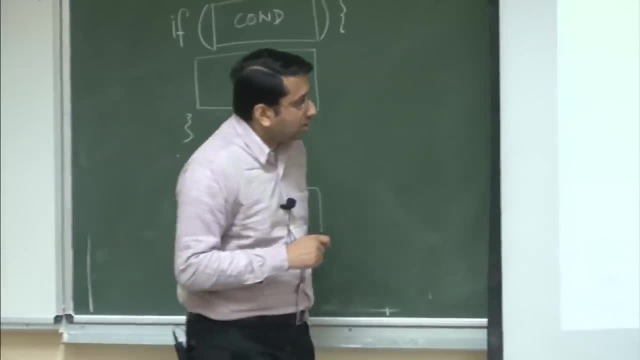 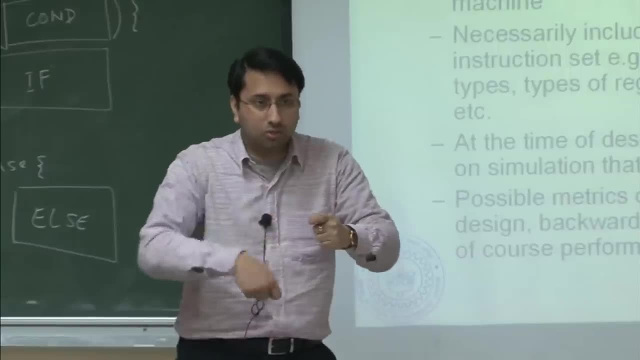 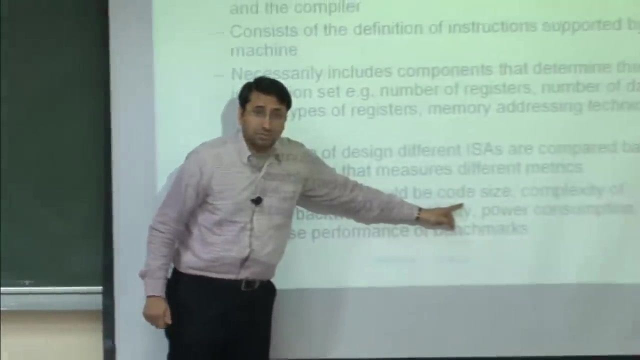 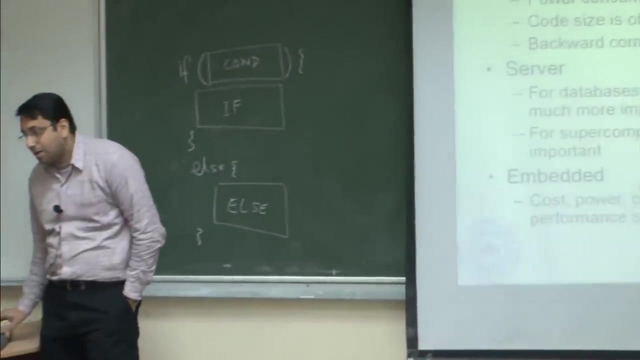 It would require a very complicated hardware, Whereas offering just one instruction for byte copy and allowing the programmer to actually orchestrate the string copy by running a loop with byte copy instructions Okay would of course explore your code size a little bit, but your design is going to be much simpler. 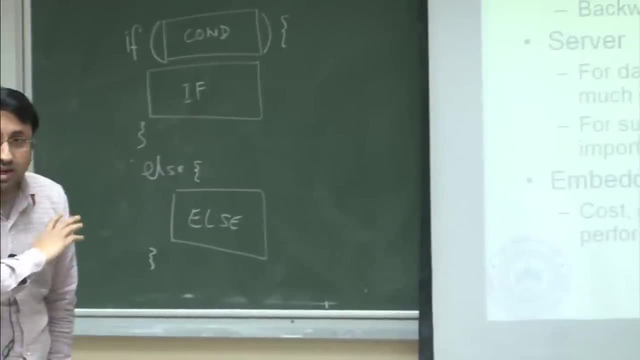 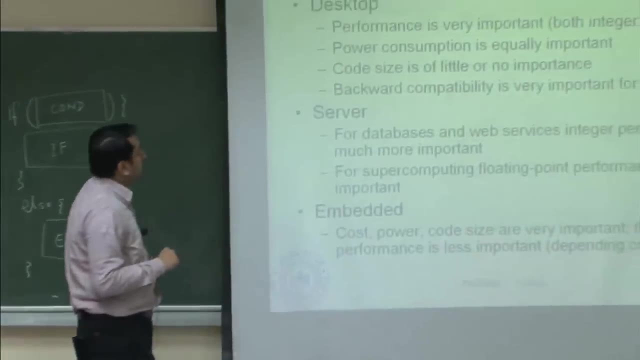 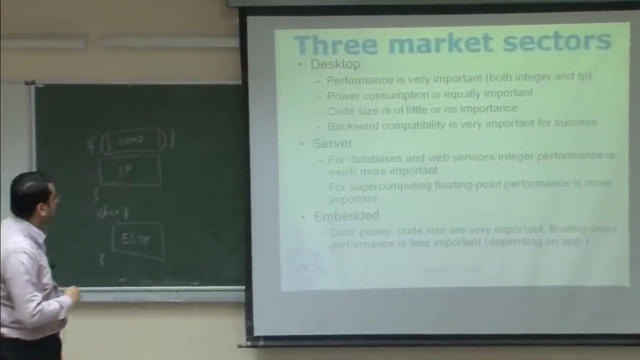 So, just to remind you, we have to keep in mind that there are three market sectors which we have to cater to. so in the desktop segment, performance is very important. so that is all that a user actually cares about in the desktop part, both integer and floating point. 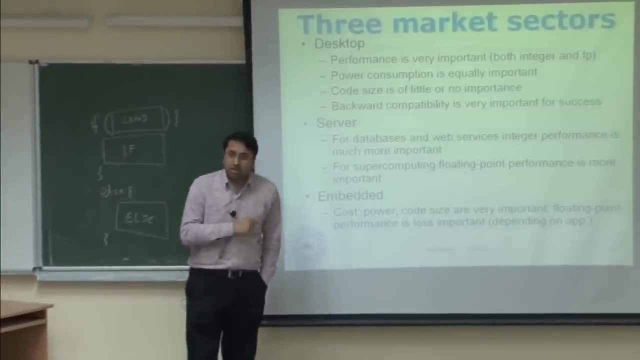 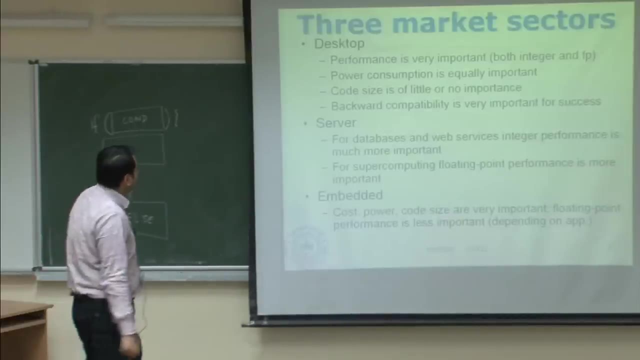 performance. Power consumption is equally important. I install a desktop in my home. my electric will cannot be doubled. then of course, that is a no go. code size is of little or no importance. I can buy, you know, DRAM cards. I can install them. code size is not that much of importance. 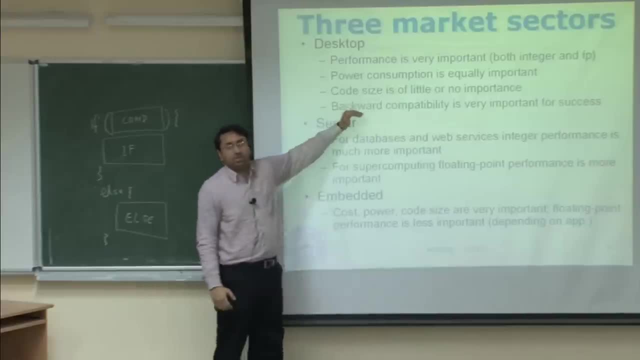 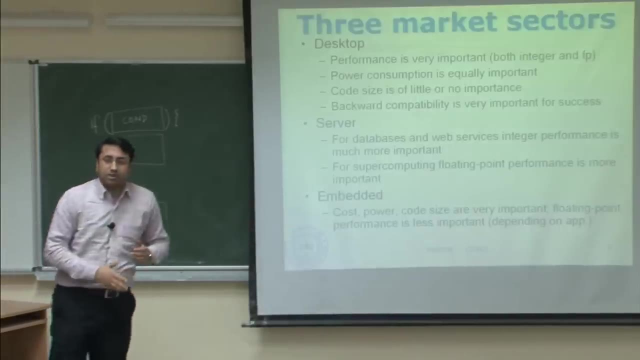 and also the reason is that we do not really run very complicated codes on a desktop. sorry, code size is not that large. that is why the code size is not that large. Backward compatibility is very important for services. okay, because I might have bought. 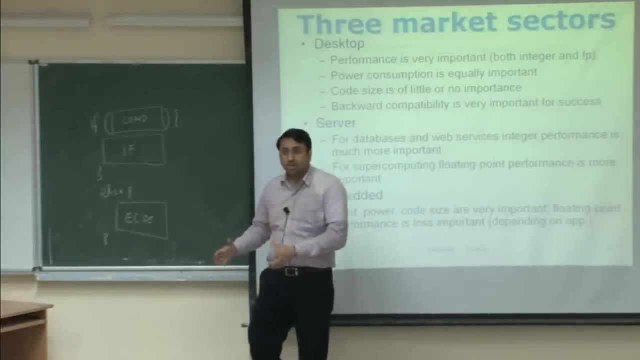 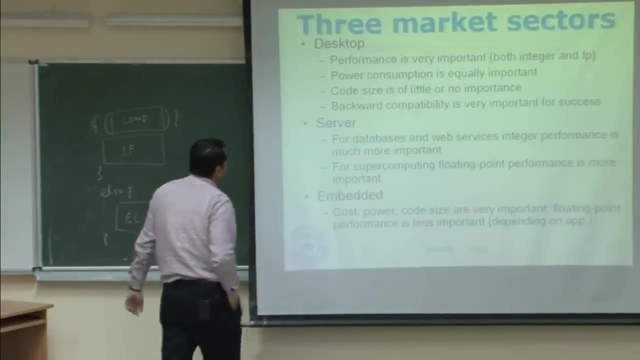 certain software for my previous computer. I get a new computer, those software should continue to run. okay, I do not have to get new licenses. that is a very costly matter In the server market for databases and web services. integer performance is much more. 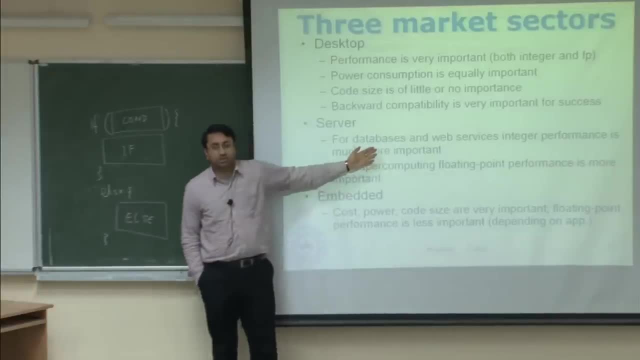 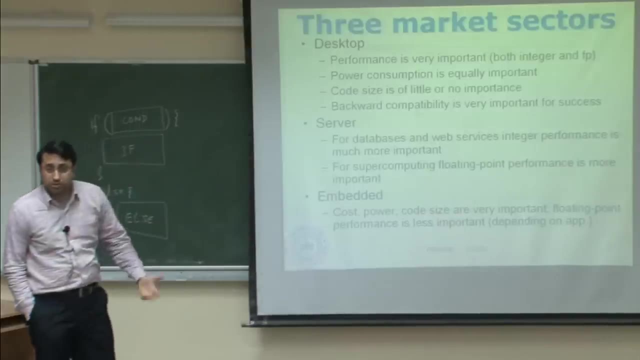 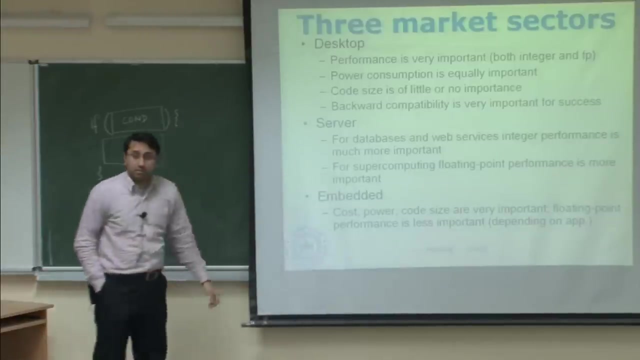 important. In fact, there will be very little floating point computation in such applications. okay For super computing. on the other hand, floating point performance is more important In the embedded market. cost power, code size. all of these are very important because 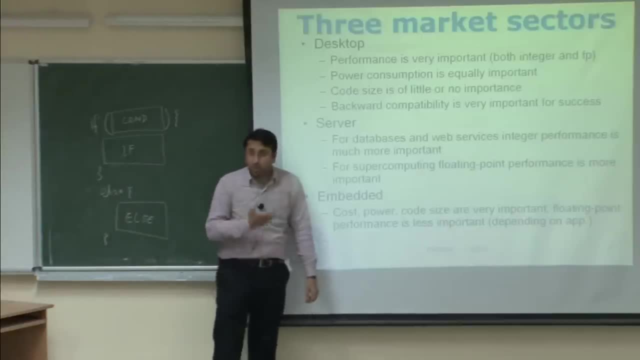 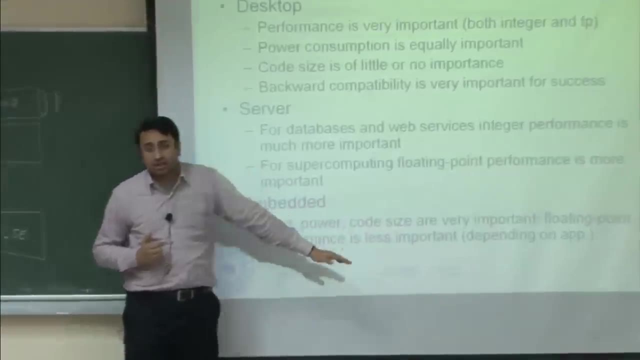 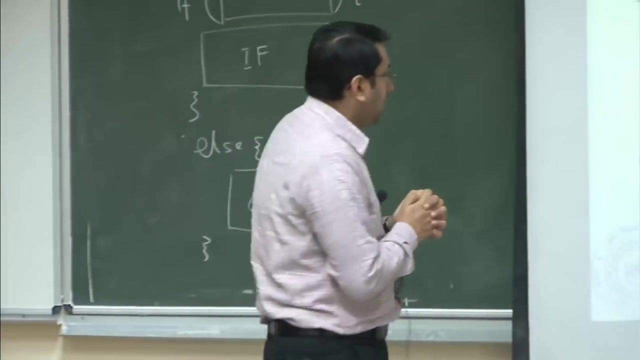 here we are talking about things like handheld, your smartphones and all where your memory on board is very small, okay, So you cannot have an ISA that compiles into a large binder. That is not done. you need to have smart, compact binaries. you need to have low power. 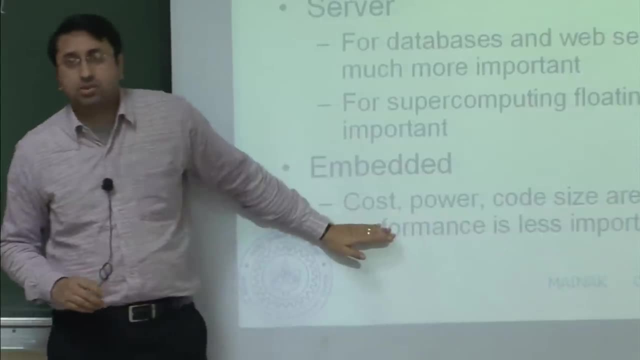 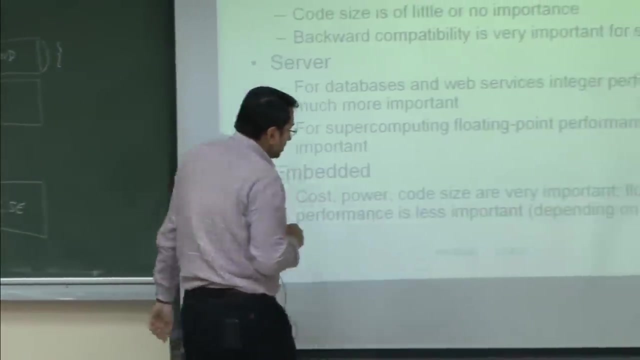 so that my battery lasts long, okay, and of course, the design should be low cost, okay. Floating point performance is less important, depending on, of course, the application If you are, if you are running, for example, various image processing applications on your 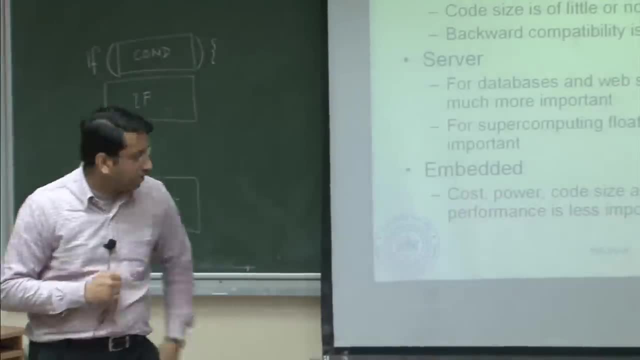 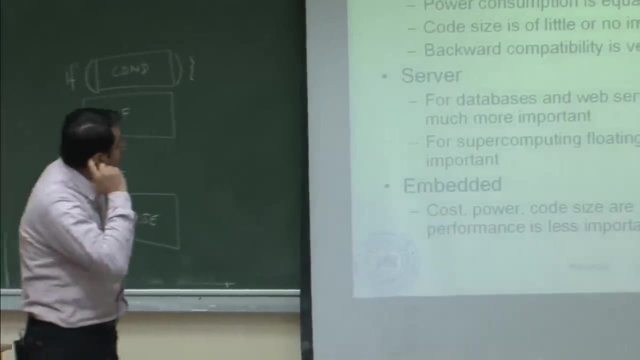 handle. of course, floating point performance will be important in those cases. So keep this in mind, Thank you, Thank you. So keep this in mind when designing your application. sorry, instruction set architecture, because when you design a processor, usually what happens today is that you would be keeping. 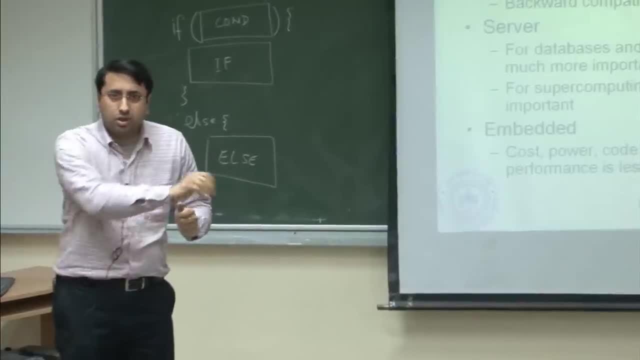 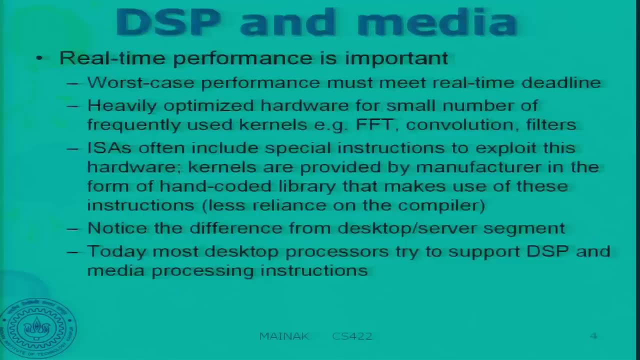 your instruction set more or less unchanged and you will be catering to all these three markets. okay, So you have to, you have to have a common ground for all of these. And of course, there is digital signal processors and the media applications, where real time 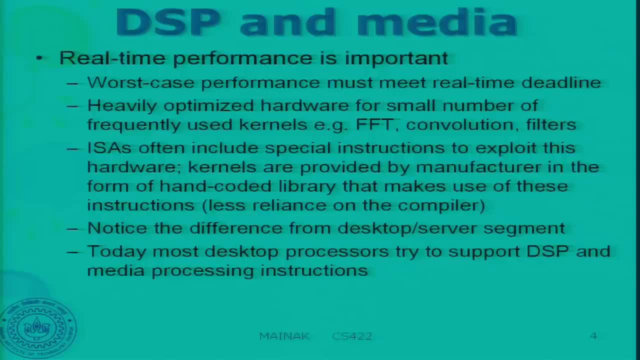 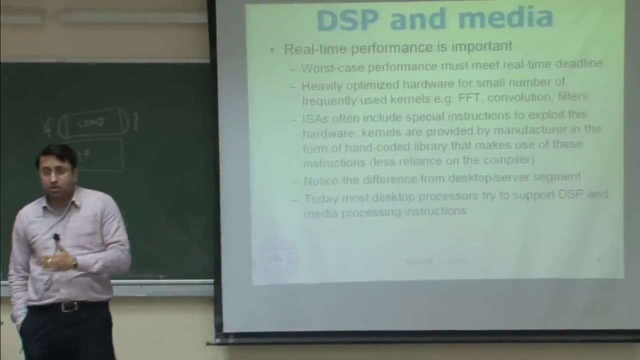 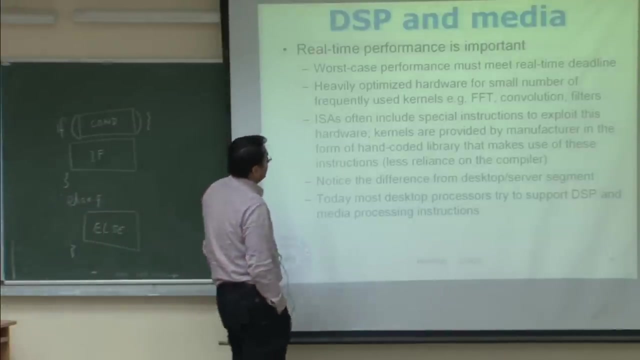 performance is important. Worst case performance must meet real time deadline. For example, if you are running a codec, it should be real time. okay, it cannot. it should not take longer, otherwise the user will get annoyed. Heavily optimized hardware for small number of frequently used kernels like fast Fourier. 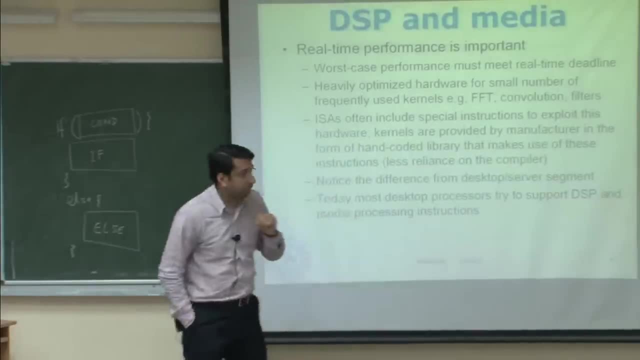 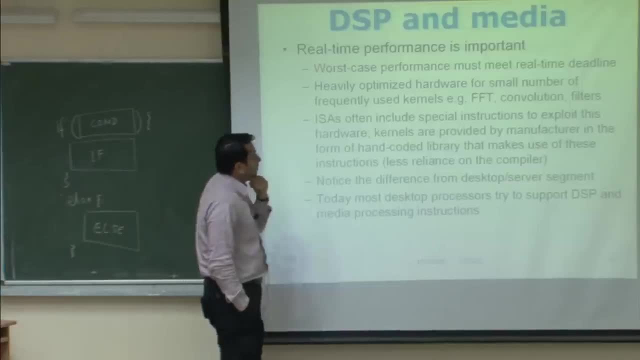 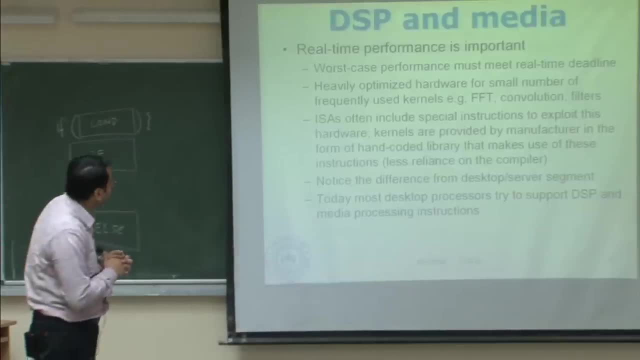 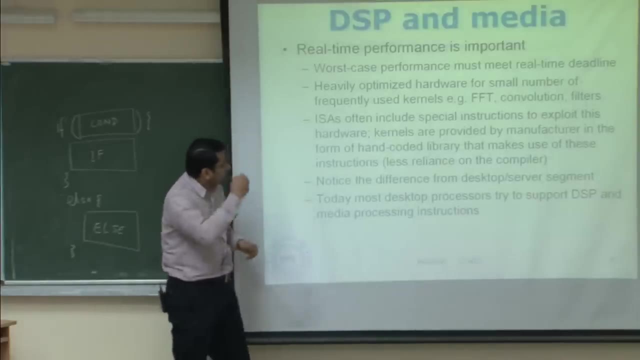 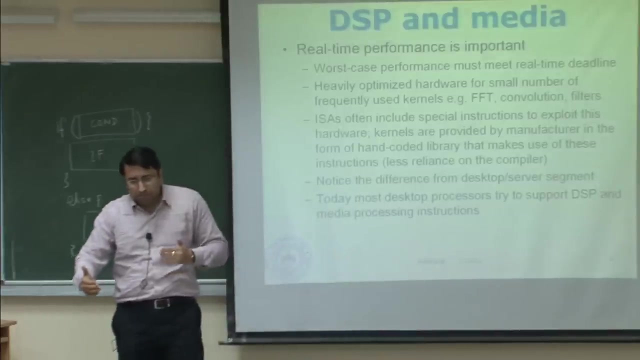 So just one instruction would actually do an FFT for you. okay, Kernels are provided by manufacturer in the form of hand coded library that makes use of these instructions. So here there is less reliance on compilers, but it is improving. The simple reason is that, given a piece of code, compiler will have very hard time figuring. 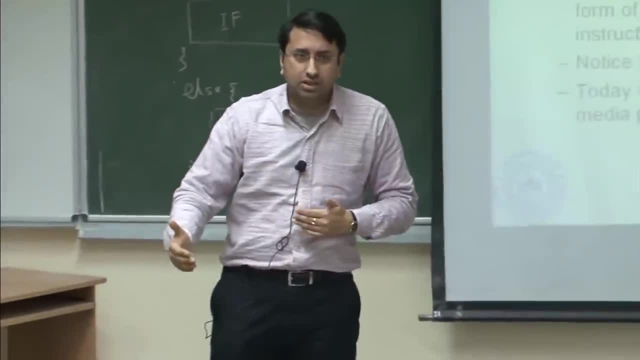 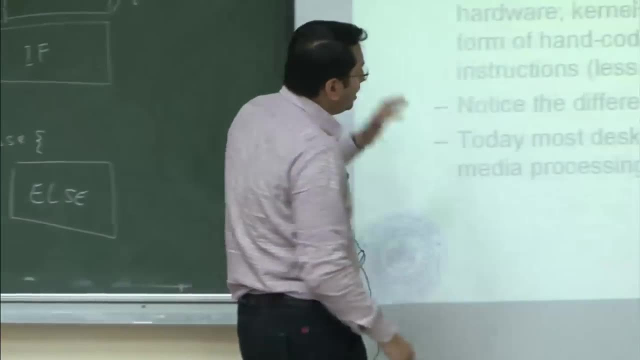 out that, oh, this is an FFT. that is very difficult actually. It is an unstructured piece of code that somebody has written. How does the compiler figure out that it is an FFT? So that is why you know the. the vendors already provide the, the libraries for you. 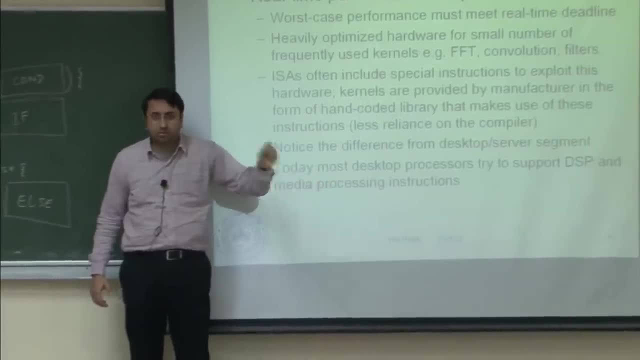 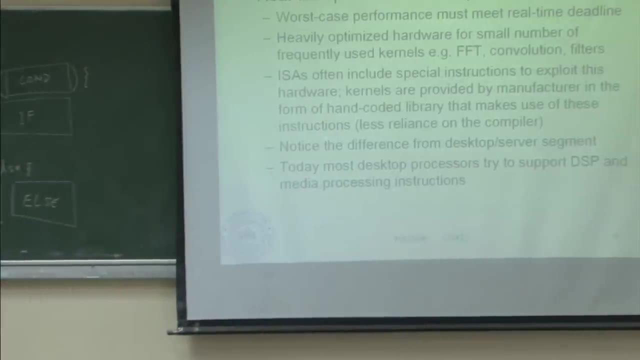 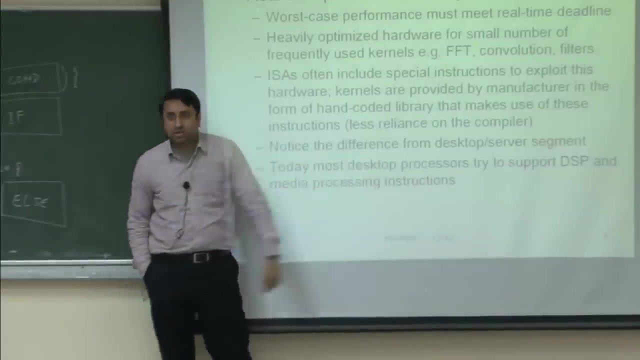 You just have to invoke that library function, which is actually already been compiled, to use this particular instruction FFT module. So this is a big difference from your desktop server segment where we rely very much on the compiler- okay, which seldom do hand coded assembly programming. 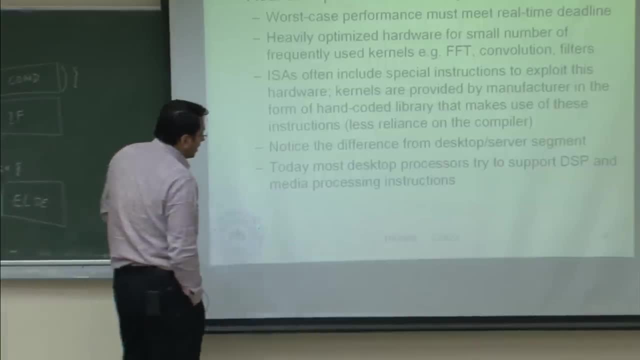 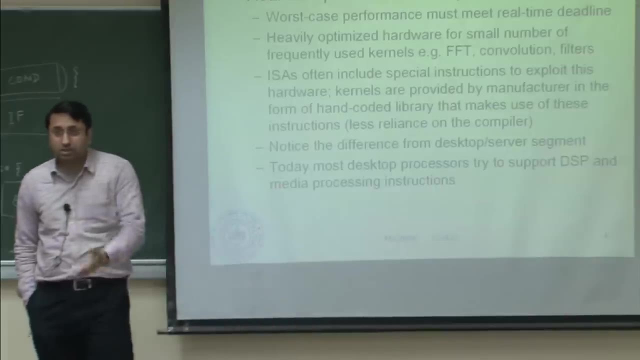 And today most desktop processors try to support DSP and media processing instructions. In fact, this has become an integral part of your processors today, like you must be knowing about your MMX and all these things right multimedia extensions in your Intel processors. 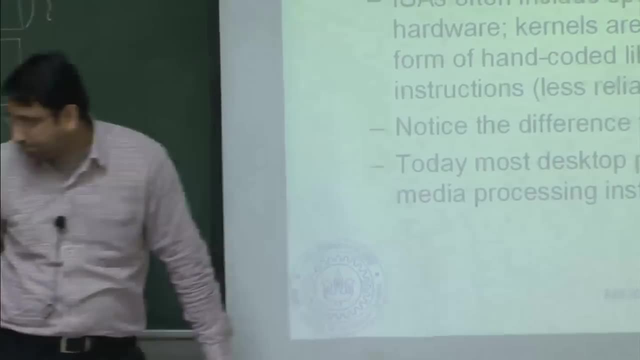 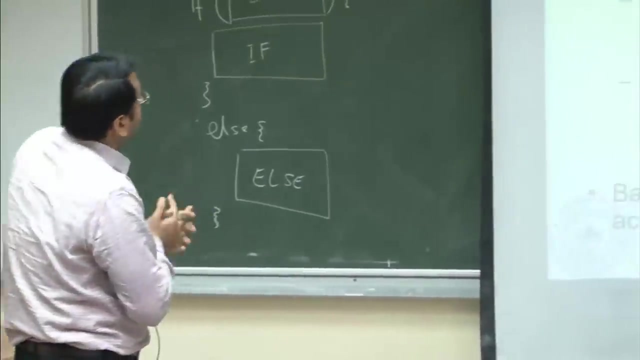 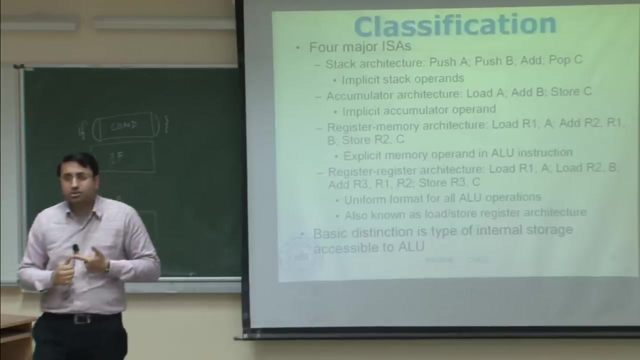 So, so they, they all have these instructions, So we will start with a classification of the instruction set architectures: Stack architecture. Stack architecture essentially is an architecture that has arithmetic operations and the other two operations to operate on the stack, that is, push and pop. all right, 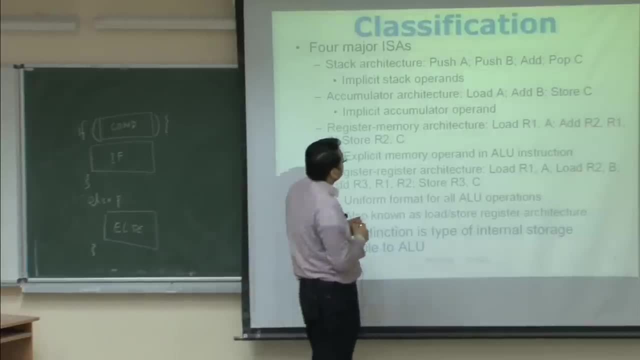 So. so if you look at this sequence of instructions here- push A, push B, add and pop C- what it does is that it first pushes. so essentially I want to do an add operation. okay, I want to add A and B, store the result in C. That gets compiled into data. 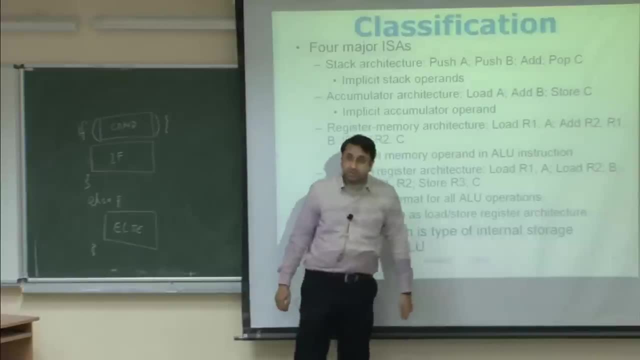 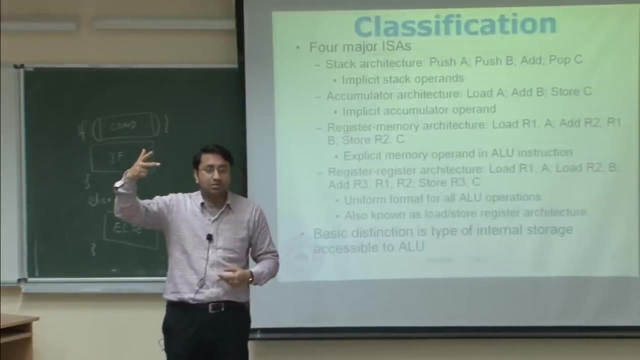 So I push my first operand, I push my second operand And then I do add, And the add instruction has two implicit arguments. What are they? The top of the top two elements of the stack, all right, And the result goes on the top of the stack. 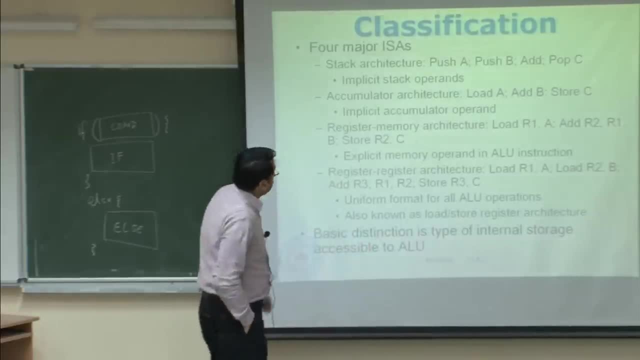 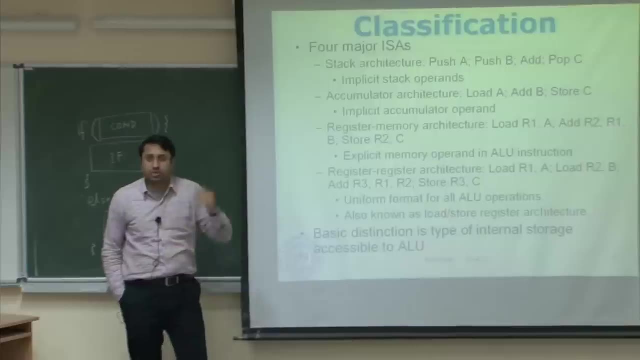 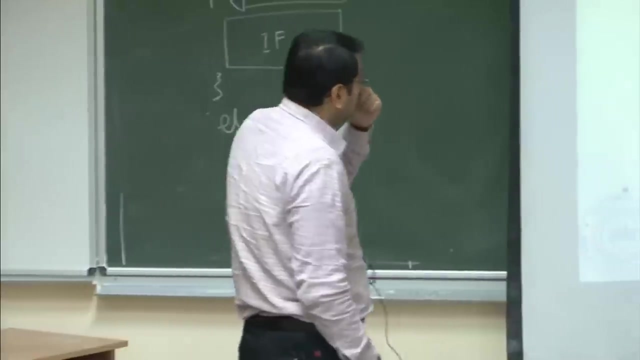 Then I pop, it goes back to C. okay, all right, Is that clear to everybody? The stack architecture: Okay, So it will only have push, pop and arithmetic operations with implicit arguments. The next one is accumulated architecture: Okay, Where what you do is you have implicit accumulated operands. okay. 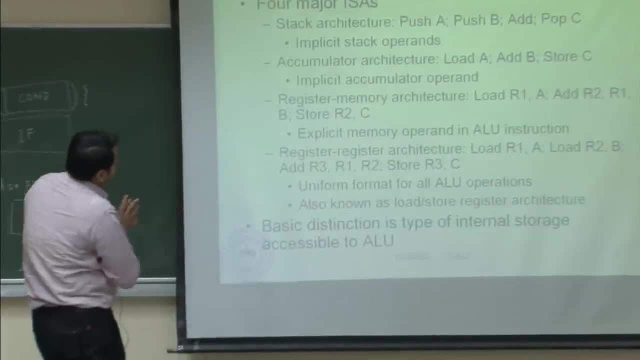 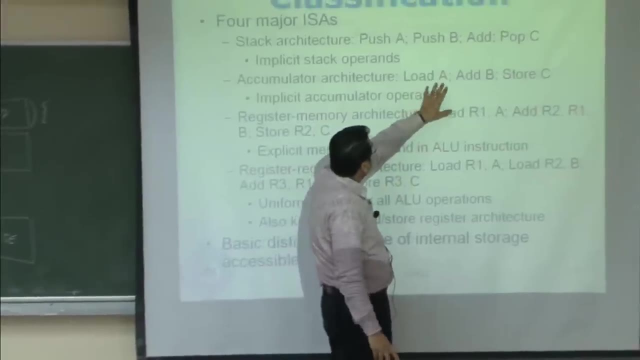 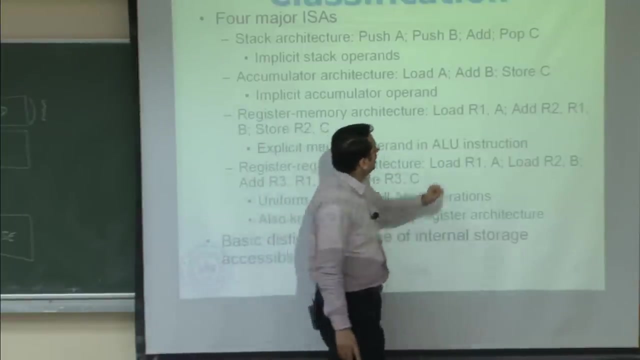 So the same operation, C equal to A plus B gets compiled into that. So you first do load A, okay, So that brings your, your, your, your, your operand A into an accumulator. all right, Okay, Then you do add B, where one operand comes from memory, where B is stored. 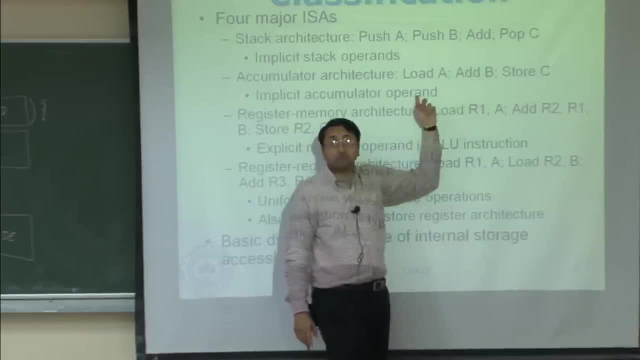 Okay, All right. Then you do add B. where B is stored, The other operand comes from the accumulator, which is A, all right, And the result remains in the accumulator, so that when you finally say store C, the operand is picked up from the accumulator and sent it to C and sent to C. 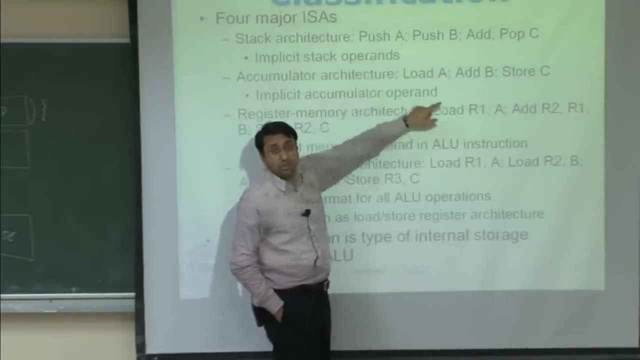 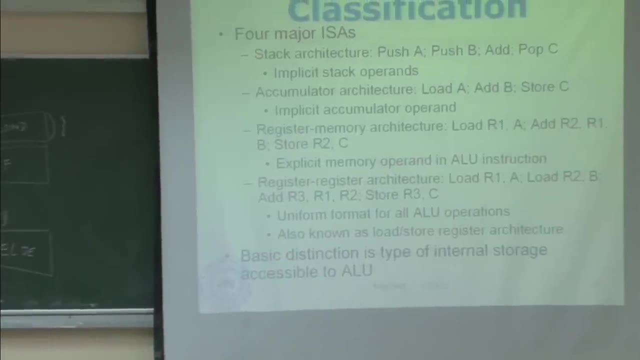 So here the the operand was always the top of the stack, Here the operand is always the accumulator. okay, one of the implicit operands. The third one is register memory architecture, where your, your, your, your, your, your, your. 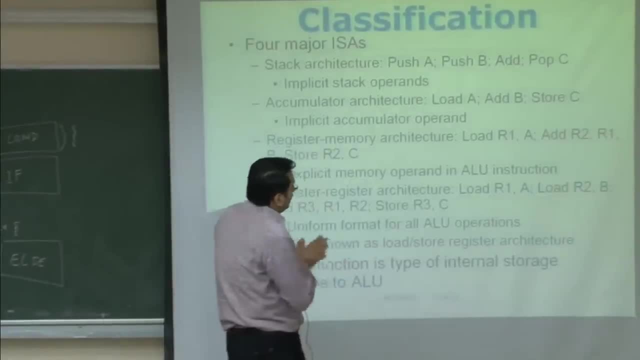 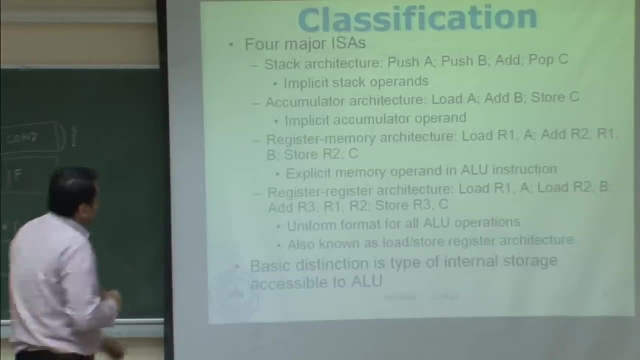 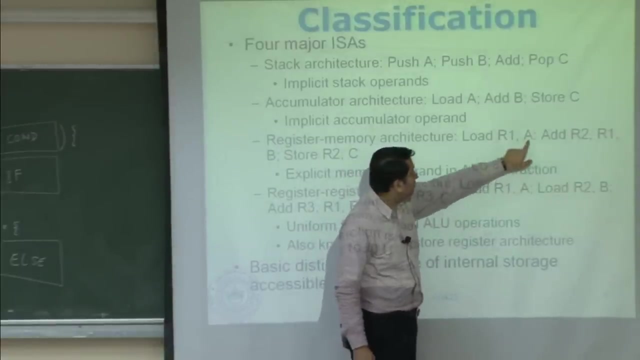 that your, your, your operations can either take a register or a memory or both, or a memory operand or both. So load r 1 comma a. you load the value of variable a into register r 1.. So this is a memory address, this is a register. all right, then you say add r 2. 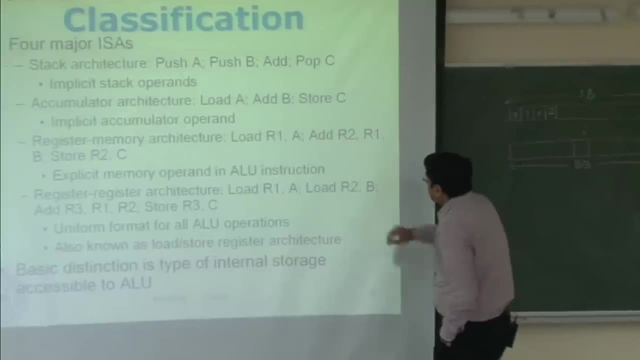 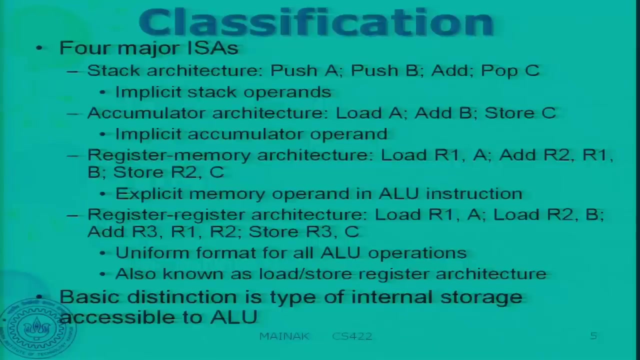 r 1 comma b. So always we write the destination first and the two sources next. So it is essentially adding r 1 with the memory operand b and putting the result in r 2.. So these are combined. register memory operation takes one register. of argument takes one memory. 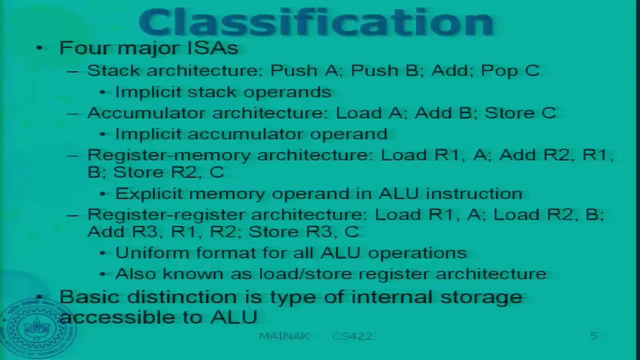 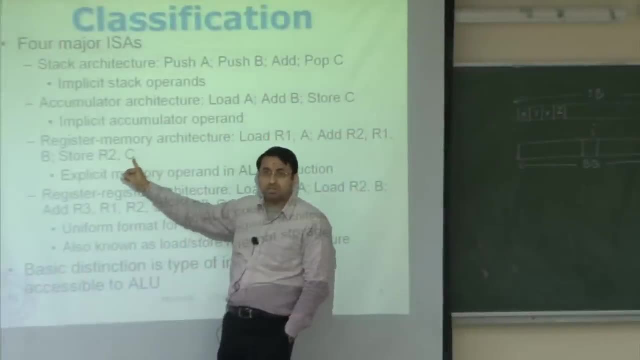 argument and pulls the result in the register. And then finally, I say store r 2, comma c, which picks up the source from r 2, pulls the result in the register But back to a memory location, c. all right, So here we have explicit memory operand in. 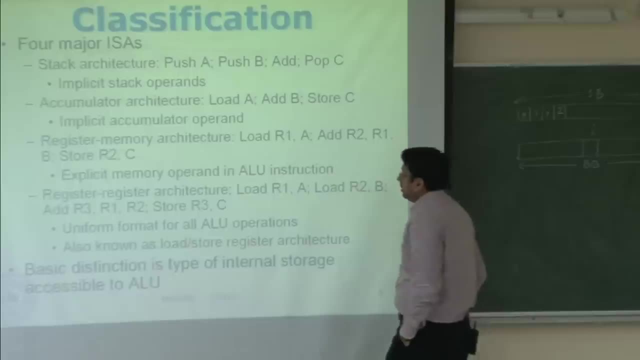 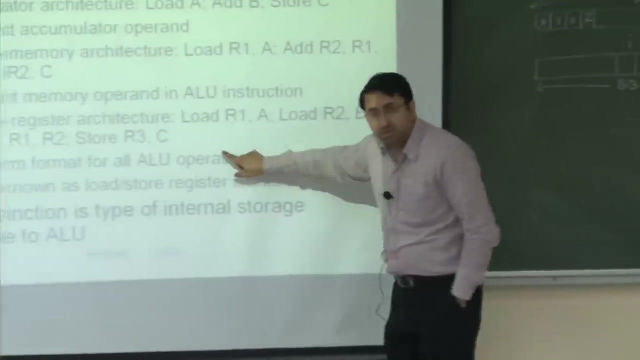 ALU instruction. And finally, register register architecture, where the only difference from this with this is that no ALU operation can be done on memory in this particular architecture- register register architecture. Otherwise it is exactly same as this. So here you also. 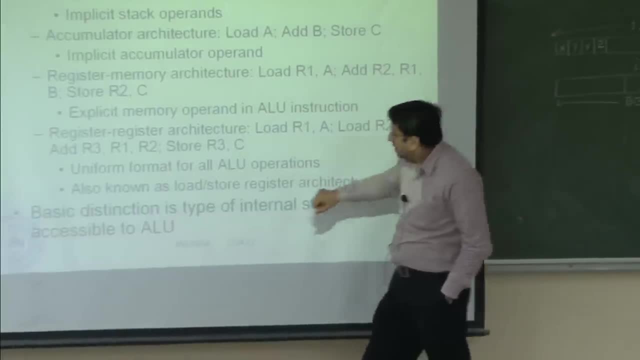 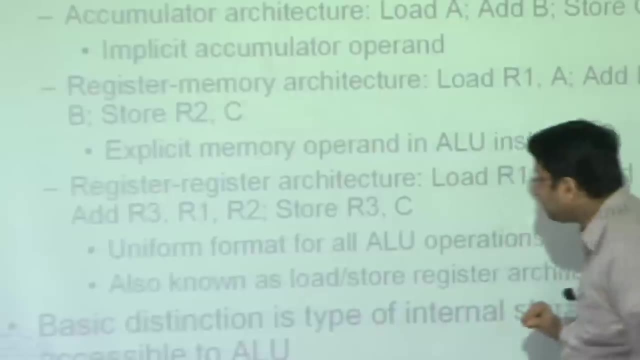 have load r 1 comma a, Then load r 2 comma b, and then you have add r 3 r 1 r 2.. So this add operation here cannot take any memory operand, it all has to be register. and then you say store r 3 comma c. The result: 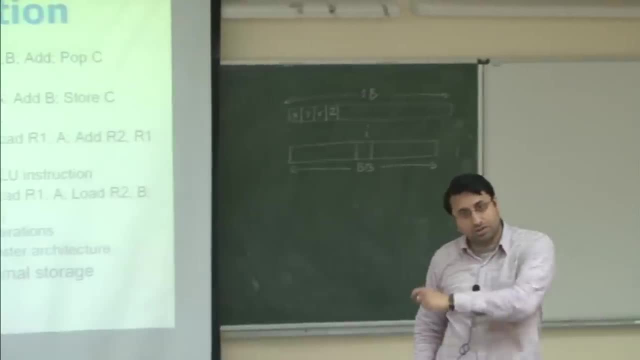 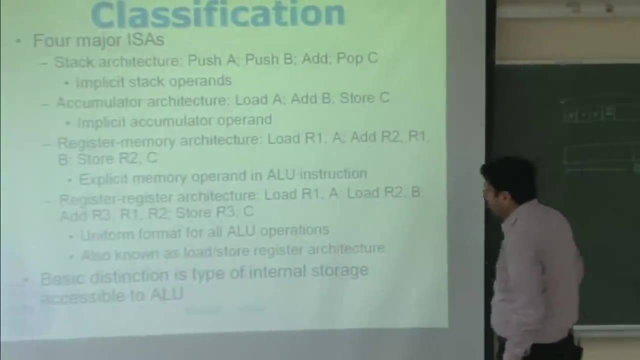 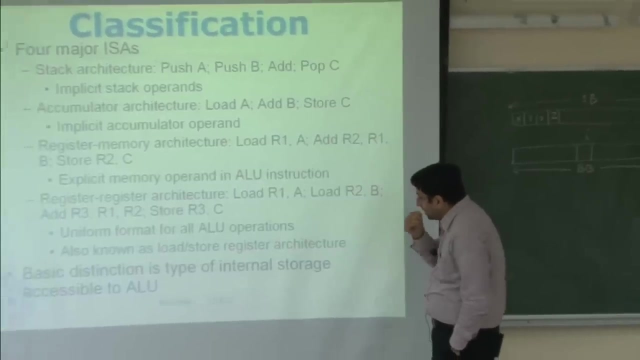 is always stored in register and then you have to pick it up from there with the store store operation and yeah. So here you have a uniform format for all ALU operations, also known as load store register architecture. What type of internal storage accessible to the ALU? If you look at all these four, this: 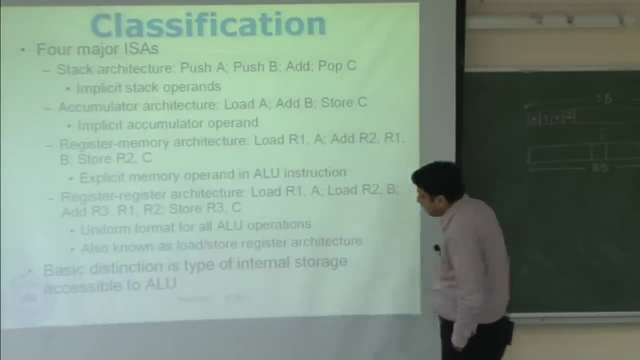 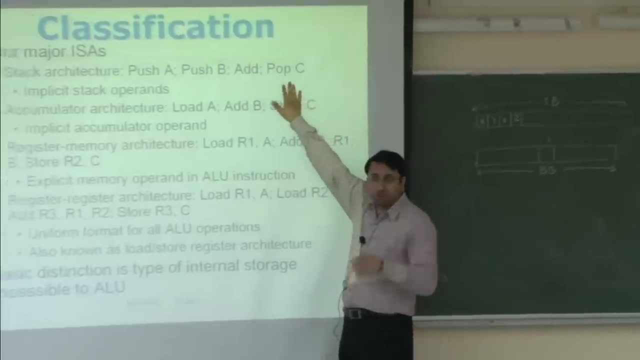 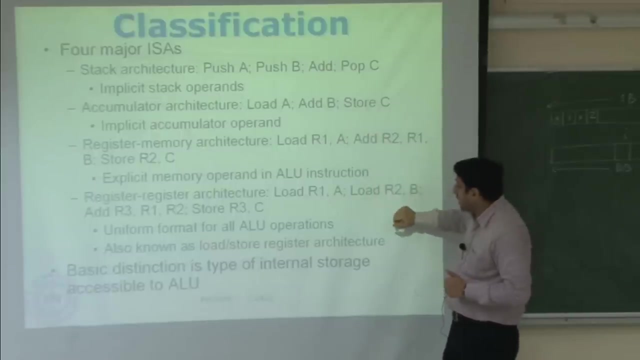 is really the basic thing that differs. ok, What? what does the ALU access when it does an operation? Here it accesses the stack top, the top two or the top most. Here it accesses the, the accumulator. here it accesses the register and the memory, and here it accesses 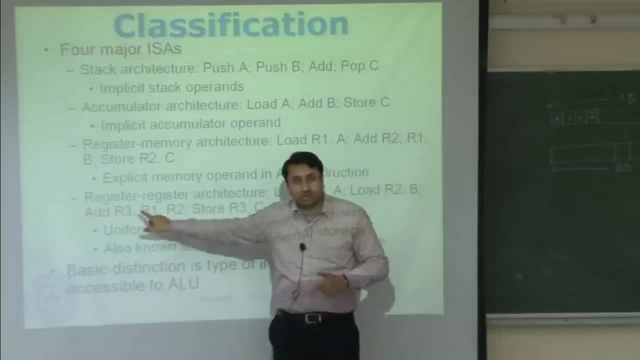 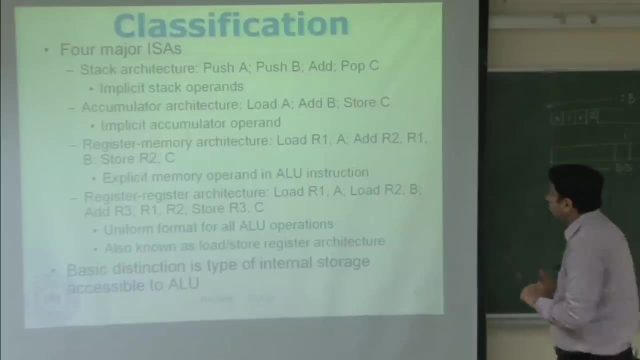 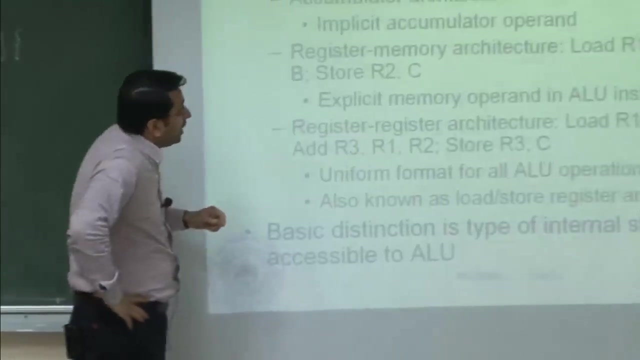 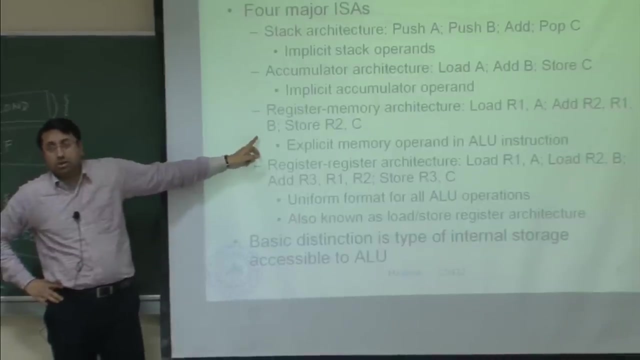 only registers. all right, And that is where the name comes. What type of storage the ALU has access. Any question on this classification? All right, So today your X86-ISA belongs to this category: register memory. it has a lot of register memory operations. will look at something called a risk architecture. that 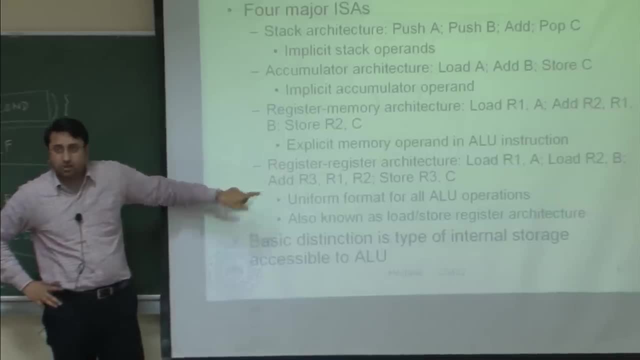 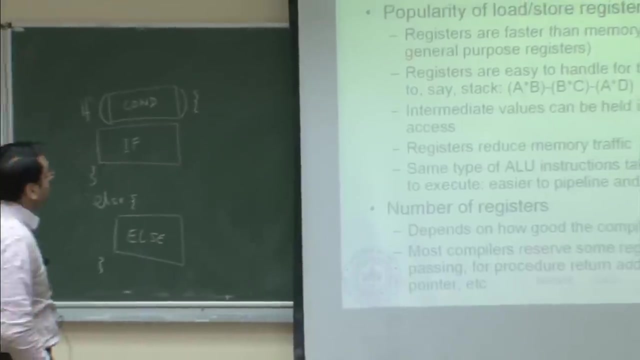 only supports this register register. ok, And to contrast with that, we talk about sysch. so which is your x86, so we will come to that soon. that distinction, So the load store register ISA or the register register ISA has become very popular and the simple reason is that registers are faster than memory so you can do very fast ALU operations and, as a result, there is a push to provide more general purpose registers so that I can do more ALU operations on registers. registers are easy to handle for the compiler compared 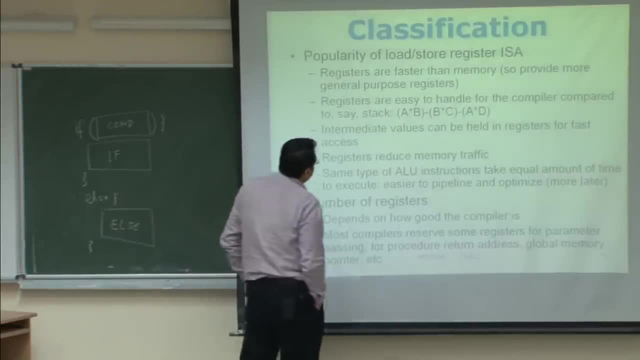 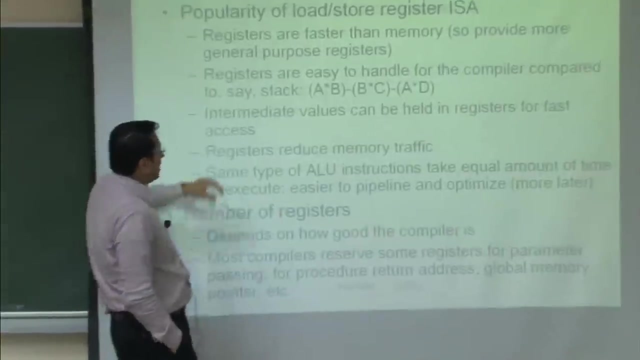 to say stack, for example. so you should go back home and try to generate stack code for this particular of this particular calculation. try to see what kind of code you get. okay, Intermediate values can be held in registers for fast access. that is a big advantage actually. 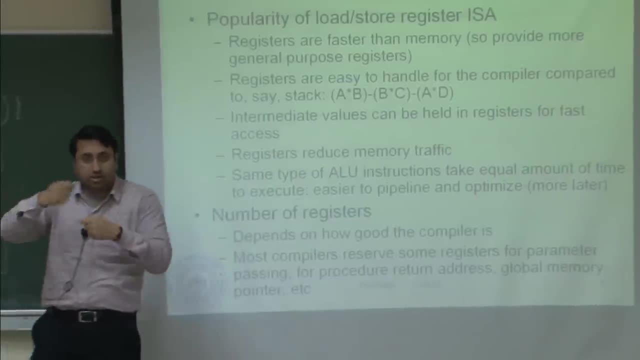 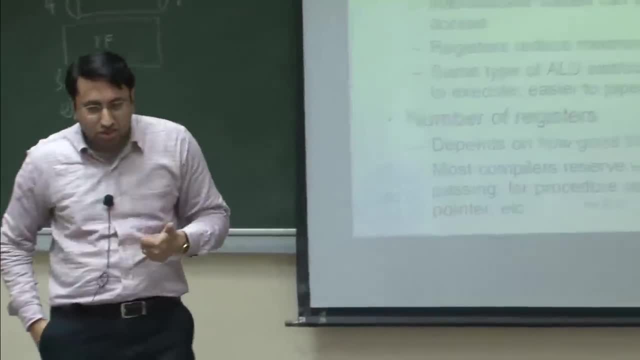 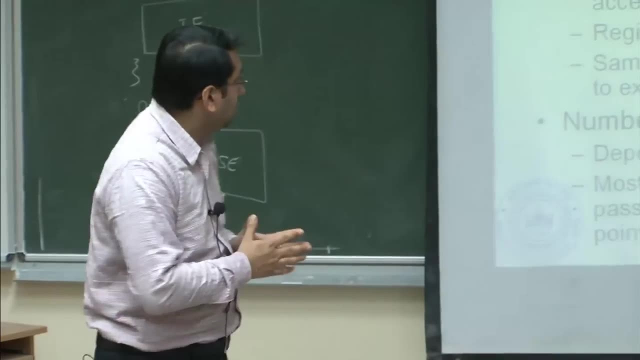 so and the simple there is. a thumb rule for compiler designers is that do not give too many options to a compiler designer, because a compiler will get confused about which one to pick. okay, So here it is easy. everything is same: all ALU instructions will take equal amount of. 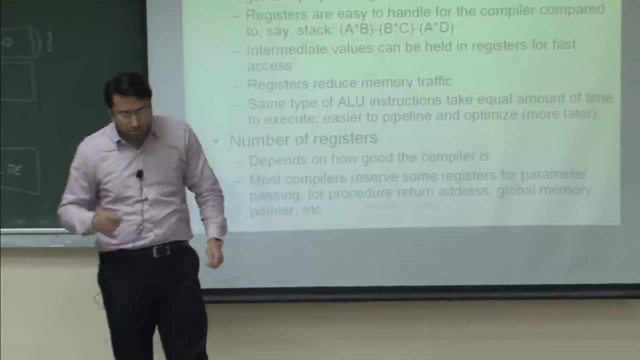 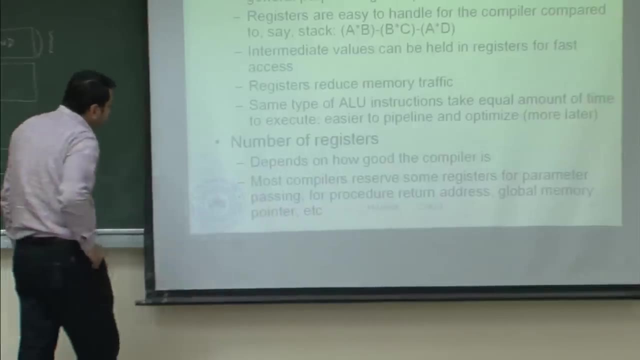 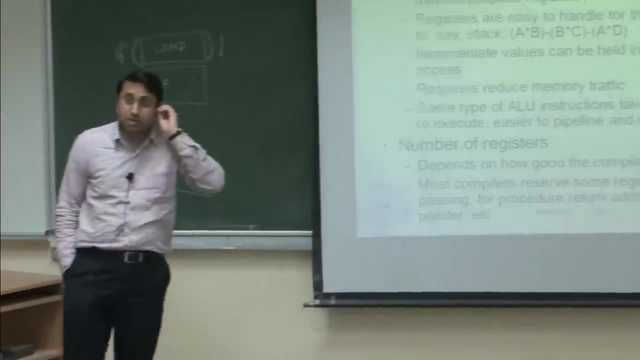 time, so the compiler does not have to debate about: oh, I can do this particular operation in two ways. which one to pick? well, you pick any one, it is the same right, it is the same time. So in this architecture, one important thing to to figure out is how many registers to 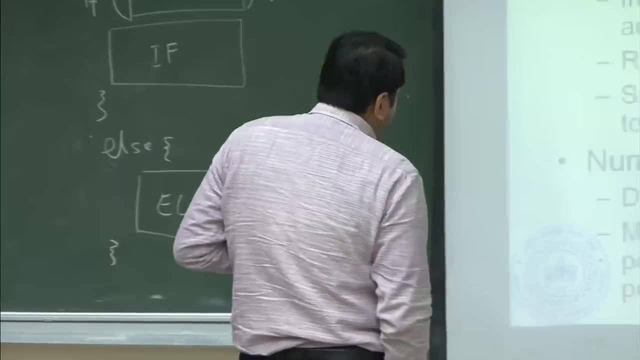 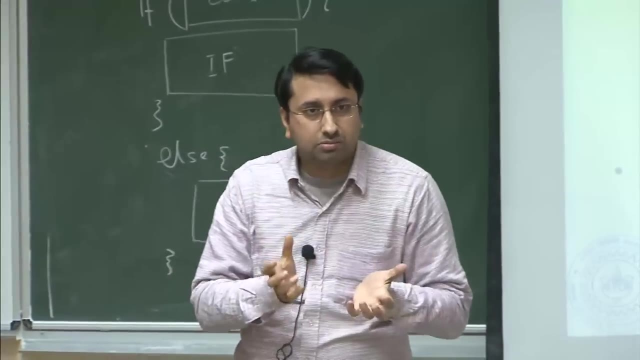 use in an architecture and it depends very much on how good the compiler is. so a smart compiler will probably be happy with a small number of registers because it can allocate the registers in a smart way, whereas a lousy compiler will keep on complaining. you give. 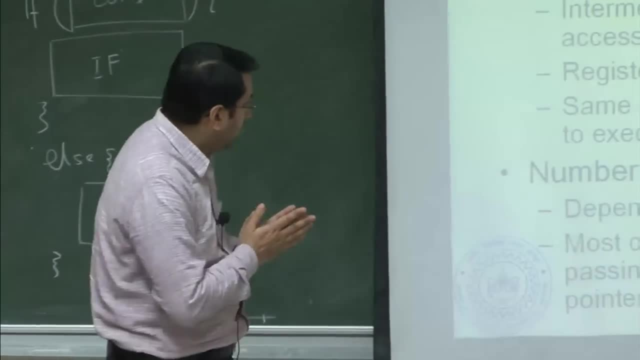 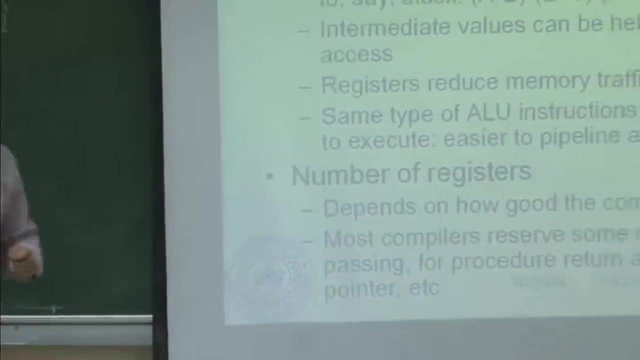 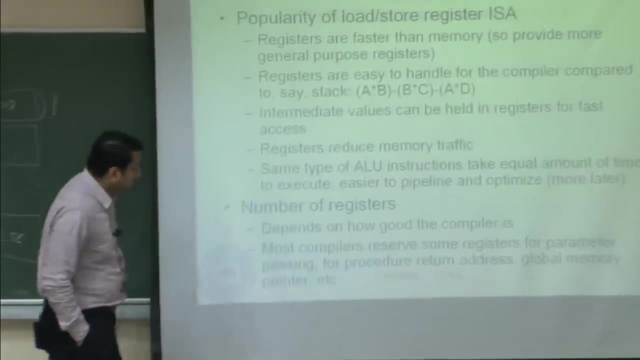 it 100 registers will say, oh, I need more. so it is a very tightly coupled thing where you sit down with the compiler designer team and decide how many, how many registers are actually needed. Most compilers reserve some registers for parameter passing to functions for procedure. 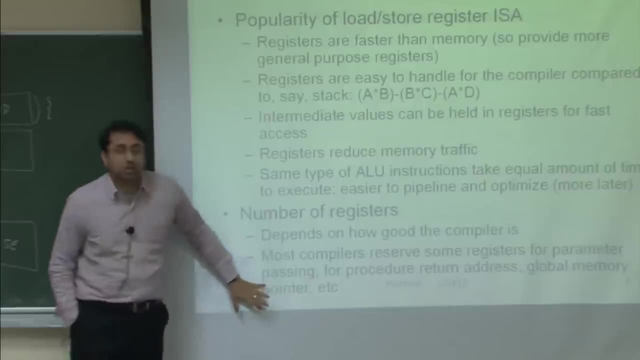 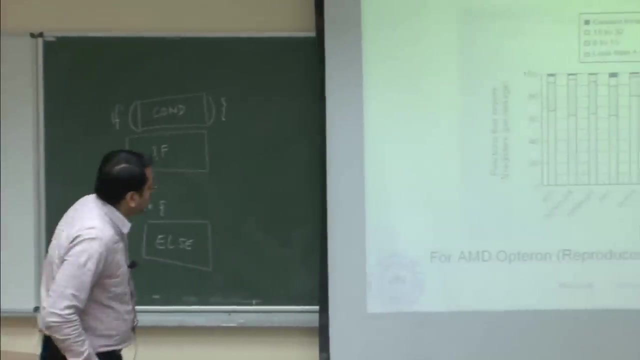 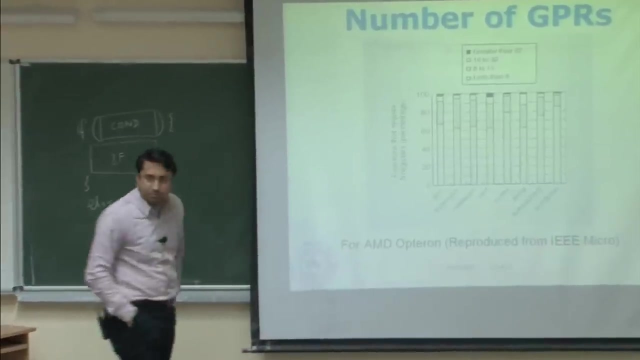 return address, global memory pointer, etcetera. so we will elaborate on this when we talk about MIPS instruction set architecture. okay, So here is some old data- very old actually- dates back to 2004-5 time frame, when AMD Opteron. 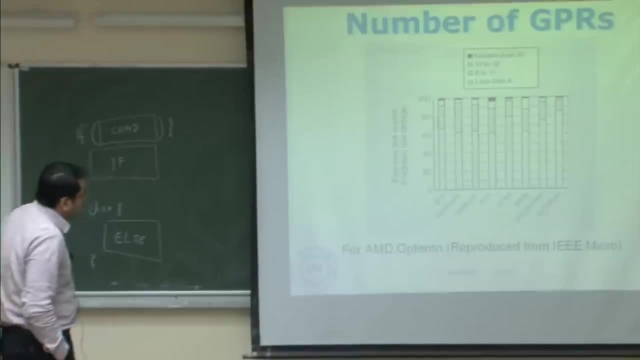 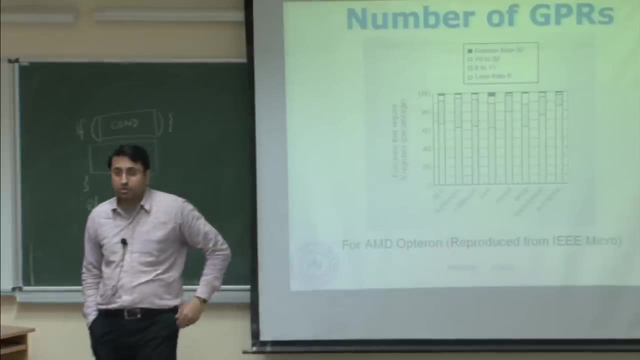 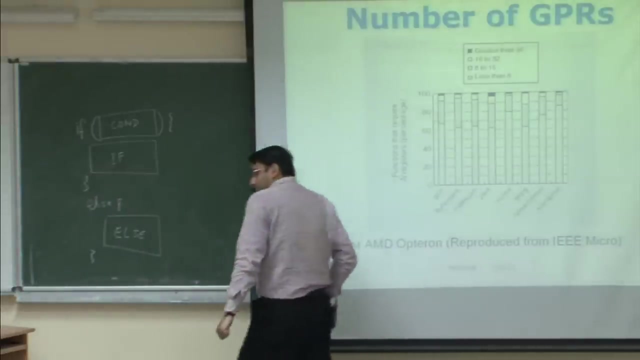 was coming out. So AMD Opteron Made a made a change to their number of registers compared to their previous Athlon plus okay, So they have to figure out how much to increase. so here, what you can see is. so here I have. 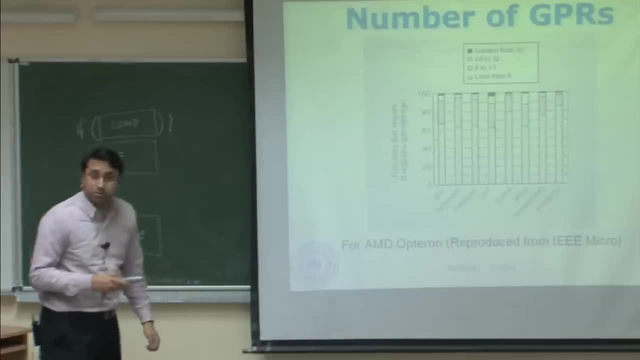 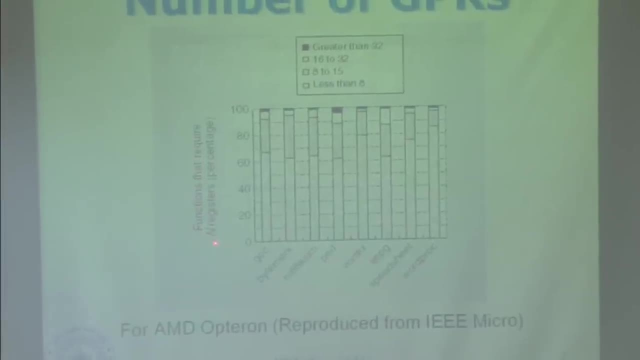 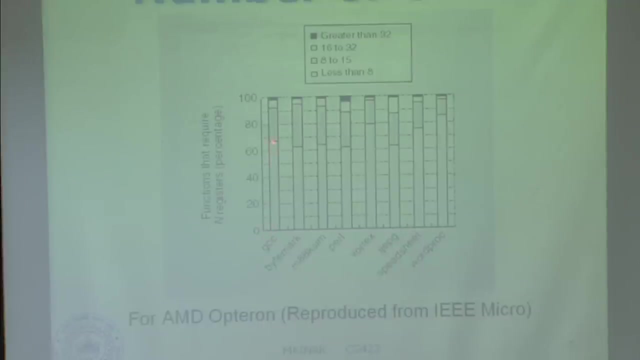 several benchmark applications. these are from old spec benchmark source and y axis shows functions that require n registers. Okay, so percentage of that, All right. so, for example, in GCC, if you look at this portion of this bar, it says that: 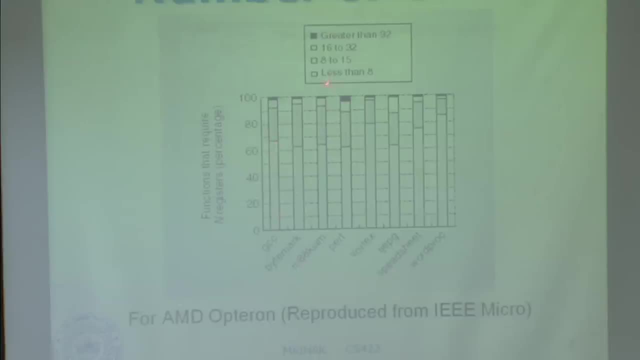 about 70% of functions are happy with less than 8 registers. that's what it is, all right. So you can see that you seldom require more than 32 registers- very few actually, okay, Right. And 16 to 32 is also very small. 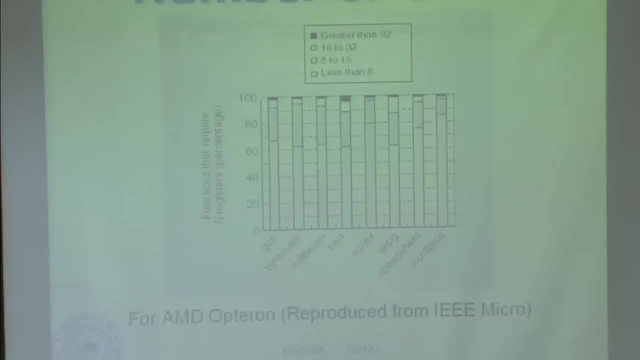 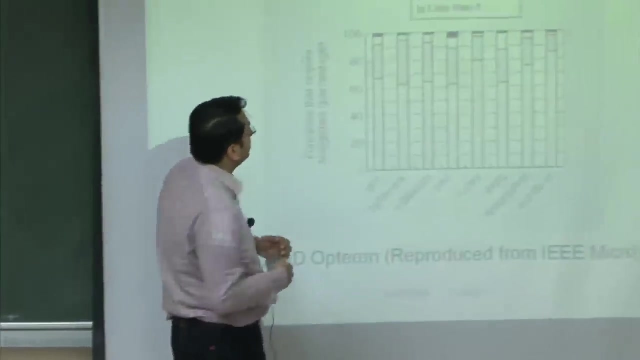 So this is the thing here. this is the kind of data that you normally require to decide how many registers to support in a machine. So essentially, what they did was that they simulated a processor with different number of registers and they ran these applications and they generated this data. 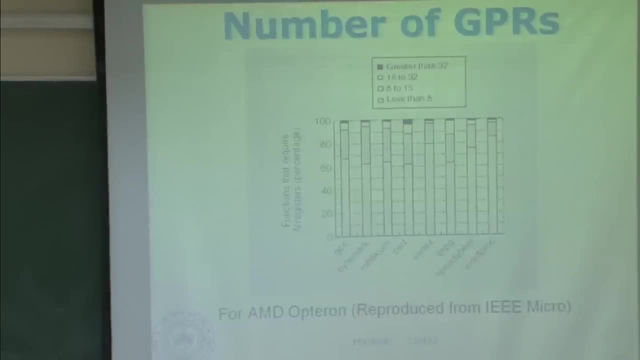 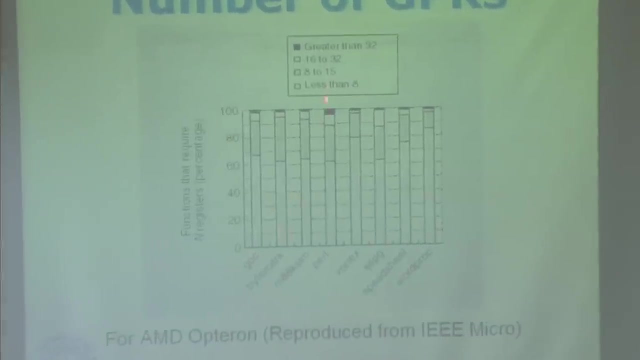 So now it becomes very clear what you should do. you can do a cost-benefit analysis now based on this particular result, right? So so in most cases, I would be- I would pretty much happy to have 15 registers, right? 15? 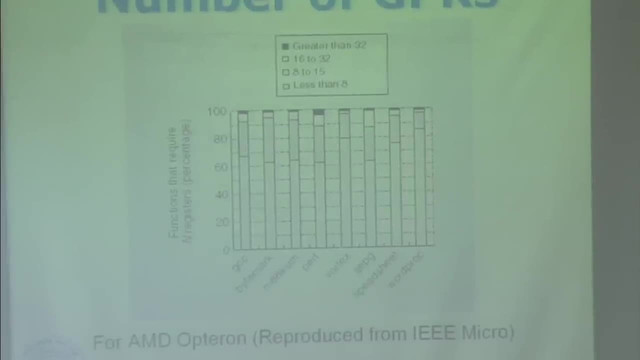 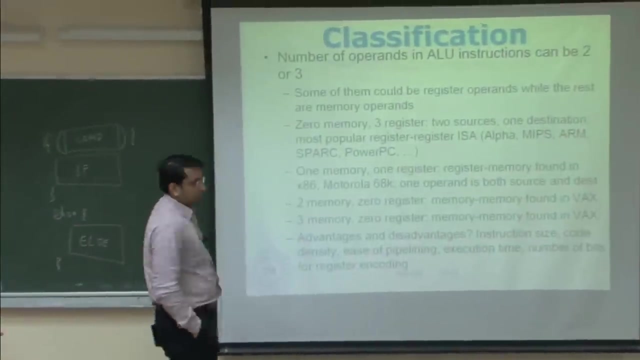 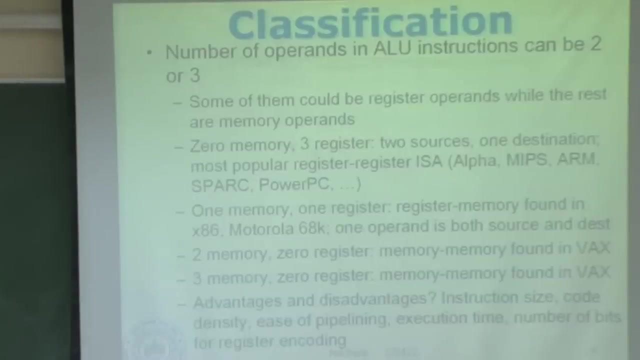 registers have very good coverage. So, continuing with the classification number of operands in the ALU instructions, that is also important. it can be 2 or 3. So some of them could be register operands, for the rest are memory operands. So it is not just about your register register architecture, register memory architecture. 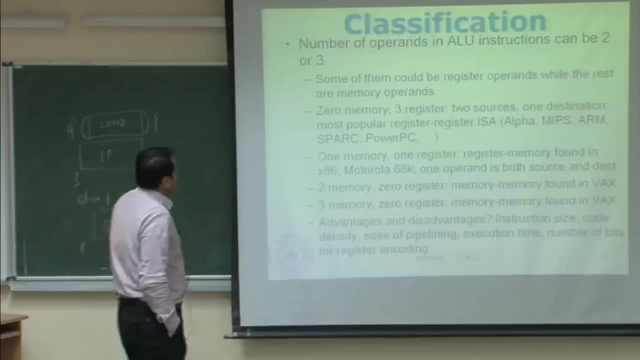 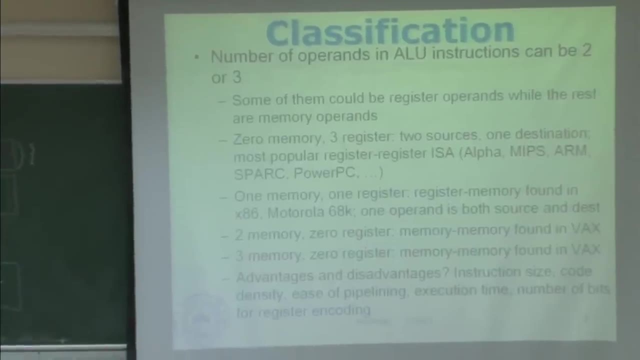 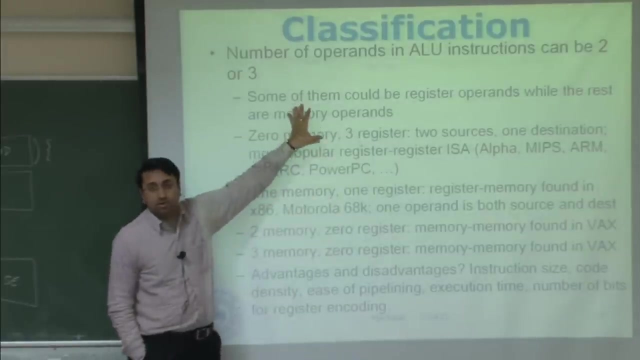 is also included here, So so if you have 0 memory operands, So in that case you would be having 2 sources and 1 destination. this is the most popular register register ISA. So here I am again classifying your ISA based on number of ALU operands and the types of 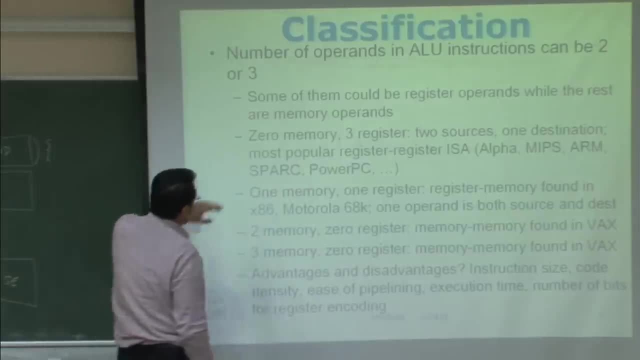 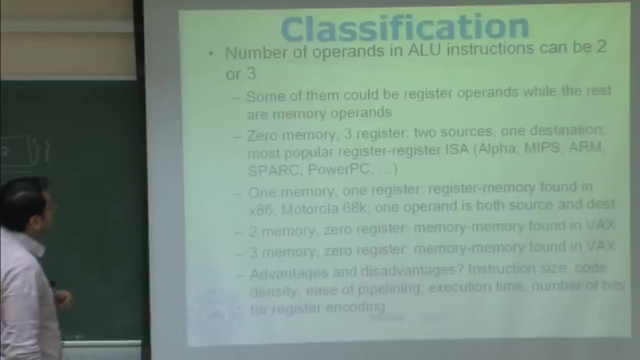 them all right? The first classification is that you have 0 memory operands, 3 register operands, out of which 2 are source, 1 is destination. So these are most popular register register ISA found in alpha MIPS, ARM, SPARC PowerPC. 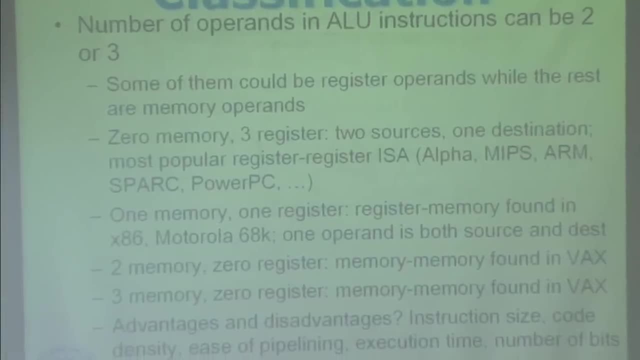 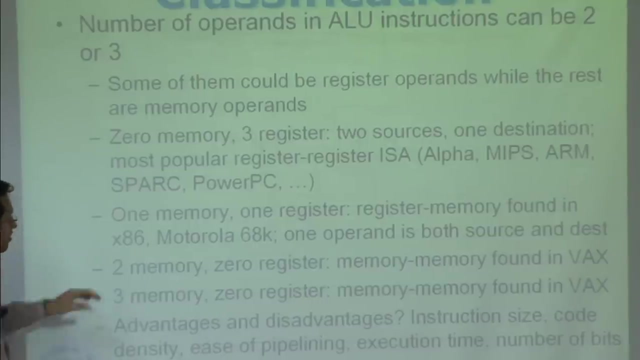 So you might be surprised, So you might be surprised, So you might be surprised to see that x86 is not there in this list, right? So, because it is actually not a register register. ISA 1 memory, 1 register register. 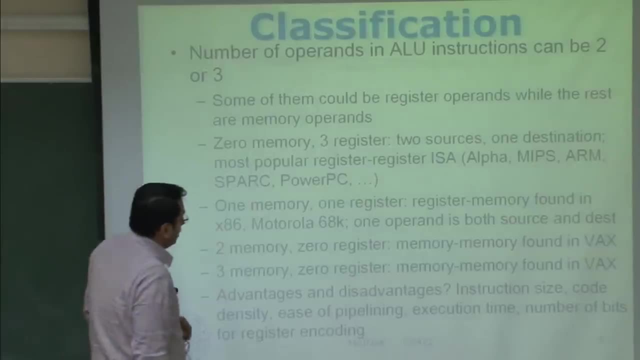 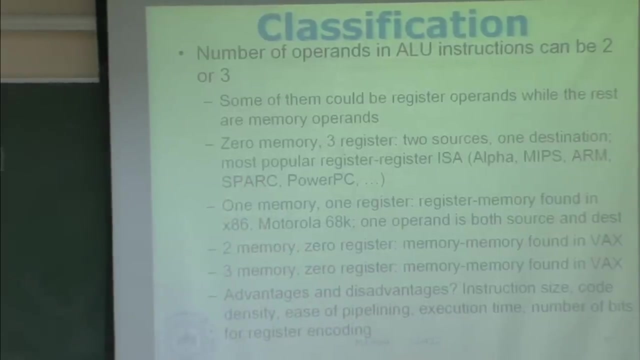 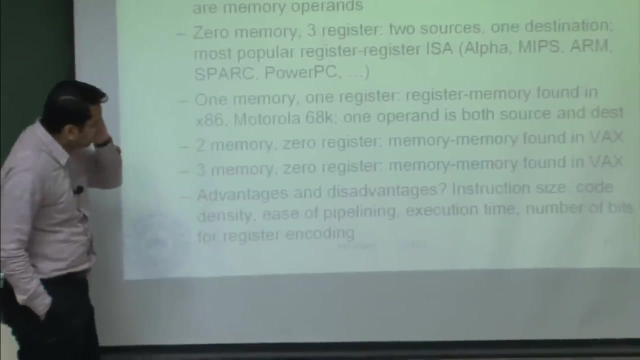 memory found in x86, Motorola 68K and 1 of these 2 operands is both source and destination right, So it is a shared source destination 2 memory 0 register. these are memory memory operands found in VAX old machine. 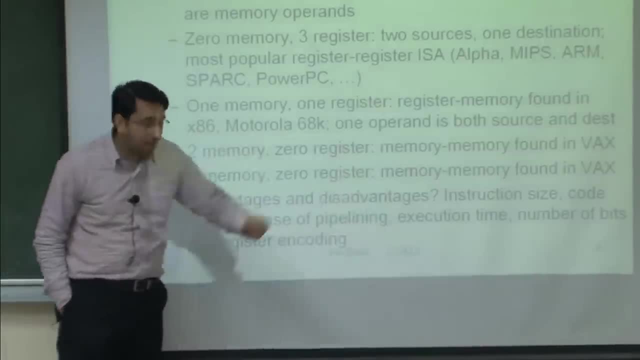 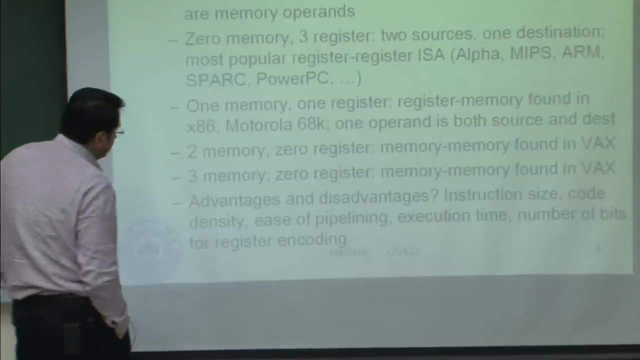 3 memory, 0 register memory memory found in VAX. that is again old Advantages and disadvantages, so it so. this has implication on your instruction: size, code density, ISA pipelining, execution time, number of bits for register encoding. 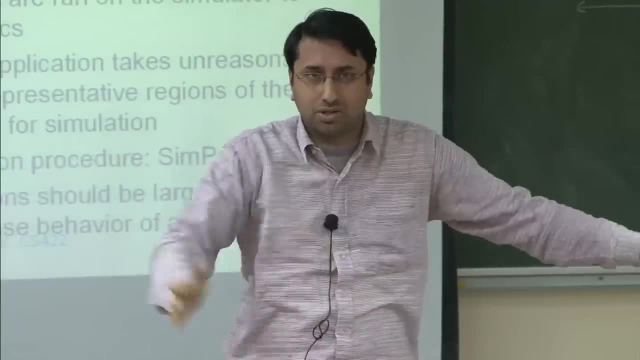 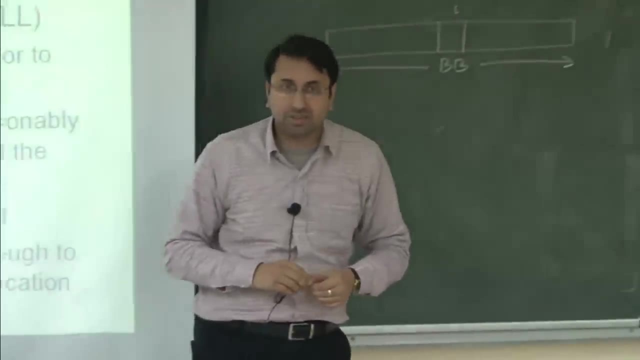 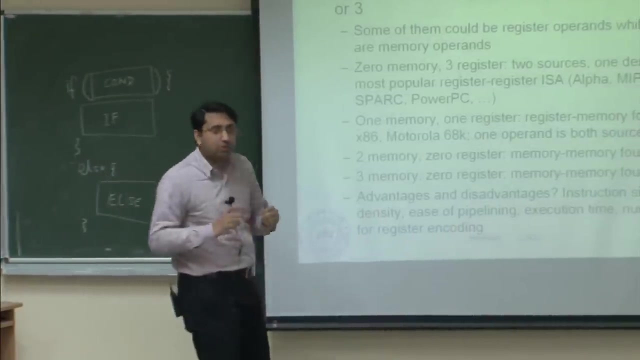 So let us go one by one, some sequence. I have chopped it up into 100 parts, The one that is closest to the center of this, of these vectors, right, Remember that when you are designing an instruction, If you have a memory operand in the instruction, there has to be way to encode the address. 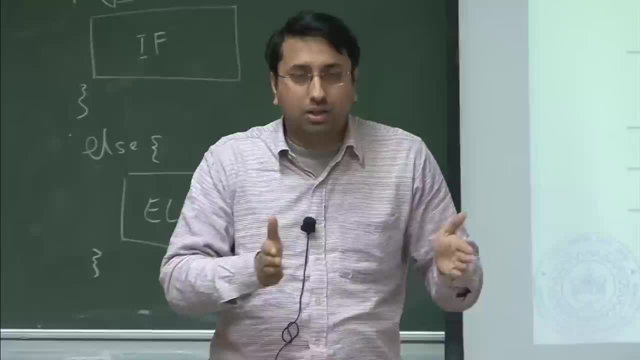 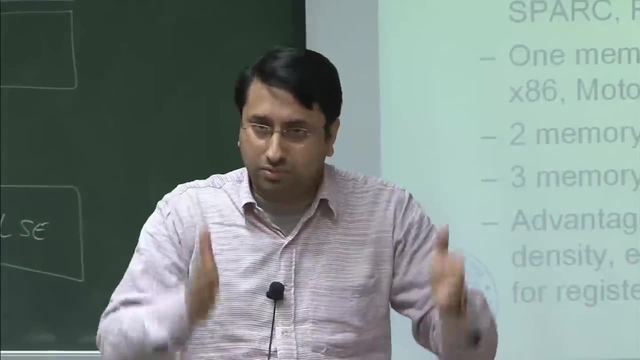 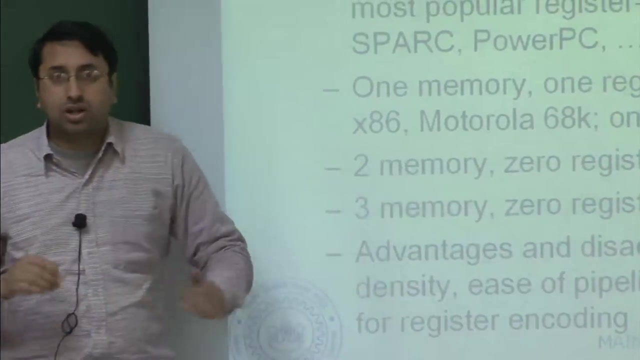 of the memory operand right in the instruction. that requires lot of bits. For example, if you have, if you want to address 4 gigabyte of memory, you require 32 bits for that. just for that right. So clearly your instructions that require memory operands will look large. that will. 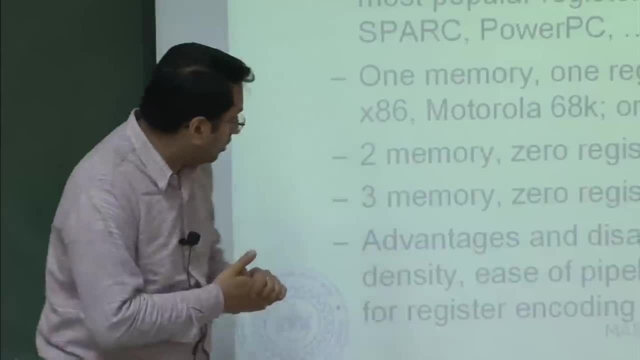 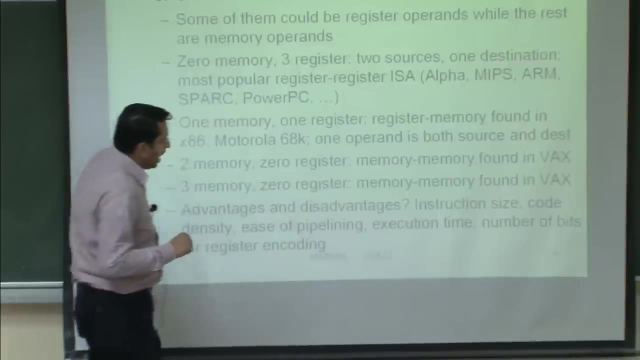 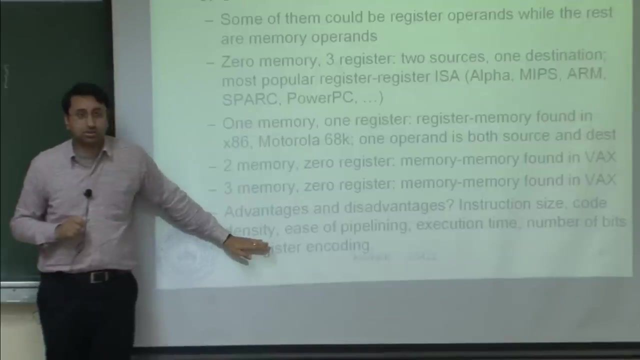 require more space than your register register operands. ok, So so that is. that is what determines your instruction size. size of one instruction: ok, all right, And if you have large instructions to do the same operation, you will have larger code size also. ok, that is obvious, ok. 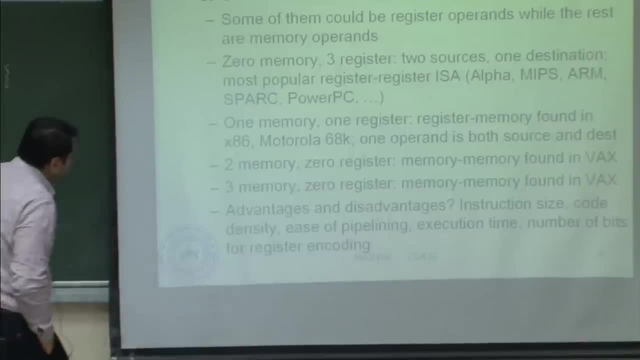 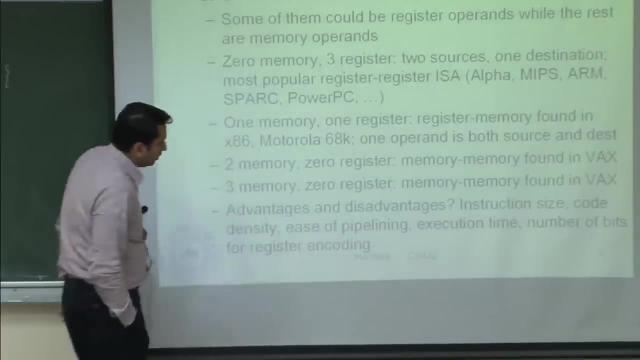 We have the same instruction count and then, if you have memory operands inside your instruction, pipelining becomes difficult. So we will talk about this soon. So, and your that will impact your execution. So that is all, Thank you, Thank you. 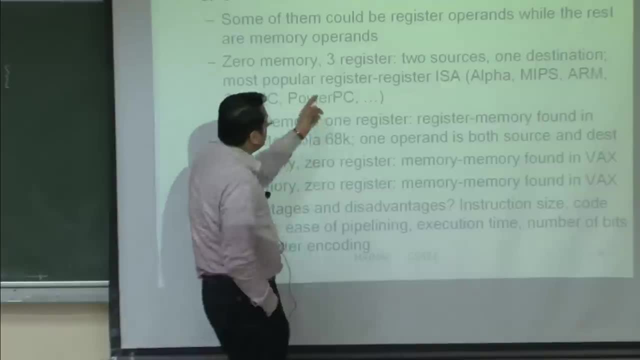 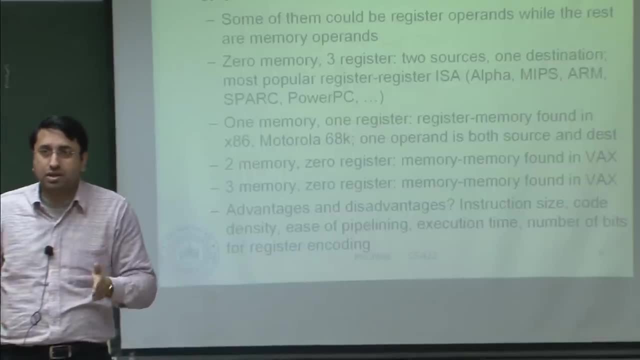 Yes, sir, Ok. So let us take another example. One day I have a custom number. One week ago I made a custom number. Now you have a custom amount of 10 thousand and you have the same value. You have the same value. 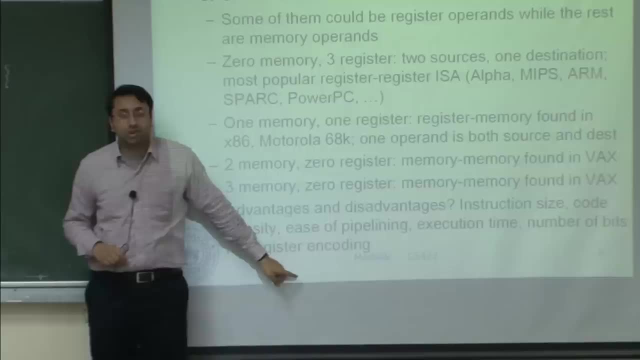 Yes, sir. Ok, So you give me the same value of 10 thousand, so that is basically 10 thousand. That is another problem. Now you have a custom number. I can write down that this is not. So I am not implying that it does not apply to other devices. 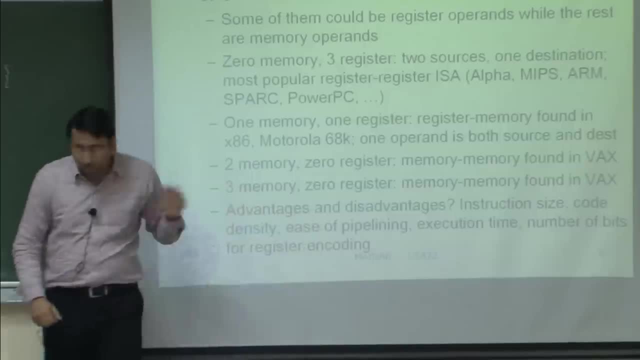 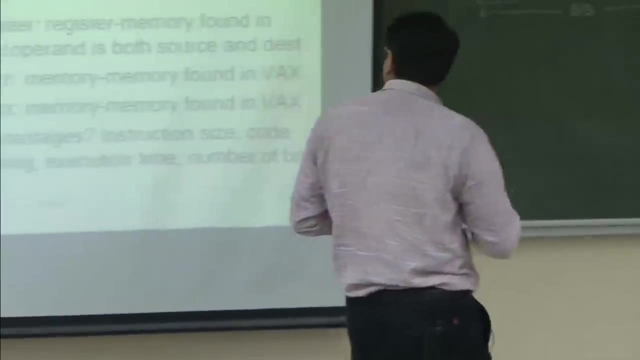 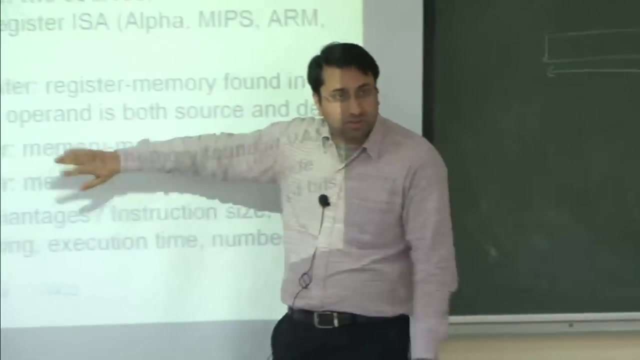 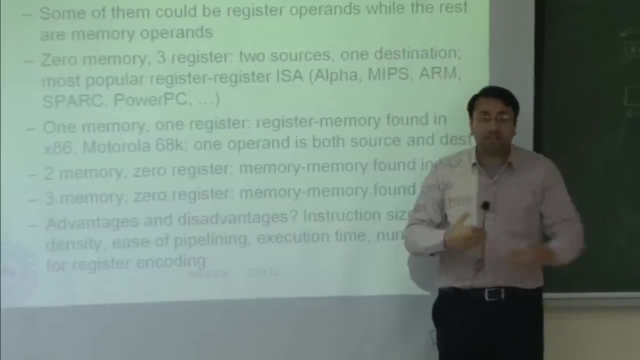 than your memory addresses. So we will continue from here. yes, exactly. So register memory ISA will require less number of instructions because it would actually be encapsulating an ALU operation and the store operation, or a load operation and an ALU operation.